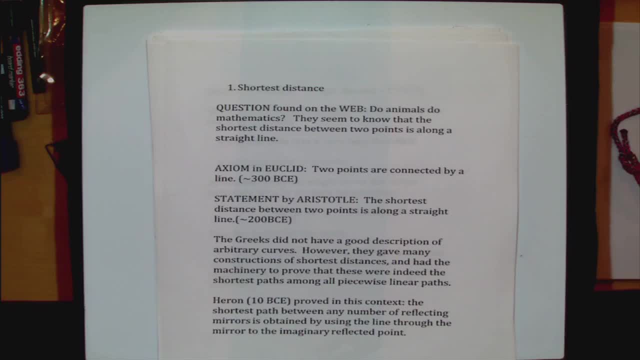 stories and so forth, and I found all sorts of stuff on the web. Let me tell you, don't trust Wikipedia. The university websites are far more reliable, Anyway, but I found some somewhere on the web and I'll never. I couldn't find it again, so I couldn't give you the 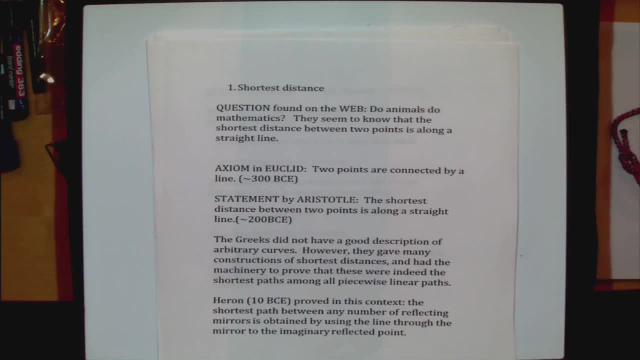 reference. The question found on the web is: do animals do mathematics? They seem to know the shortest distance between two points is along a straight line. So that's the first example that we all know of a minimization problem. Okay, And now if you look in Greek. 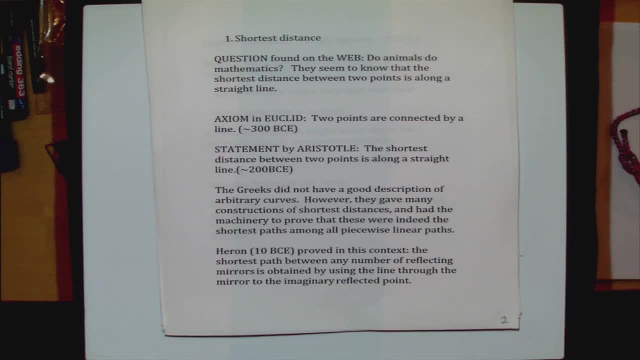 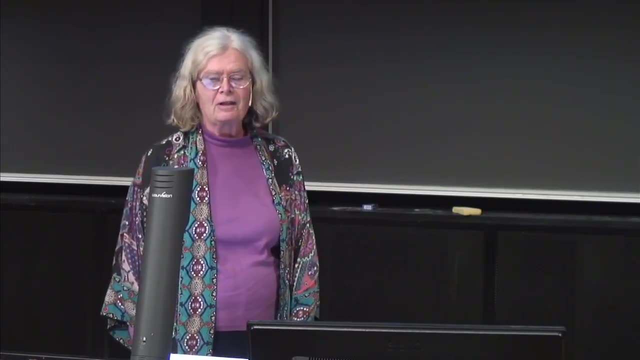 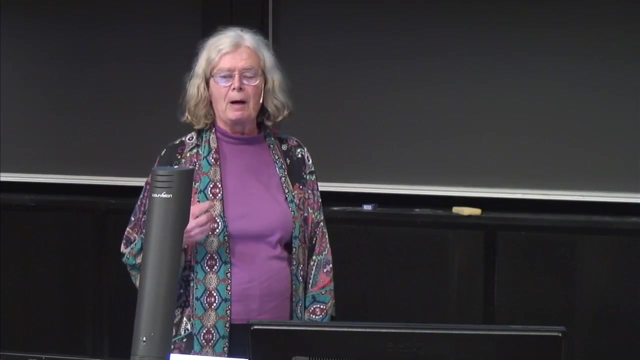 mathematics they actually don't talk about. at least Euclid doesn't talk about shortest distances, He taught they actually make a lot of constructions that are shortest distances, For example, the fact that you can drop, that you can drop a perpendicular from a point to a plane, or, in fact, the most. 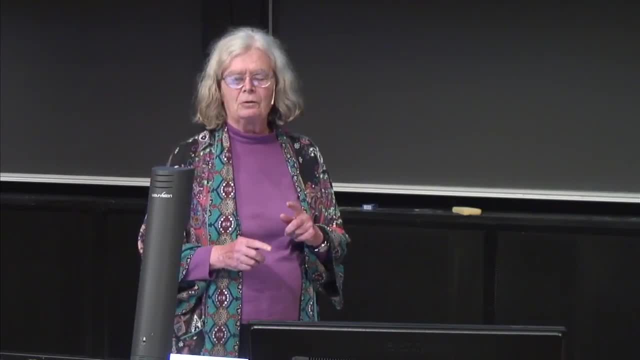 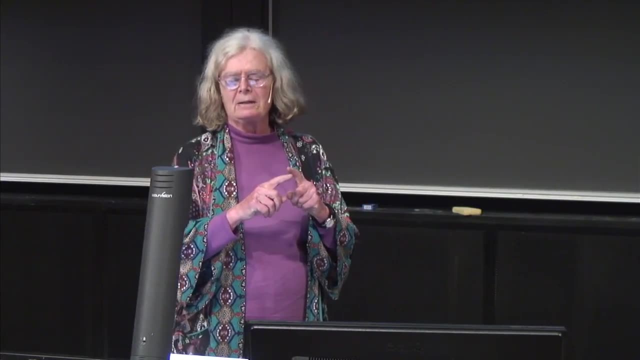 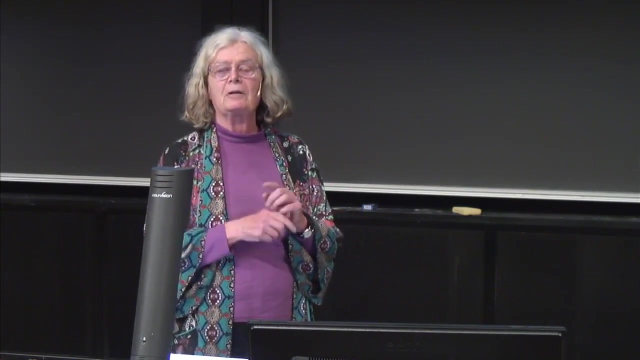 complicated one is that you can draw a line between: if you have two lines in space, skew lines in space that don't intersect, they actually have a line perpendicular to both of them, which, and that, of course, does realize the 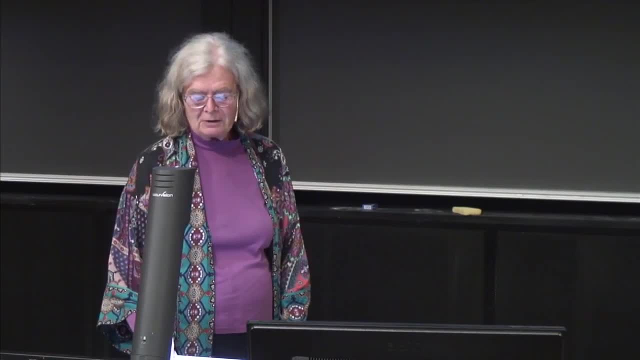 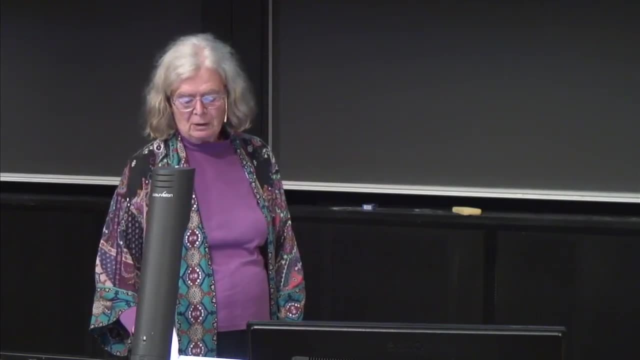 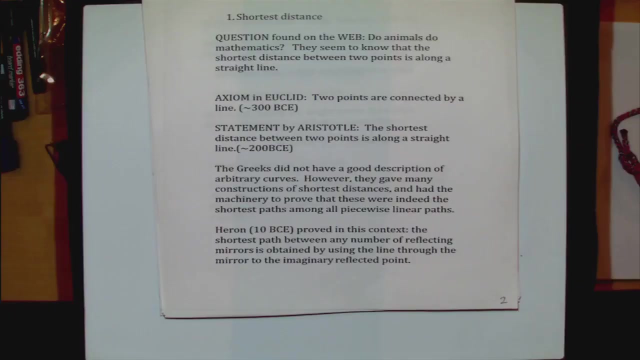 shortest distance. But it is certainly a statement by Aristotle that the shortest distance between two points is along a straight line. So that's the first quote. The Greeks didn't have a good description of arbitrary curves. I mean, this is what mathematics is for, is it tells? 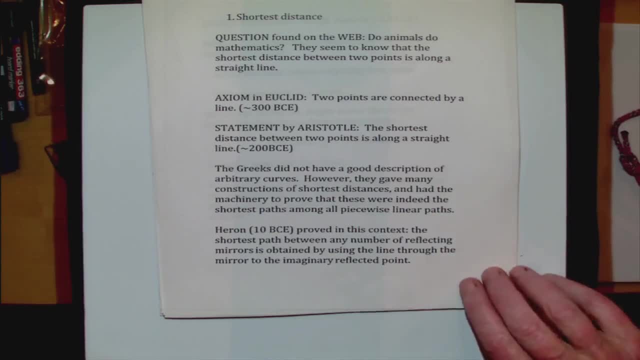 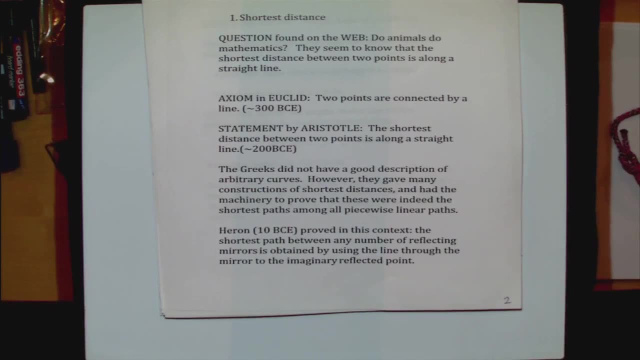 you how to describe things and they didn't do it. But they gave lots of examples and they gave lots of these constructions and they did have the machinery to prove that these were the shortest. the constructions they made were indeed the shortest paths among. 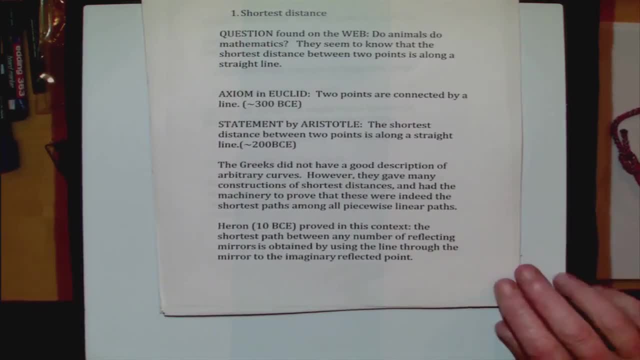 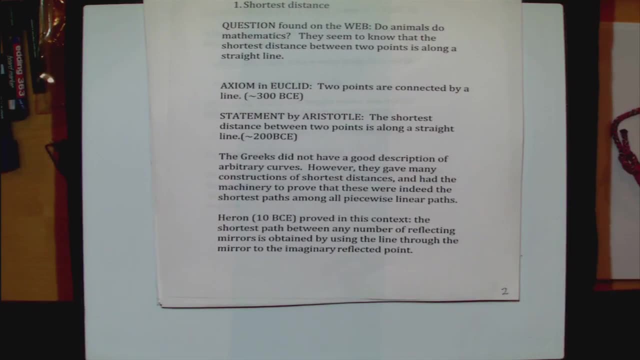 all piecewise linear paths. that is broken straight lines. And it's interesting- because we'll come back to that- that in 10 BCE, Heron proved that the shortest path between two points with any number of reflecting meters, Reflecting mirrors, That's typical mathematics, right? You do it for one mirror and then 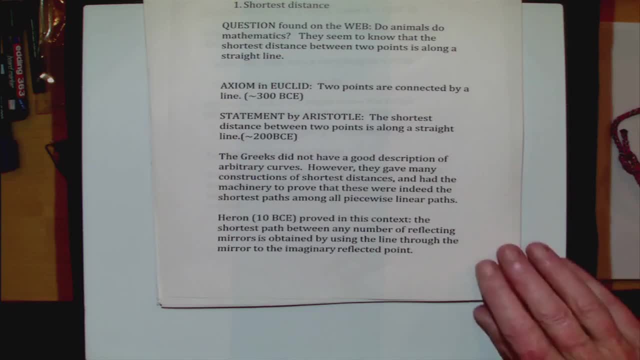 you say, oh yeah, but I can do it for any number, And so any number is gotten by. if you want to find the distance through the mirror, you actually reflect the point through the mirror- We'll come back to this- And you actually draw the straight line. and then 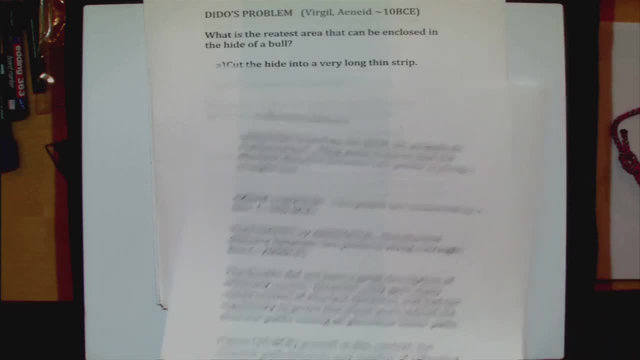 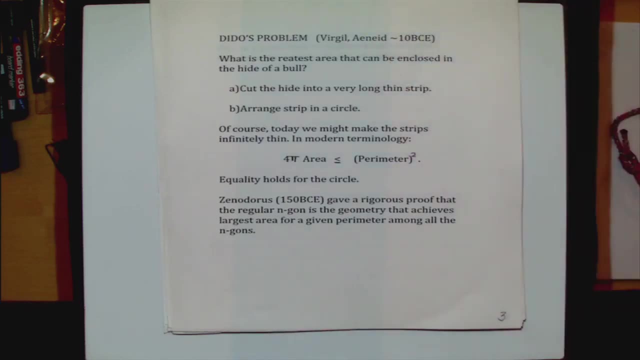 you reflect the line, So that's okay, But so we want to have some women in this talk. So Dino's problem is in from Virgil the Aeneid, which is 10 BCE, And the question is: the question asked is: the story is that? 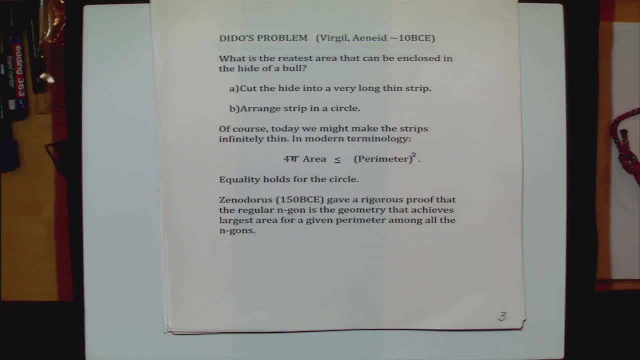 she was a princess in Tyre and she had some difficulties with her brother And so she sailed all that way and she just A todospanos, because if I got crosses for my brother I would see them again. So it's off looking to found a new city and she arrived on the coast of sorry Carthage right and 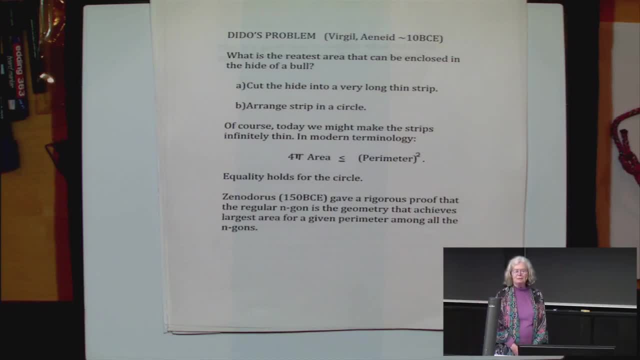 she met the barbarians there and asked for some land. and she asked for the amount of land that she could you can enclose in a hide of a bull and the. so they said, oh sure, this silly woman will give her what she wants, and so she. the first part is clever, but the second part is. 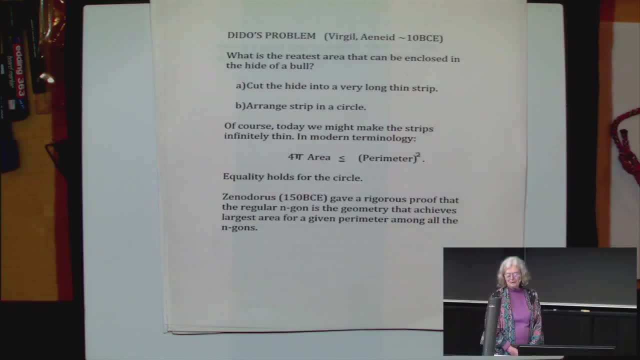 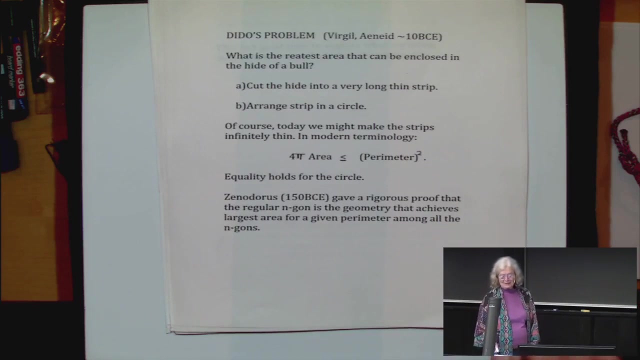 mathematics. she cut the hide into very long, thin strips and of course nowadays we would say as mathematicians we can cut them into infinitely thin strips and we get an infinitely long line. but the Greeks? the Greeks weren't that ambitious. and then she arranged this strip in a 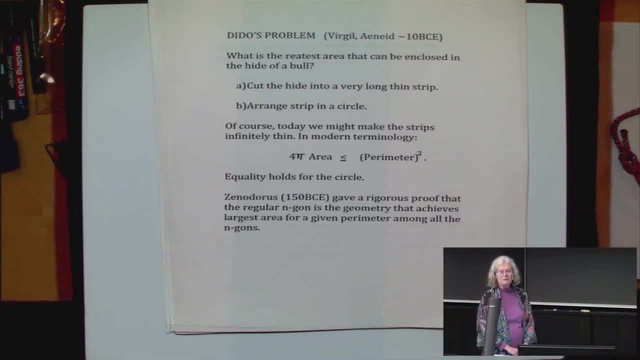 circle and today, this fact that the circle, if you have a length of string and you want to enclose the biggest area inside it, you would arrange that in a circle, and that is called the isoparametric inequality, and it's of course been extended to many other different kinds of geometry. 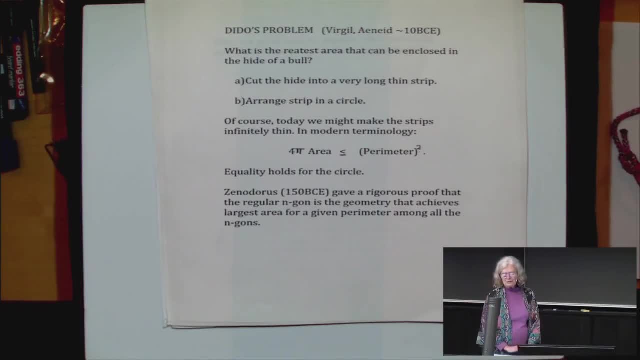 and it's interesting because, again, since the Greeks didn't have the description of curves, they couldn't actually prove this. but in 150 BCE, Xenodorus gave a rigorous proof that if you did this with an n-gon, that is- and again that was, they were ambitious- any number of sided thing. 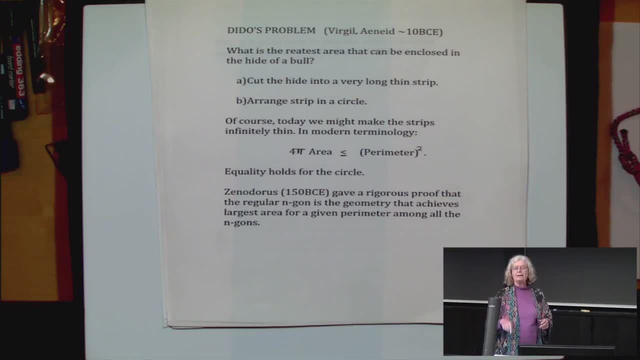 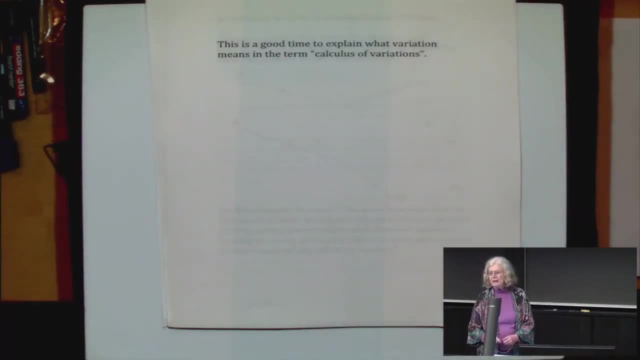 that the solution was the regular n-gon with even more sides. Now, right now, maybe this is the time to explain what variation means in the calculus of variations. So we're, we're going to be dyed out and we have a long strip of bullhide that we've cut and 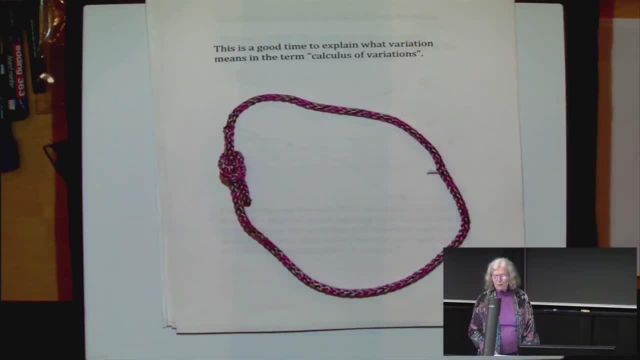 tied it up and we've ranged it down and we want to know how to think that the circle is the answer. Well, if we lay it down and put it a bit longer, We want to know: can we make it shorter? 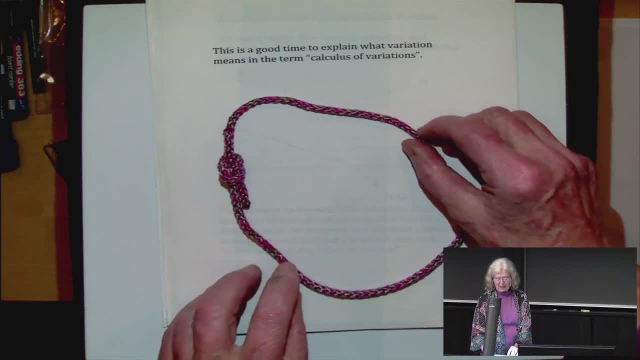 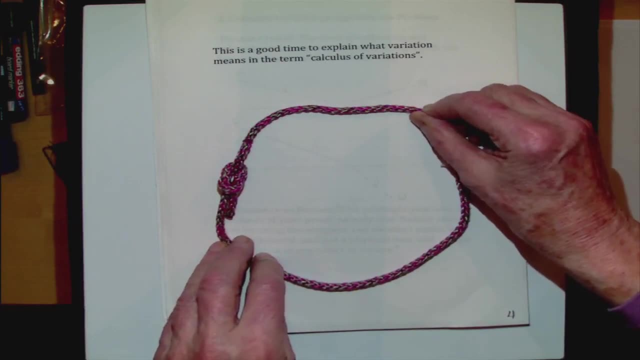 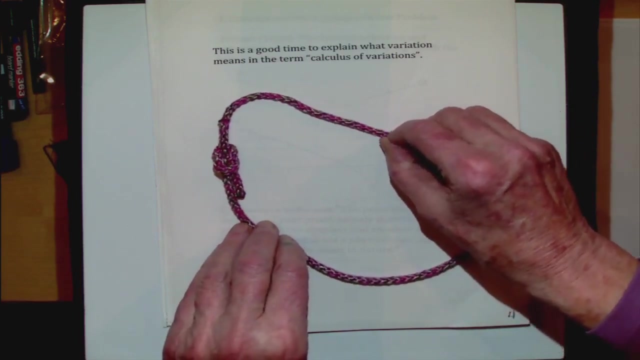 Can we enclose more area? What we do is we actually choose a direction and we move the string in that direction and we calculate the difference in the area. Now, this motion is actually in the And we would actually in modern days. 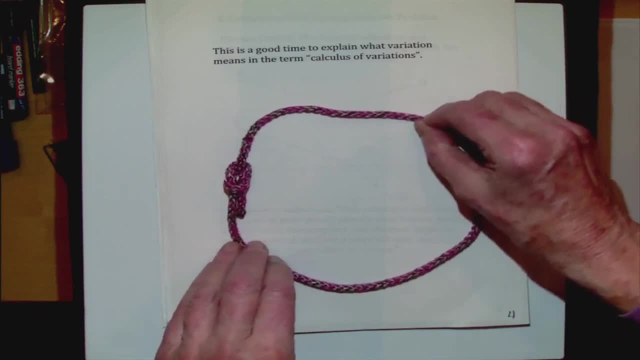 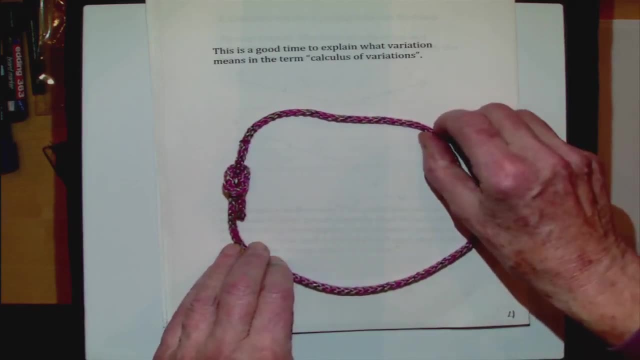 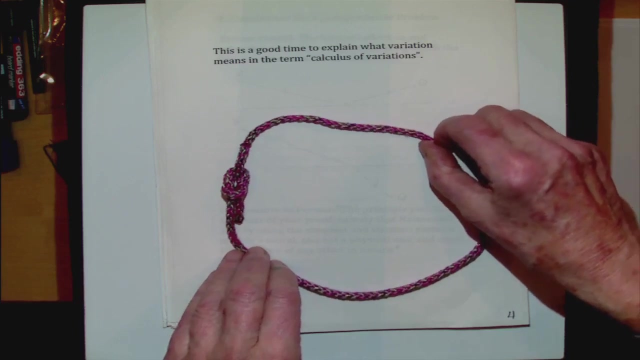 we'd assign a parameter to that motion. People often say time, but that's confusing, because time it isn't time, It's an external parameter. And you move the external parameter in this and you see if the area changes, And in fact so you actually. 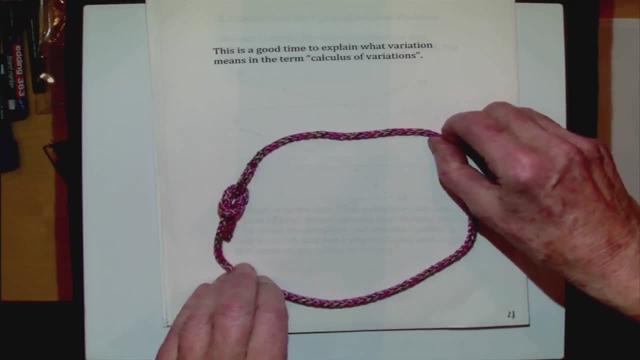 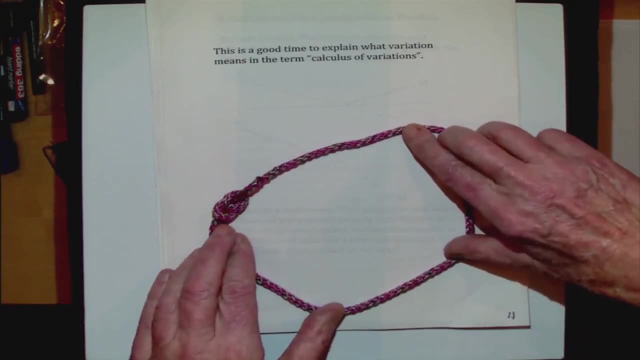 What you do in modern days is you calculate the derivative of the area along that motion. And if the derivative is zero, like for a circle, we know that. We don't know that it's a minimum, but we do know that. We know there's no obvious counter-example. 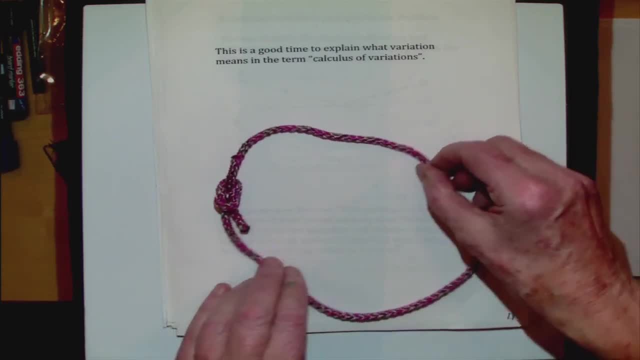 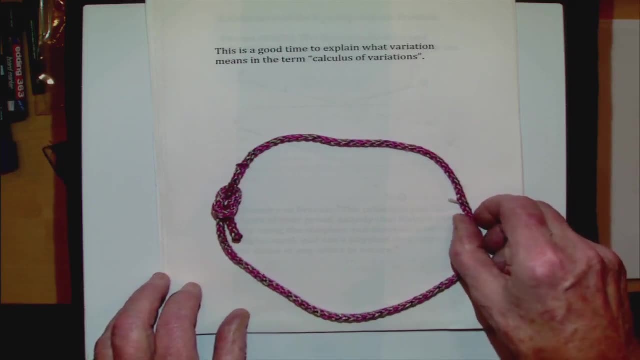 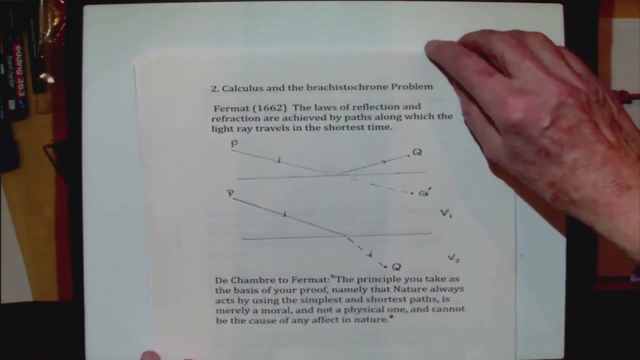 whereas if it's not a minimum, then we know we move it in this direction and it becomes less, And so that's our test for a minimum. Okay, So now we come to, We go back to Zenodorus, and So Firma and 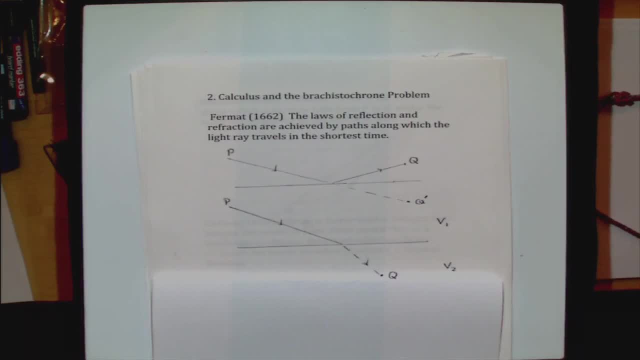 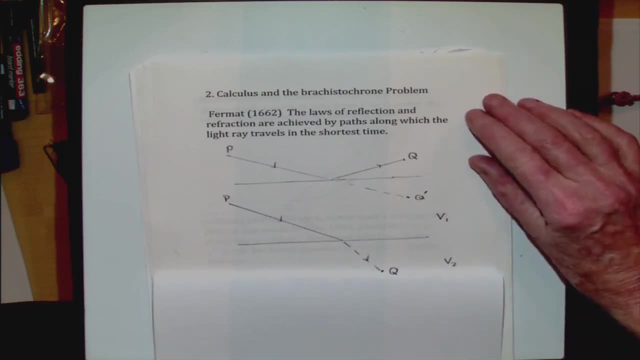 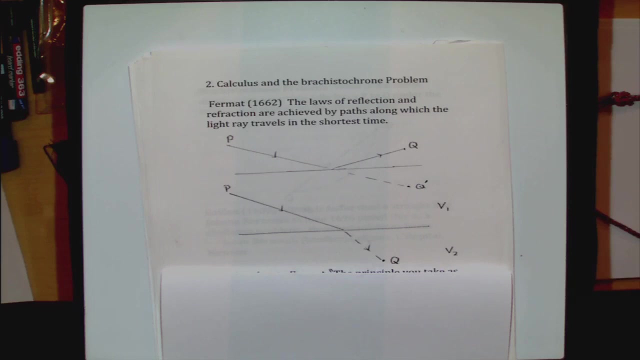 So this is a big skip in time. We're going to have several big skips in time. Firma In 1662 derived the laws of reflection and refraction. It claimed that light travels from P to Q along the path of shortest length. 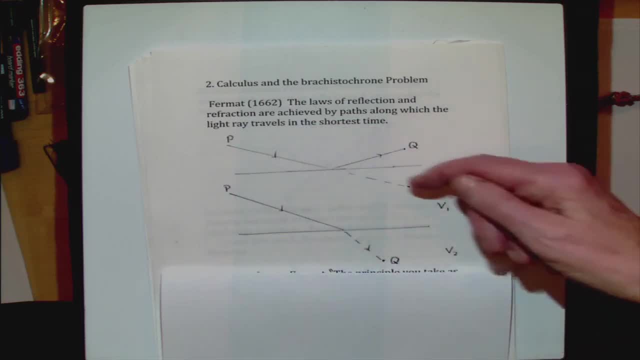 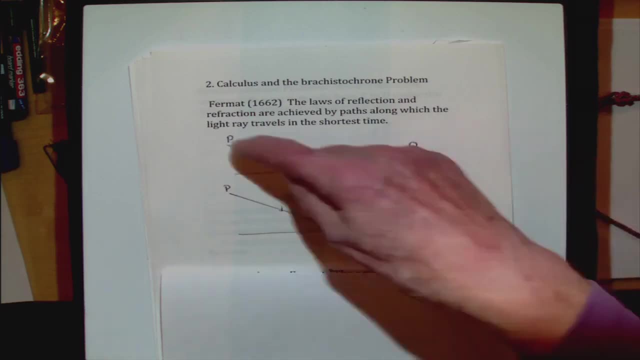 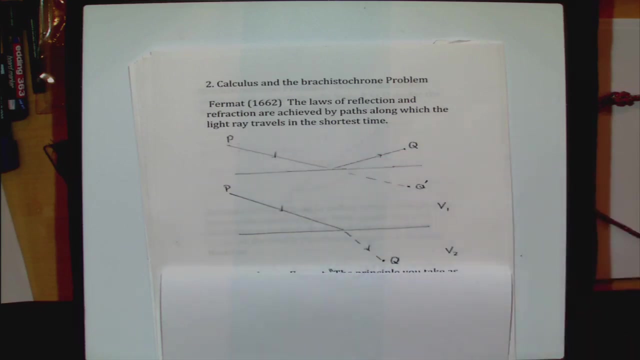 And again, the path, This is, This is, This is Here on again. That is, you want to go from P to Q And, by the way, notice, it's not a minimum, Notice that if you were to draw the straight line, 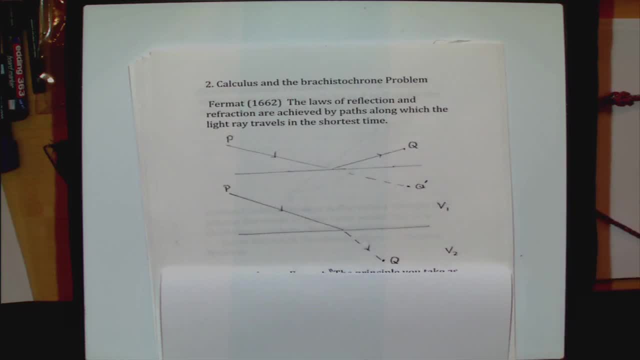 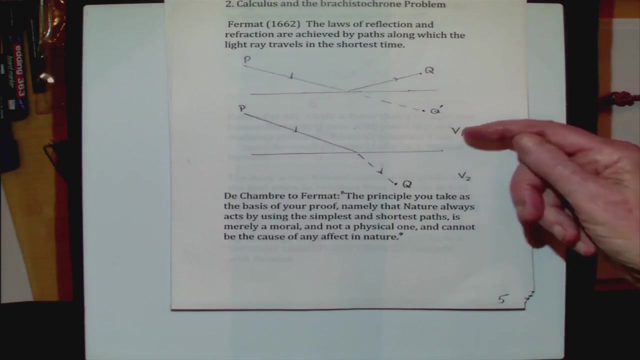 from this P to Q. here it would be less time. So what you do is you reflect Q to Q prime, draw the straight line and then reflect the line, And again the laws of refraction are derived, If you have. 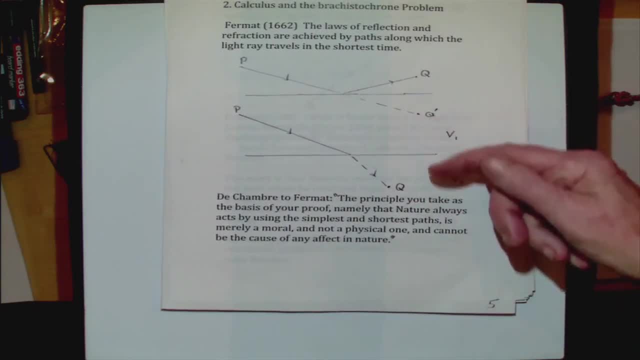 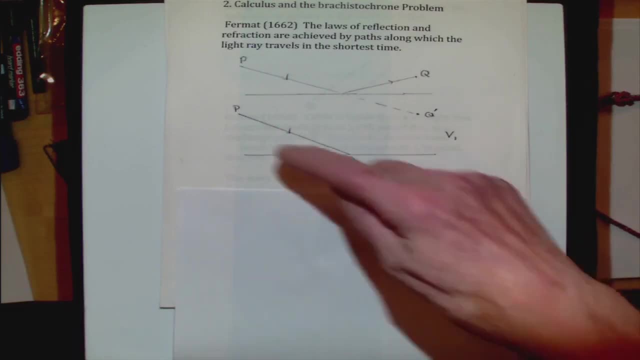 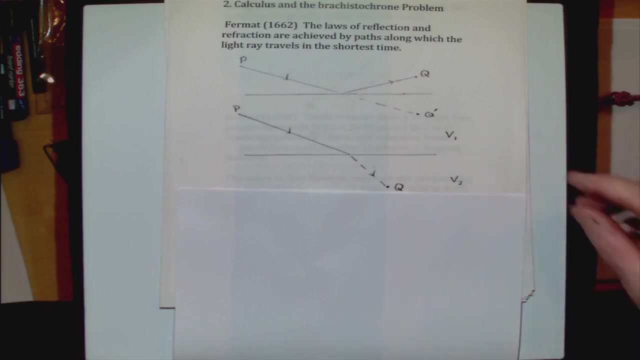 The light travels With a different velocity in this medium from the top medium to the bottom medium, then the path still takes the least time, And so you can think about it a little bit About. I drew this picture on purpose, and you can decide which. 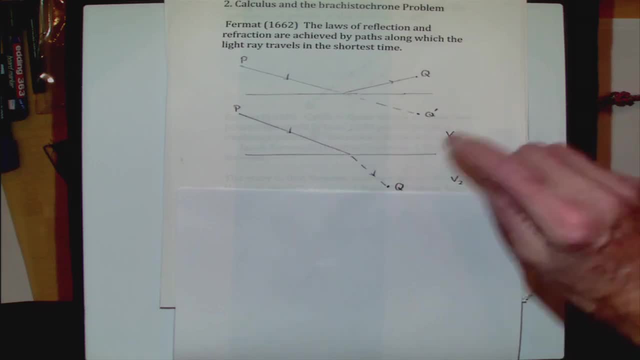 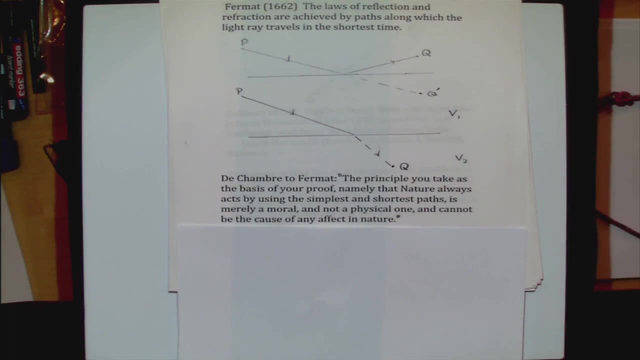 Is the velocity smaller here, larger here or here? From the picture you should be able to tell. But I found it very interesting because, And especially because, The laws of physics are very, very much based on conceptually minimizing things, And in the same year, 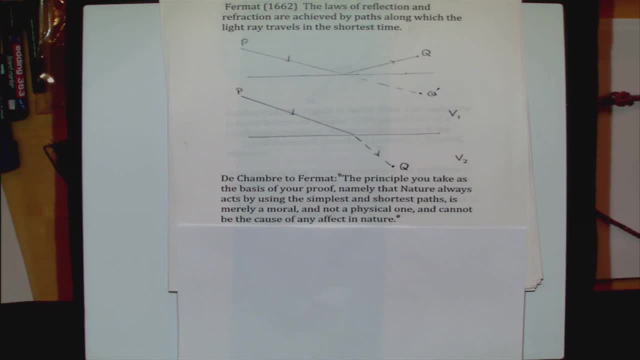 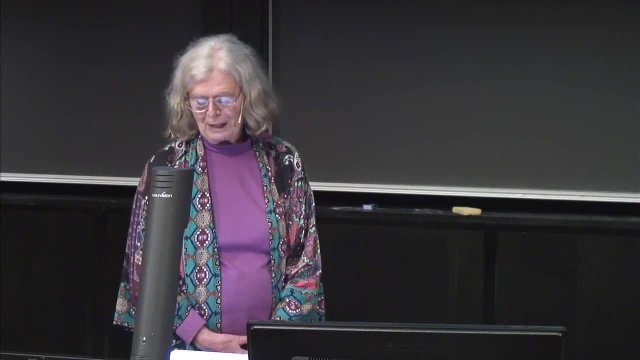 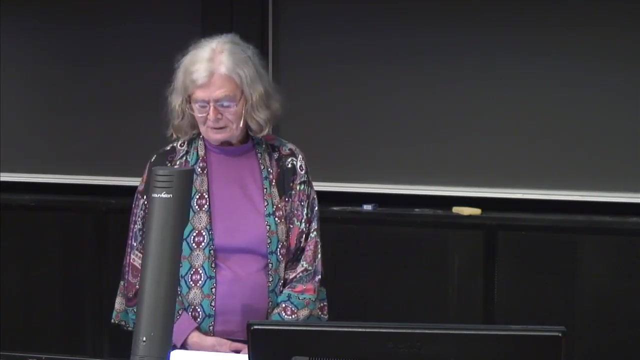 So we skipped a lot of centuries there. but in the same year de Chambre wrote to Fermat that the principle you take as the basis of your proof, namely that nature always acts by using the simplest and shortest path, is merely moral and not physical. 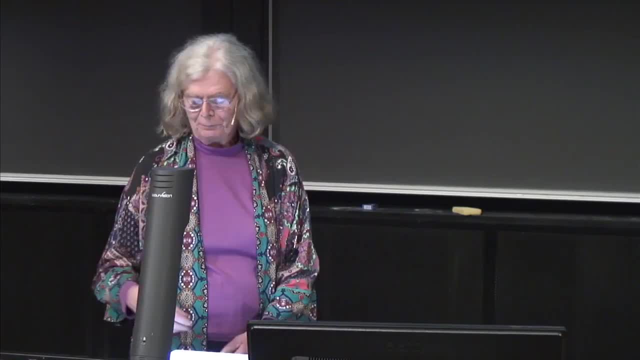 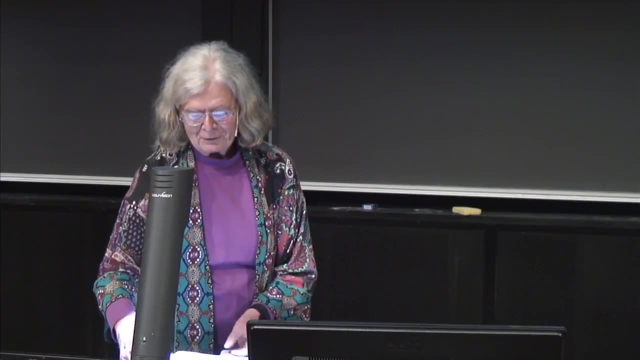 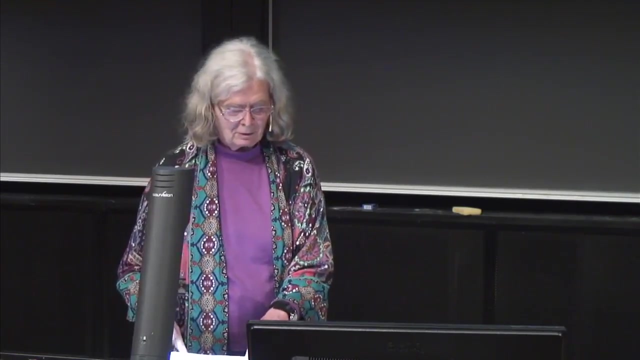 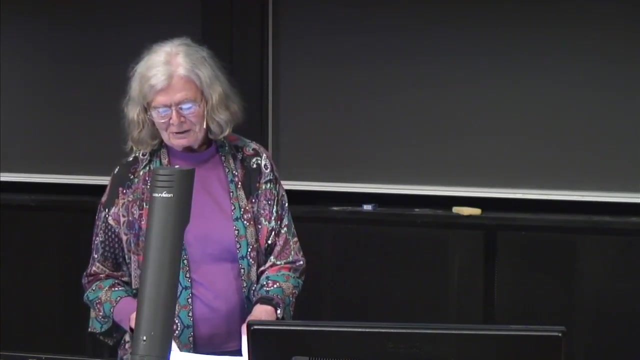 And cannot be the cause of any effect in nature. Well, you can think about that, because, Okay, Now we come to the, you know, Brachysticone problem. Oh, okay, Okay, This is the one- that my thunder has been stolen here. 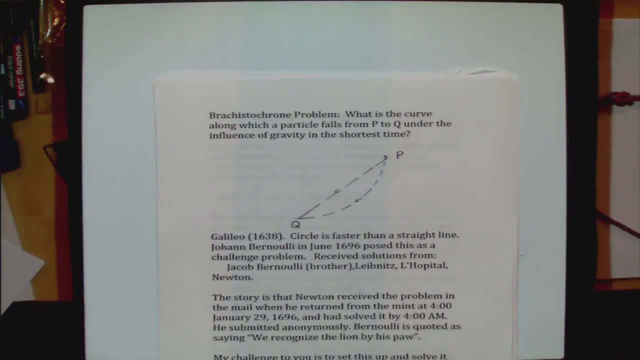 So the question is: is what is the curve along which a particle falls from PDQ under the influence of gravity in the shortest time? And I don't actually know why this question came up, and I never heard before I came to Oslo that it was called the ski jump problem. 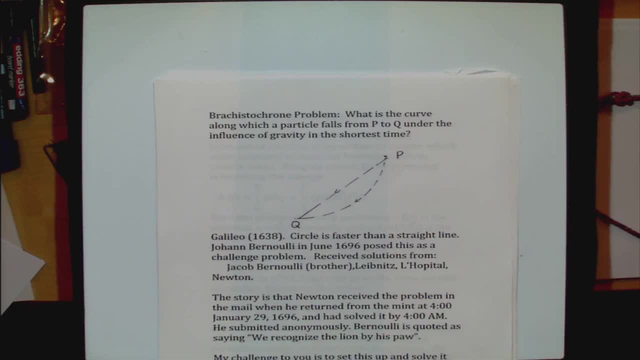 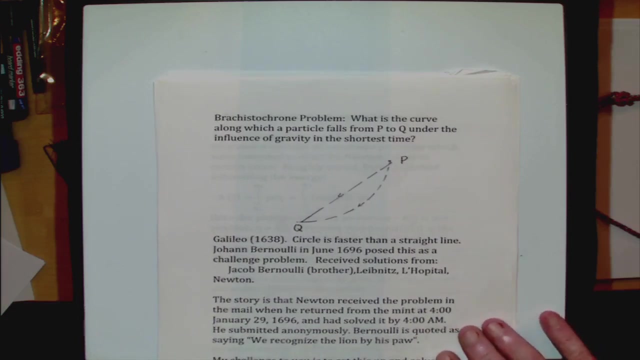 But anyway, what is interesting is is that Galileo was able to compute that a circle was better than a straight line, That is, it was faster, But- And he actually proposed that that was the solution. But So it's good to know that great mathematicians make mistakes. 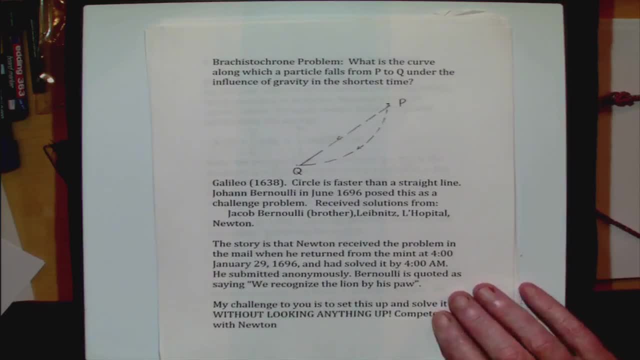 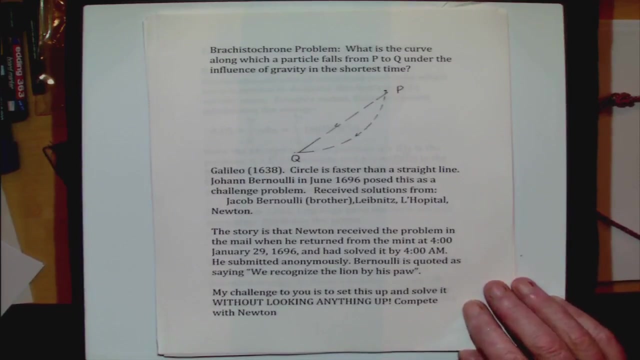 But- And Johann Bernoulli- in June of 1960, now posed this as a challenge problem. I understand Again. I don't know how much you believe when you read this on the web, but it's claimed that he actually knew the solution. 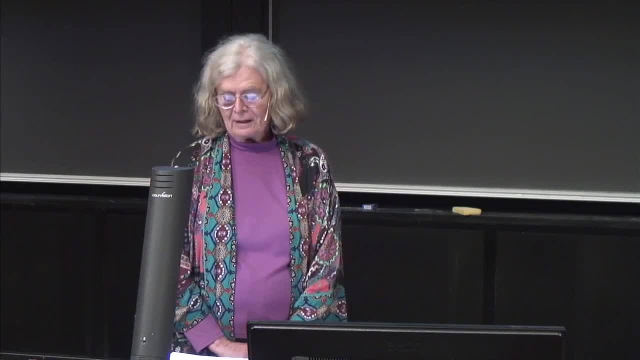 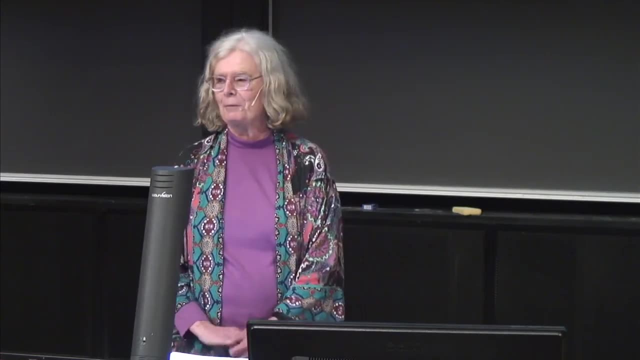 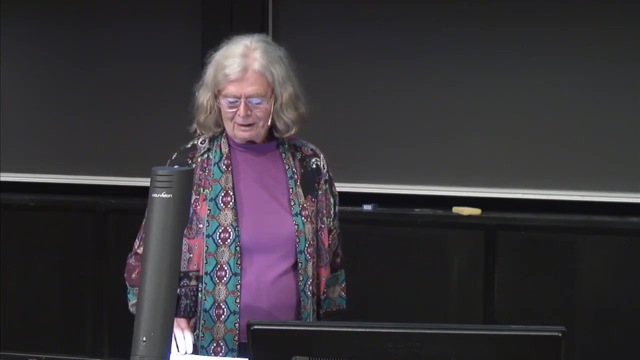 at this point And he- I also listed the familiar people. His brother also submitted the solution and there was a lot of controversy. So mathematics has never been a peaceful subject, And both Leibniz, Lobital and Newton submitted solutions. 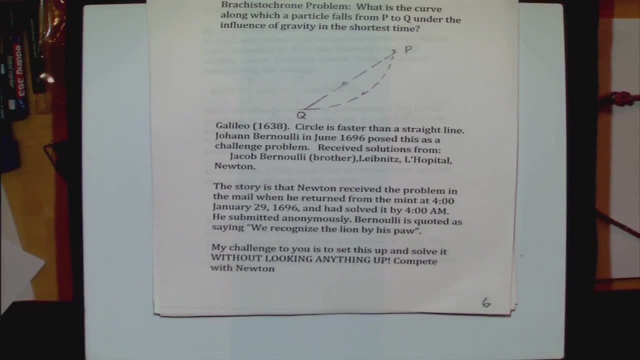 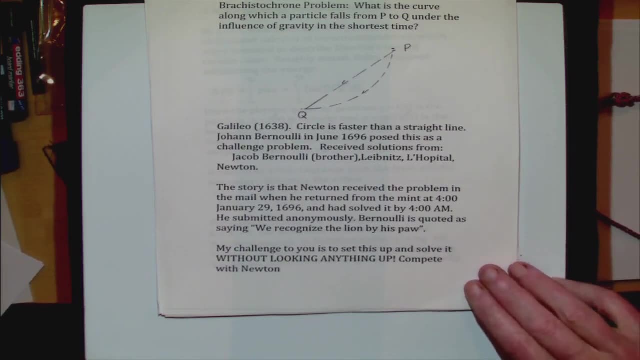 And the story of Newton is very, I don't know, It's supposed to be apocryphal, So, but he received the problem in the mail when he came back from a hard day at the Mint. You know he was. 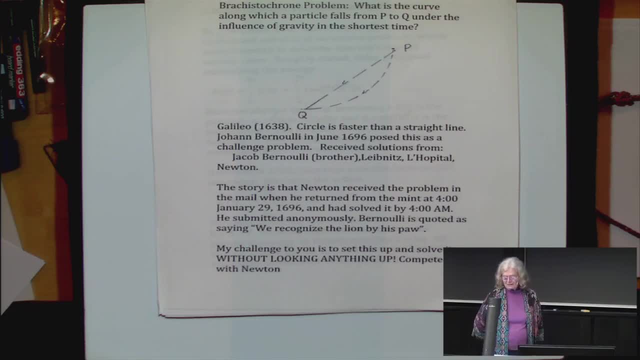 And by 12 hours later he solved it and he submitted it anonymously. And when Bernoulli got the solution, he read it and he said: we recognize the lion by his paw. Okay, And actually I have a challenge. 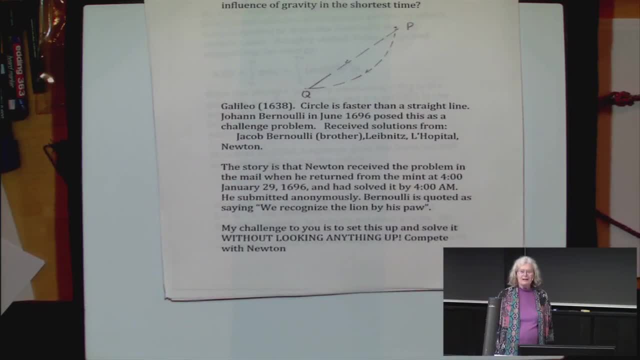 I have a challenge for you, because this just needs calculus. But I, First of all, you have to set the problem up, which is not trivial, And I don't actually know how Galileo did that, But anyway, you have to set the problem up. 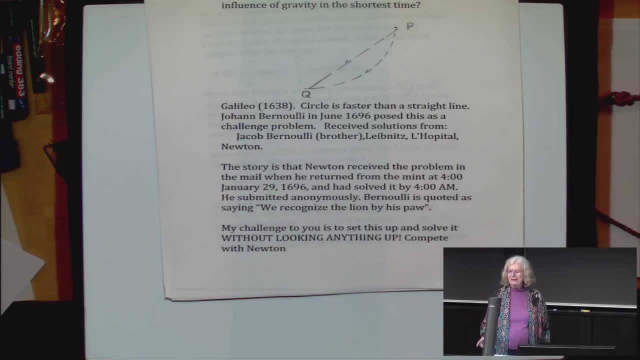 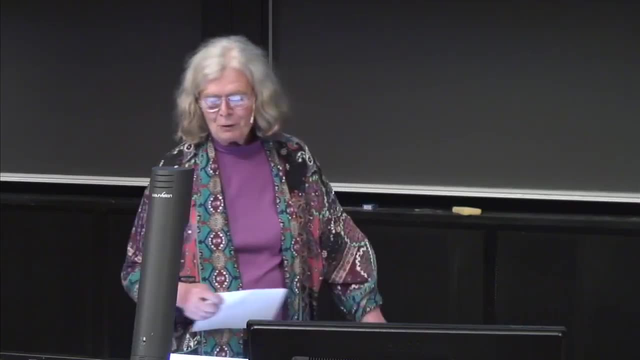 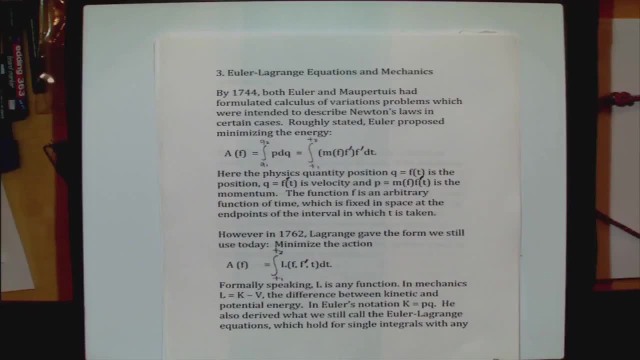 So we get into the really things. So we jump again, but not quite so much, to 1744.. By 1744, both Euler and Mopertus had formulated calculus of variations problems that attempted to describe Newton's laws. 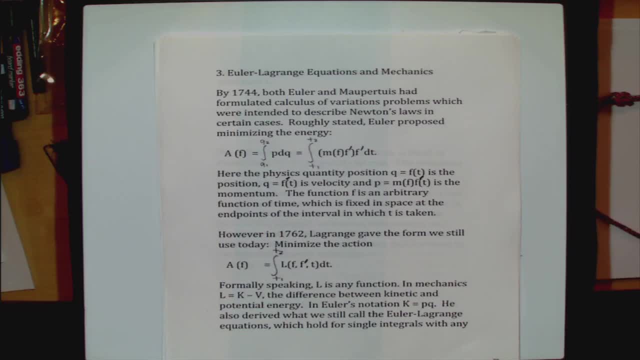 So Newton, Newton, Newton, I should say Newton. actually, The first calculus of variations problem is not the bachrystic home, Apparently he tried to compute. he formulated a problem about the shape of a rotationally symmetric solid that you could move through the air. 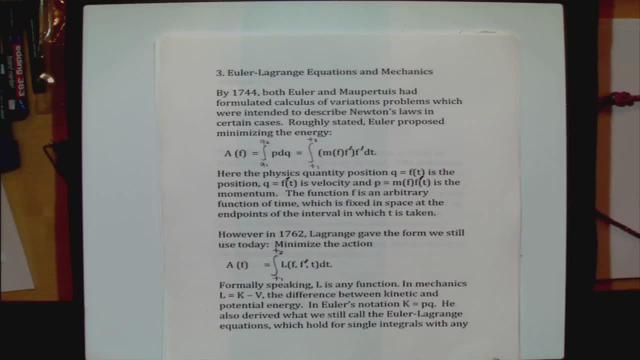 We don't remember, and he actually set it up and solved it. The thing is is the physics was wrong, So we don't remember that problem anymore, But in any case, by 1744, everybody was working at this point. 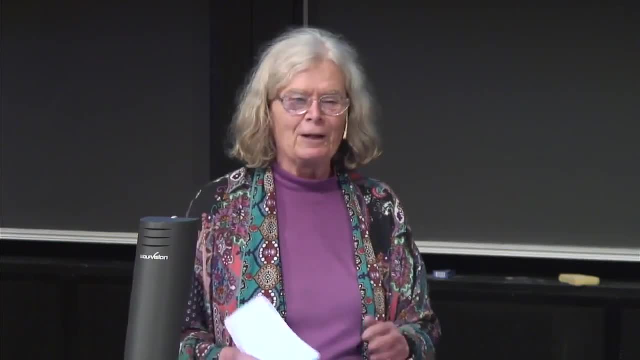 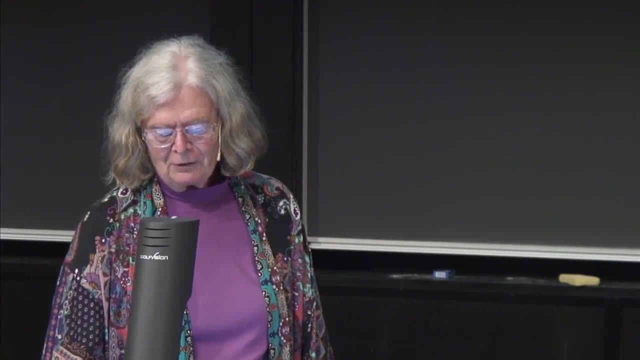 There was a whole gang of these people out there. I mean thinking of these lonely people lonely out back there. of course, they took longer to communicate with each other, But so- and in fact, Mopertus is actually often quoted. 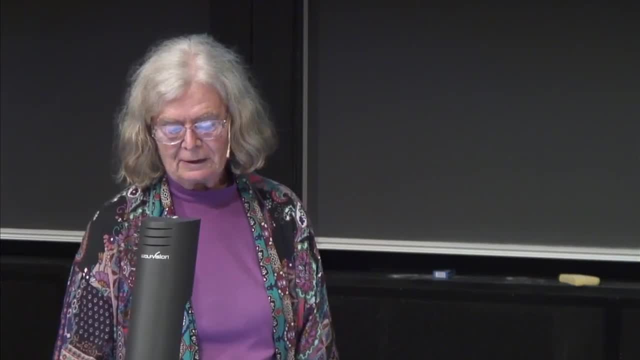 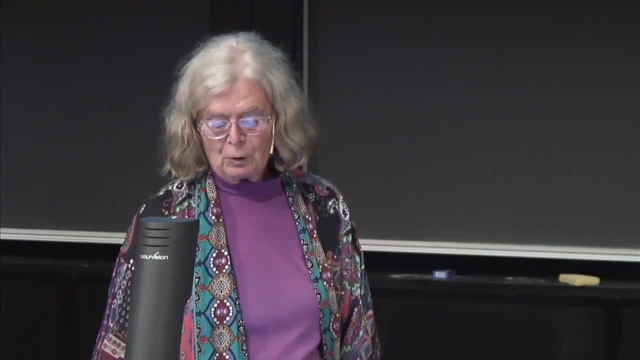 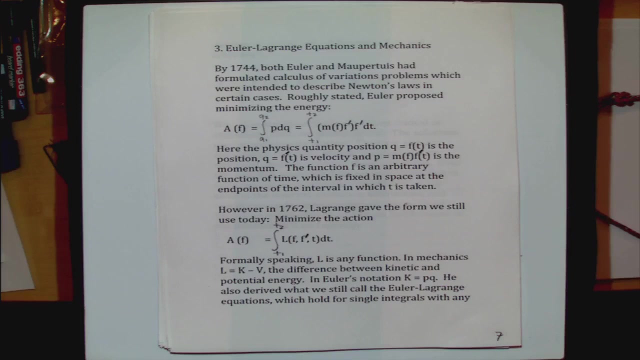 as the person to first derive the least action, least energy principle. But Euler proposed. I'll give you Euler's proposal And here the physics quantities are: position, which is a function of t. I've used q equal f of t. 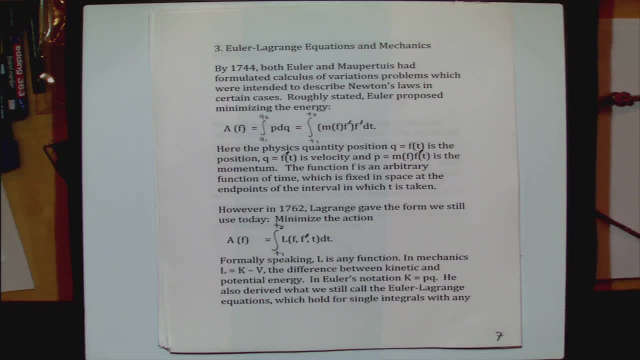 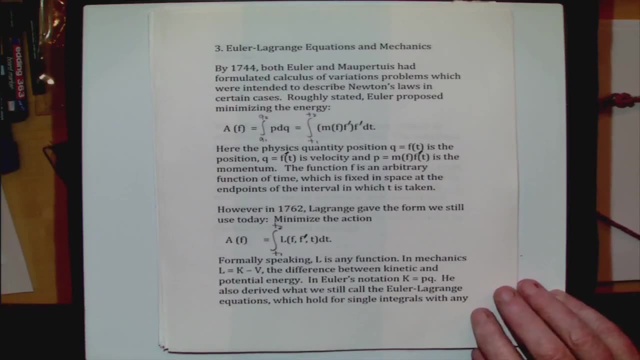 That's not the classical notation. Q is the classical notation, But we're going to see f throughout the talk. So remember f. f is the thing we're looking for in the whole talk, So we write down an a of that. 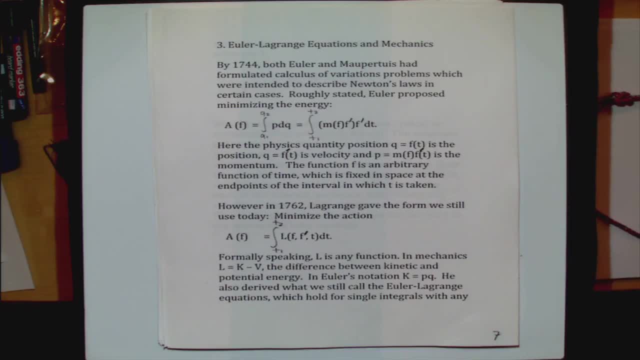 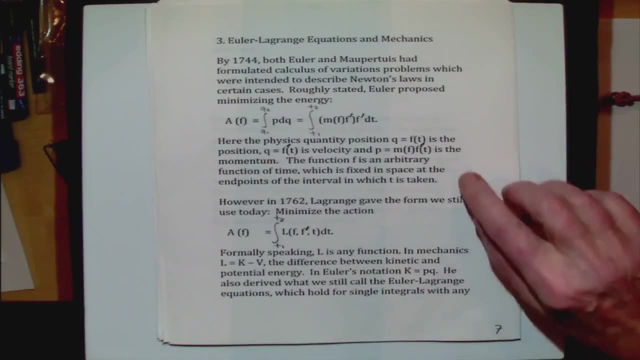 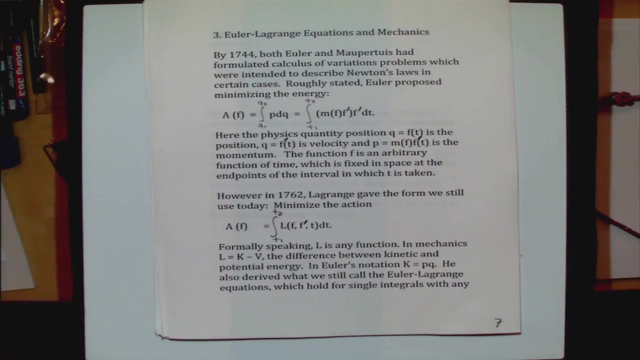 An. a is actually what we're going to minimize. So keep that in mind And that, And So the physics quantity is q and the position And the velocity is the derivative And the momentum is mass times the derivative. 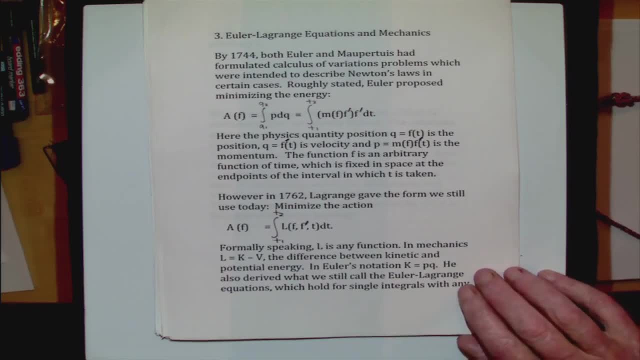 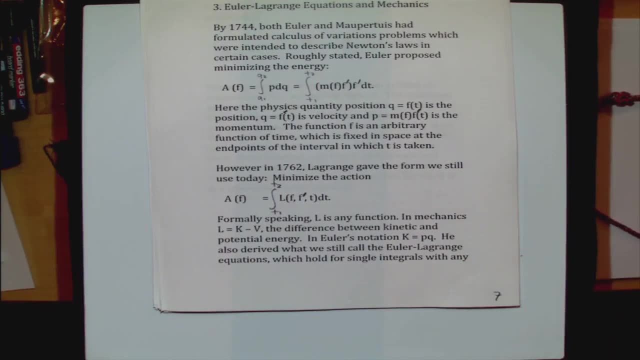 And the function is an arbitrary function of time fixed in space at the end points. But we've actually forgotten that because in 1762, Lagrange gave the form And everybody immediately dropped what they were doing and grabbed on to his idea. 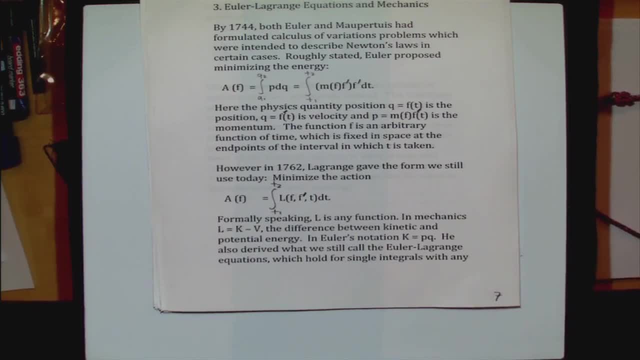 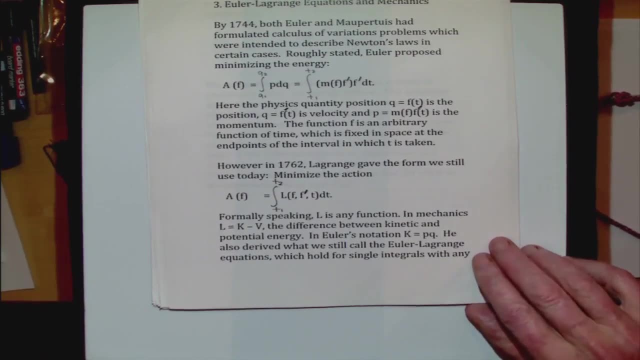 And so he actually wrote down an action. This is a for action, So that's classically in physics action. So you minimize the action integral, And here f can be any function, I mean l can be any function. 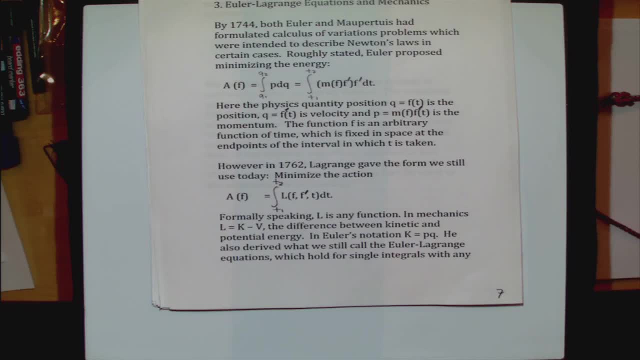 It doesn't have to have any meaning whatsoever. You know we're mathematicians, We can do anything we want. If you never wondered why people do mathematics, you should realize that If you're a physicist, you have to make sense of l. 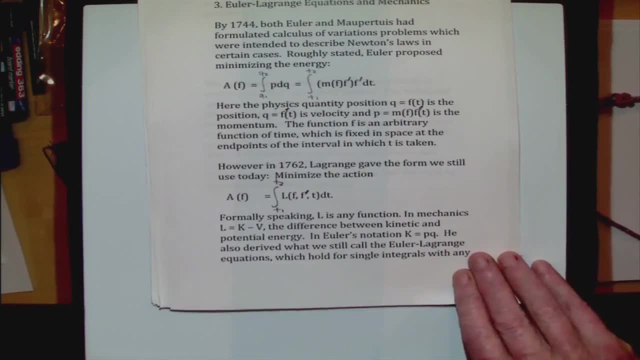 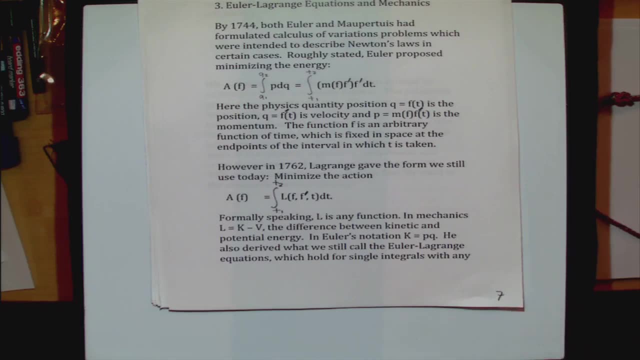 If you're a mathematician you can do anything So formally, And so in mechanics, l is the difference of kinetic energy and potential energy. So it is not a question of minimizing energy That minimizes the difference. 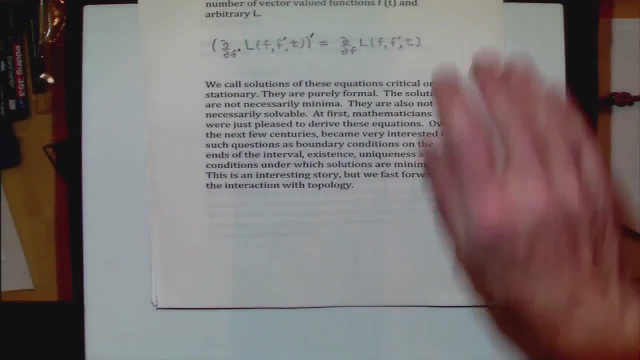 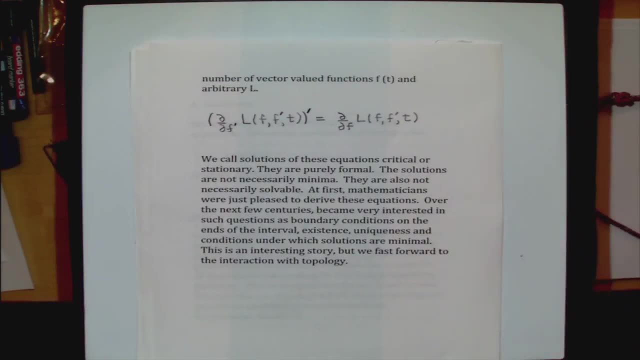 And he derived the Euler-Lagrange equations which look like this. And again, this is one of the few equations we'll see in class You take. This is grammatically totally incorrect, but most people understand. You have to take a partial derivative of l. 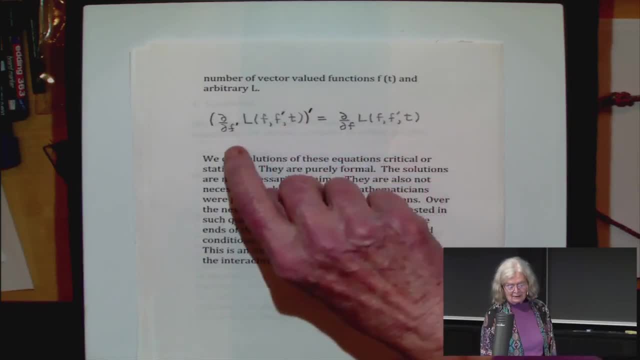 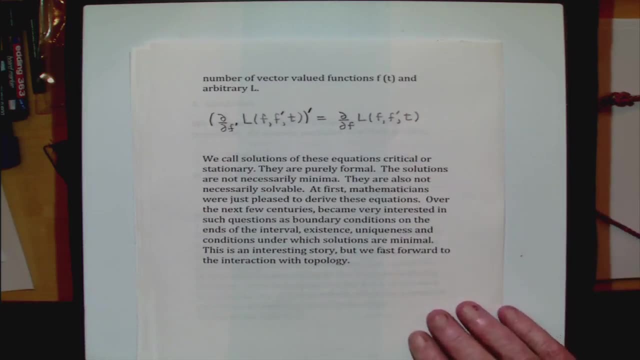 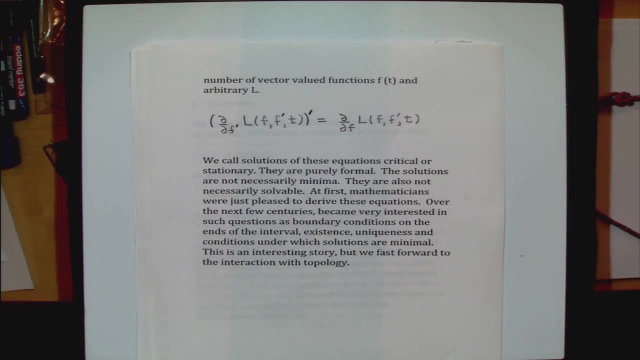 in the direction of the velocity, and then you take the derivative of that whole thing and that's the partial derivative of l in the direction of f. These are purely stationary solutions. These are called critical or stationary and they're purely formal. They can have no physical meaning whatsoever. 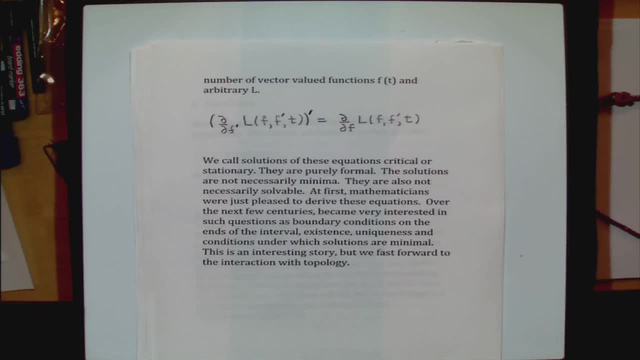 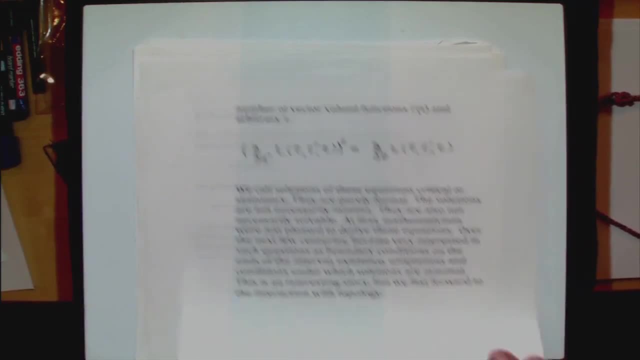 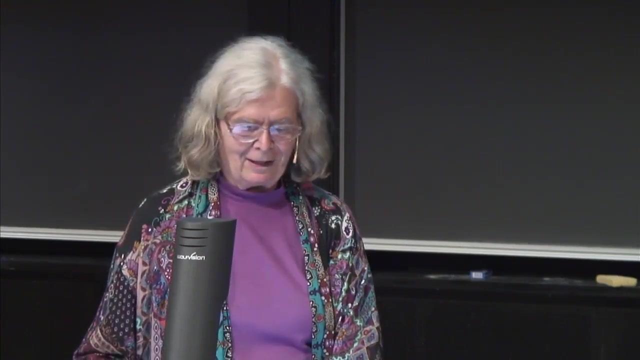 or you can have something that's not a minimum in any sense and it still has meaning, and it still has meaning. So we have to skip a whole lot, I'm sorry. There's a lot of good stories and so forth, but if I'm going to get anywhere near today, 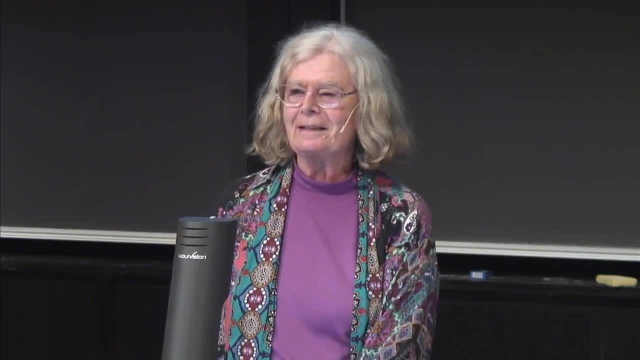 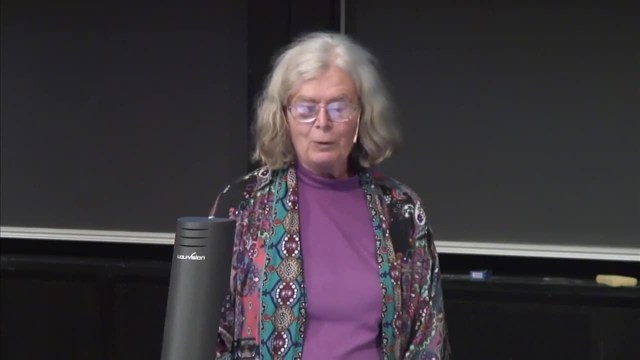 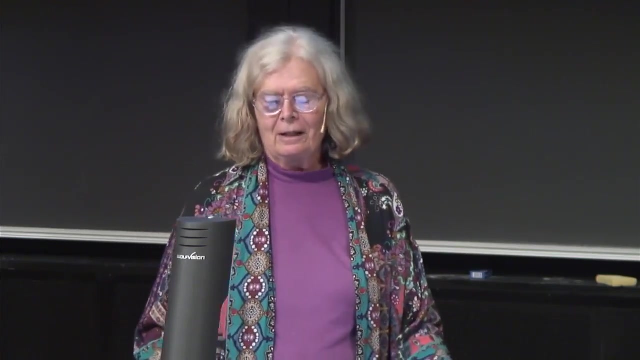 we're going to skip. We're going to go back to least distance, And something is least distance and we have to also talk about where it's least distance. So modern mathematics in geometry usually deals with something called a manifold. Now that sounds pretty terrible. 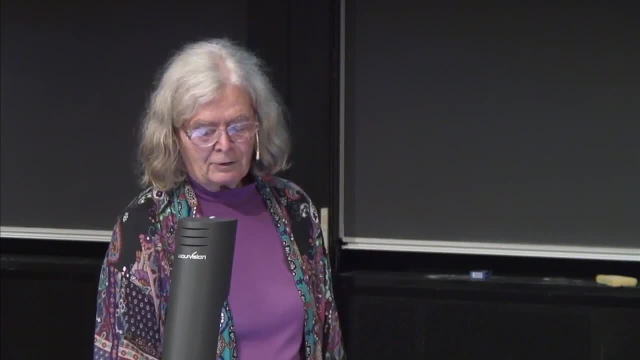 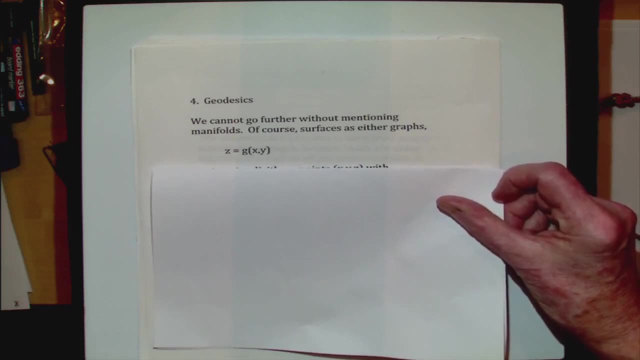 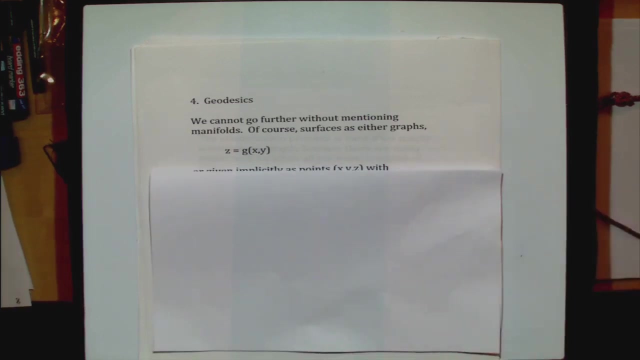 but of course Lagrange and so forth, and the physicists from way back of course knew about some manifolds because they wrote z is equal to g of xy and thought of that as a surface in space. And you also can write the manifold. 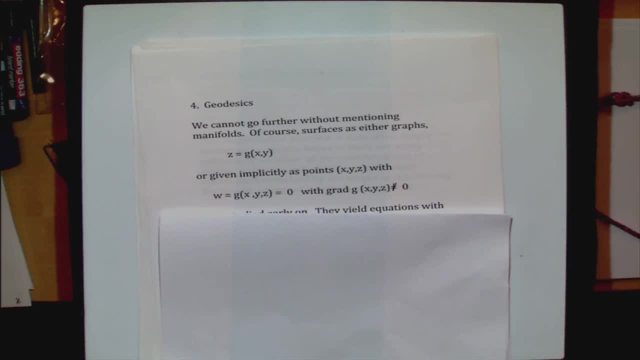 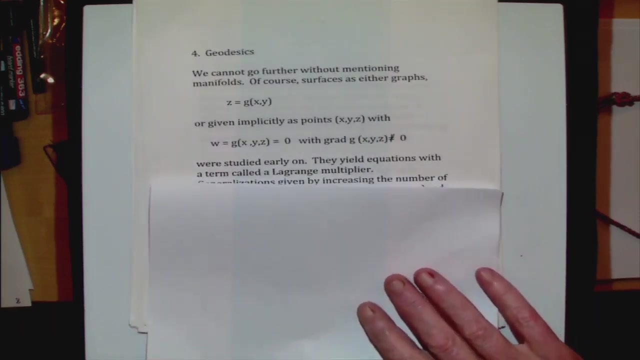 as given as an implicit function, the g of three coordinates. the function of three coordinates is zero and the gradient doesn't vanish. You have to use the implicit function theorem. So those of you And these were studied- I mean, I didn't even look up the history because 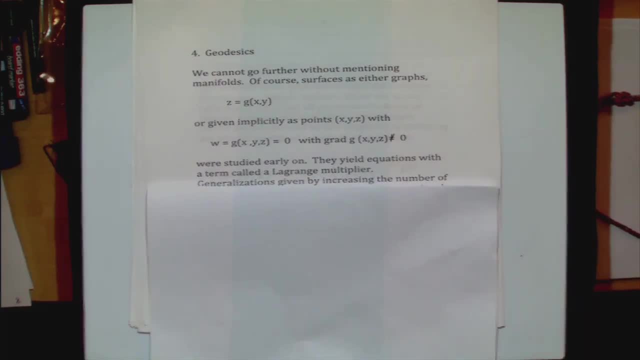 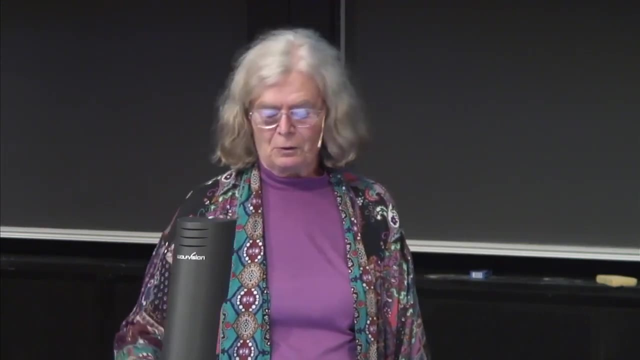 And they actually just yield the other Lagrange equations that we already saw, and there's something called the Lagrange multiplier that's thrown in there. So it's a little bit more complicated And you can generalize. See, we're mathematicians. 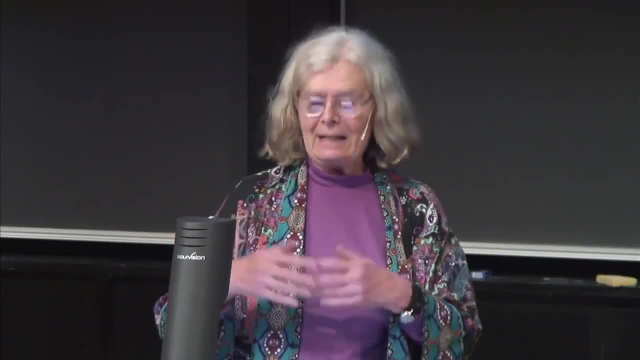 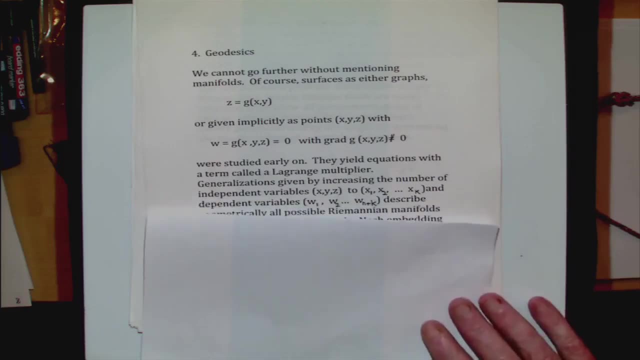 We can do anything we want. So we put any number of variables, we change x, y and z to x1,, x2 and so forth, xn And we change the w to any number of of variables. And this: 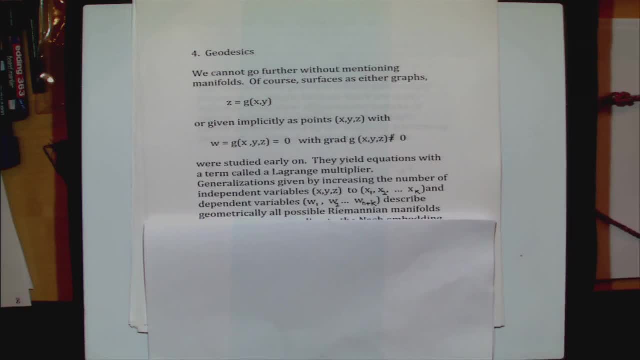 Now this might seem. Maybe there's something that we want to call a Riemannian manifold that isn't described this way, But it's a theorem of Nash, And Nash is one of the. I mean, I'm very honored to be one of the people. 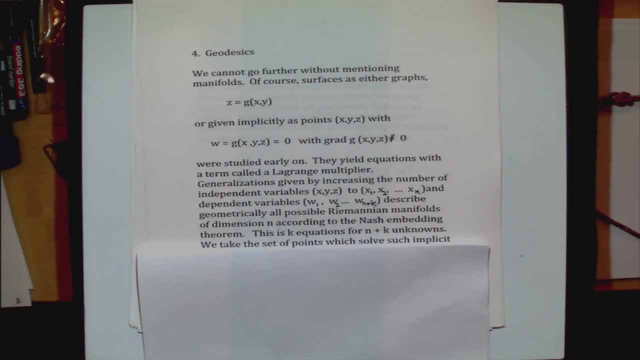 that share to get the Abel Prize. because Nash is important, work is very important. The Nash embedding theorem and what happens if you think about it is that you have k, You have n plus k unknowns, So five unknowns say: 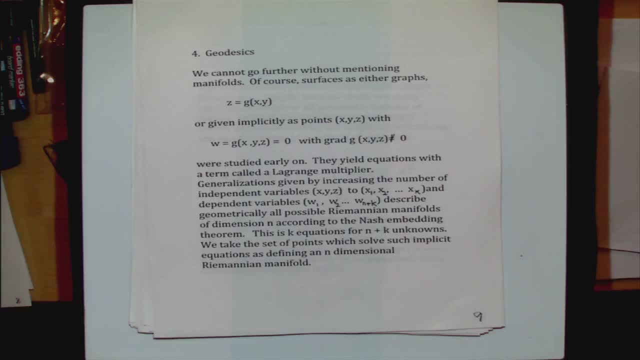 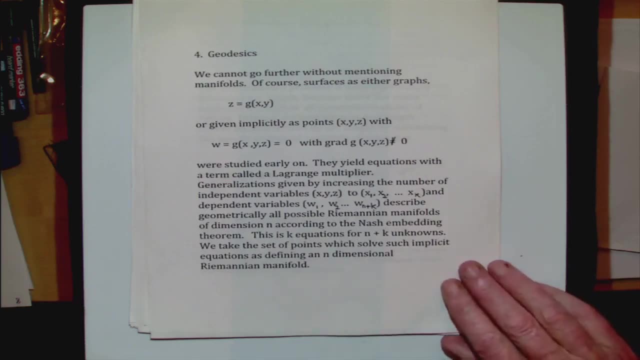 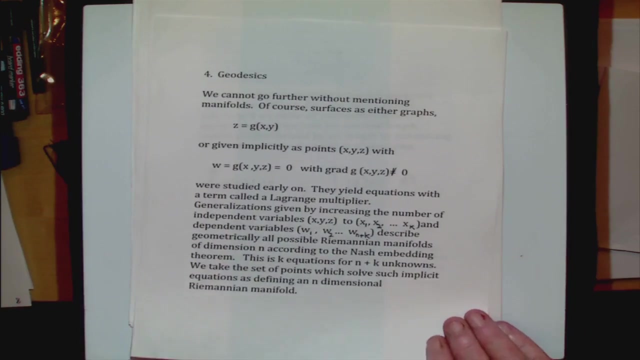 And you have two equations. You have, You have, You have, Sorry, k equations for n plus k- unknowns. Did I get that right? So we set the points which solve such equations as defining an n-dimensional manifold. So I think I got it right. 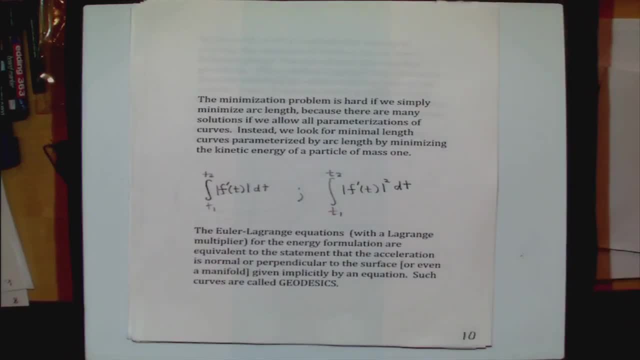 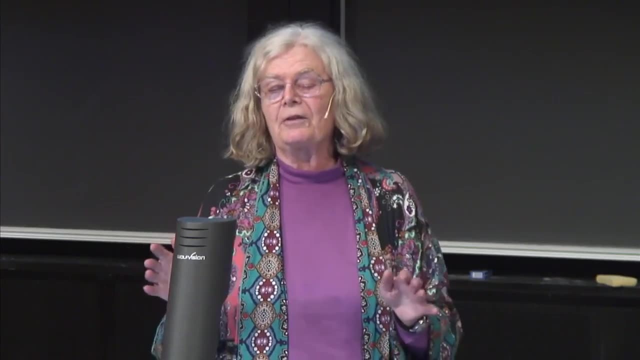 Oh well, Okay, So now we want to minimize, So we have- Think of We're in a big Euclidean space, Or you know, just think of being in a surface, in free space- And we want to minimize the distance. 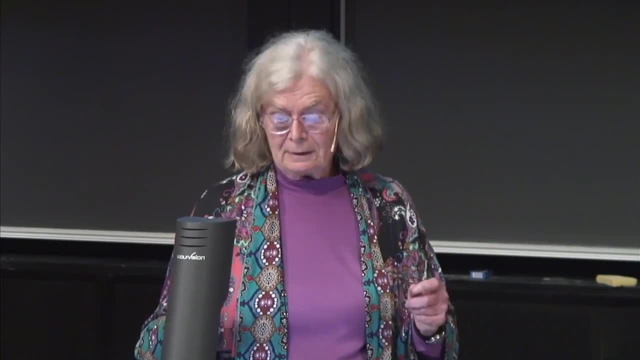 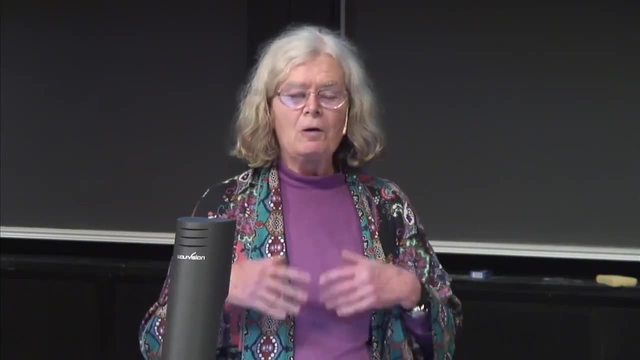 along that surface, And So we write down an integral which minimizes length. Now we come to a problem, And this all goes back. Remember, the Greeks didn't know how to describe curves. Well, when we run across this problem, 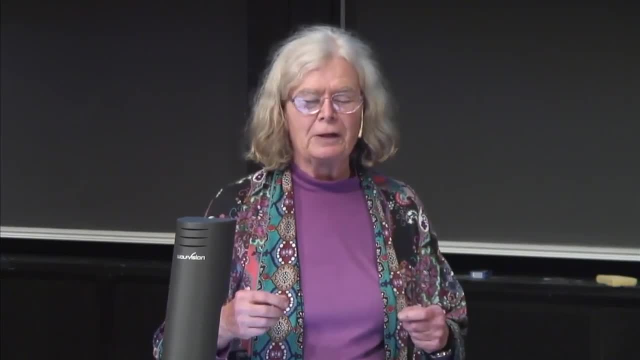 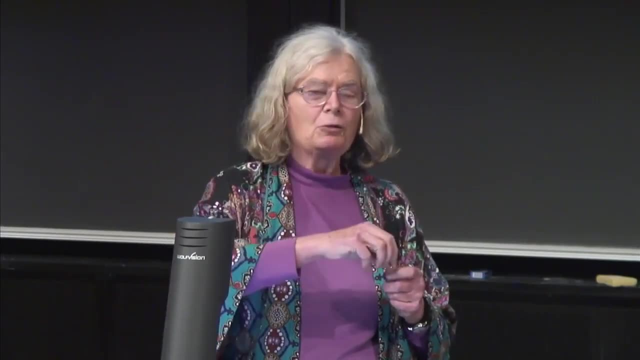 we run across another case where we don't. The description isn't very good Because if we actually parameterize a curve the way we want, a curve we have, actually We don't have a. We can just parameterize it in any way we want. 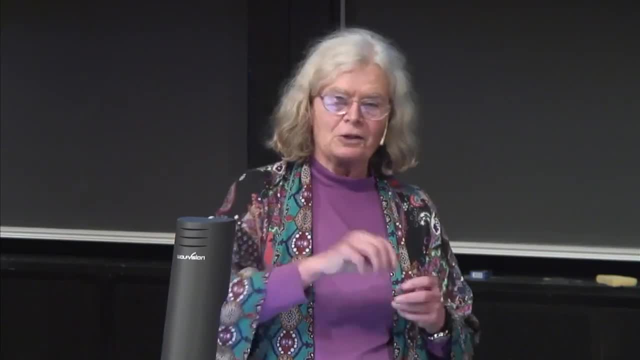 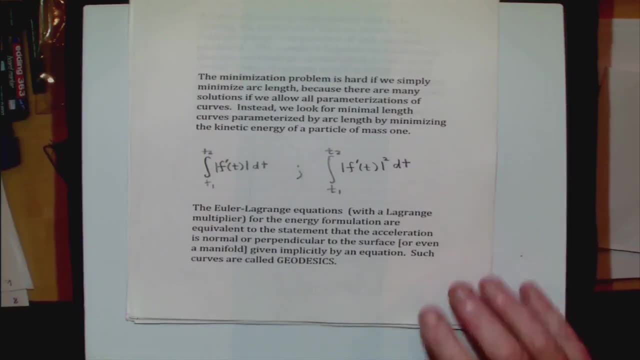 We can go along it fast at first and then slow, or slow and fast, And it turns out the way to handle the problem mathematically is to parameterize it according to arc length and parameterize it according to length And according to arc length. 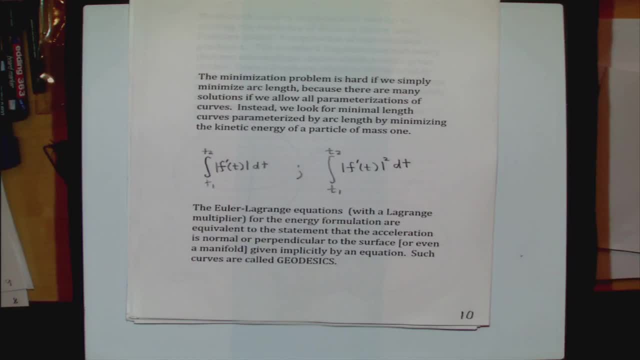 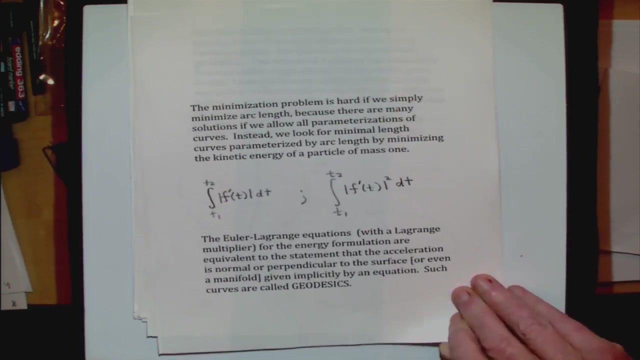 we minimize not the norm of velocity or speed, We minimize the norm of the velocity squared, And that gives us all the answers, parameterized by arc length. And So these curves are called geodesics, and they're very important in the development. 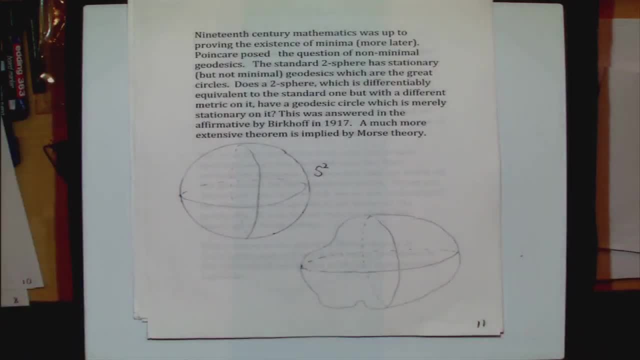 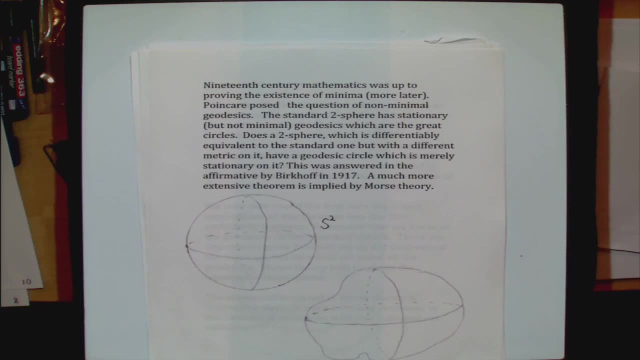 of geometric analysis. Oh, okay, Okay, So 19th century mathematics was up to proving the existence of minima. I mean, I'll explain a little bit why that's so. And so if we Again this, 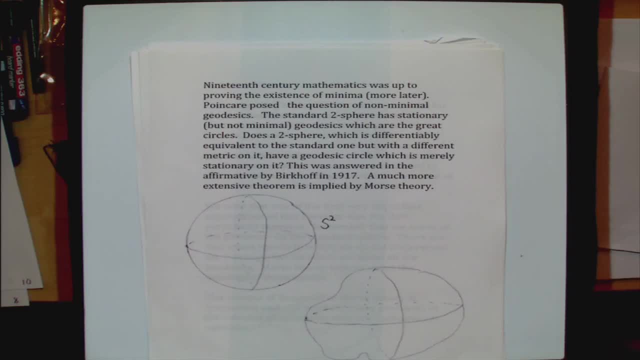 Around the turn of the century. this was of the Sorry, the turn from the 19th to 20th century. This was a question of real interest. The question came up. if you have, I'll give the explicit example. 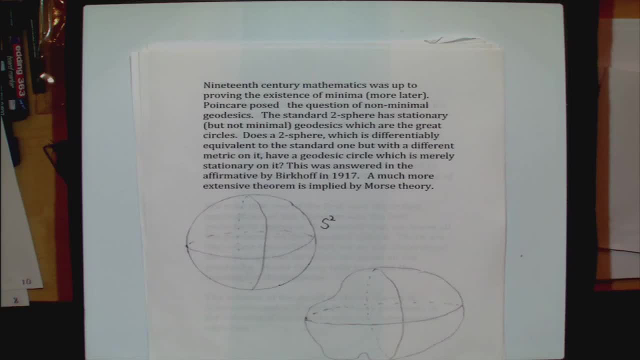 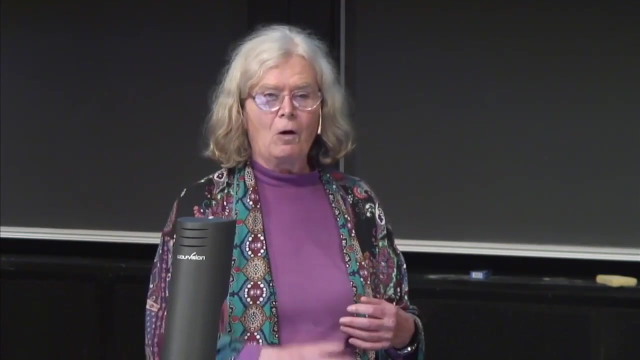 The question was: if you have a manifold, how many closed geodesics are there on it? That is, a geodesic that comes back and meets itself. Now, if you're on the regular two-dimensional sphere, you know actually what all the geodesics are. 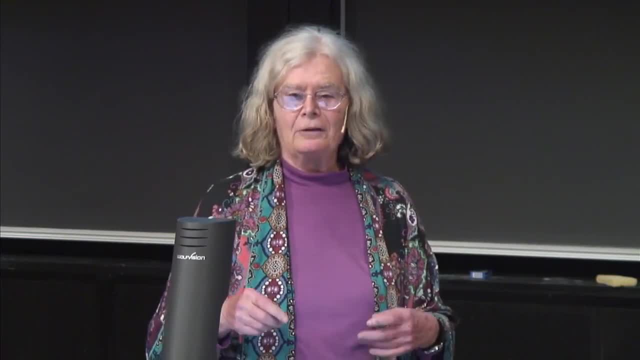 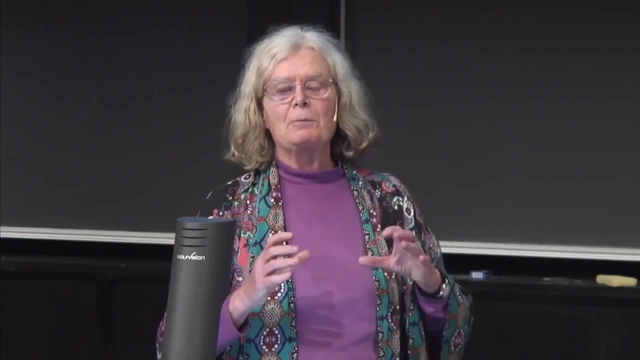 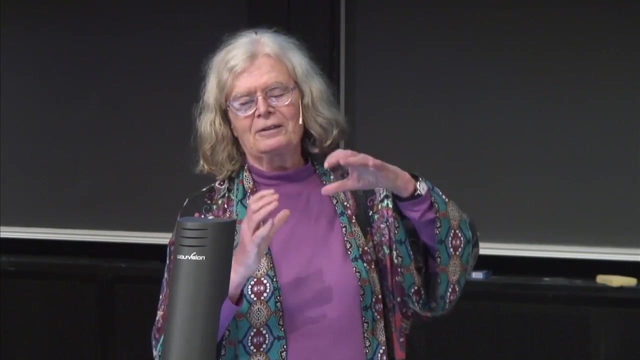 They're the great circles And notice the great circle that goes around is not minimal because you can actually slide it off, But it is a place where the energy has zero derivative. That is, if you look at the Slide, the circle to the top and the bottom. 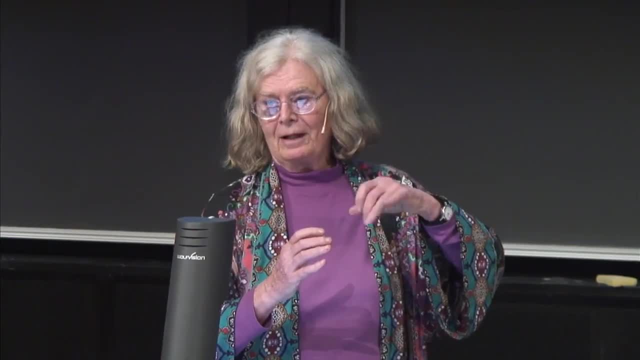 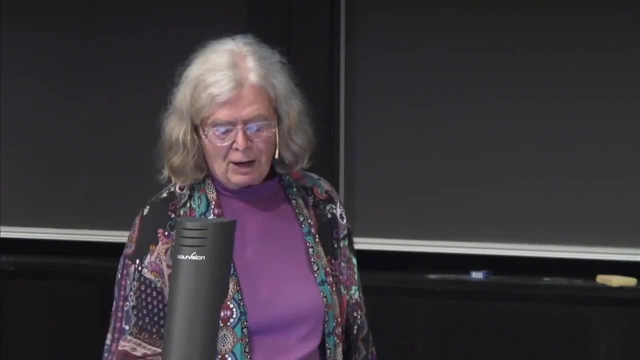 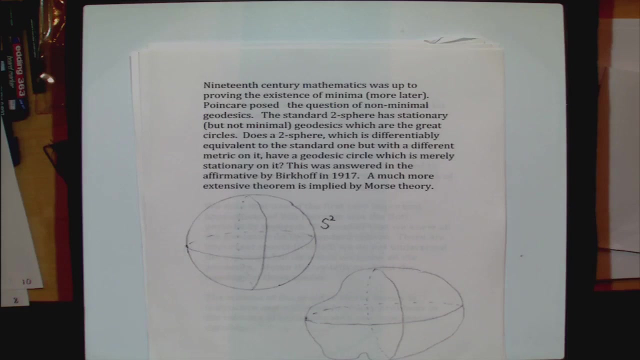 the first derivative is actually zero And it's the second derivative that actually takes you down. So if you have an ordinary sphere, you actually have a lot of these closed geodesics. These are circles that are, And of course you do see. 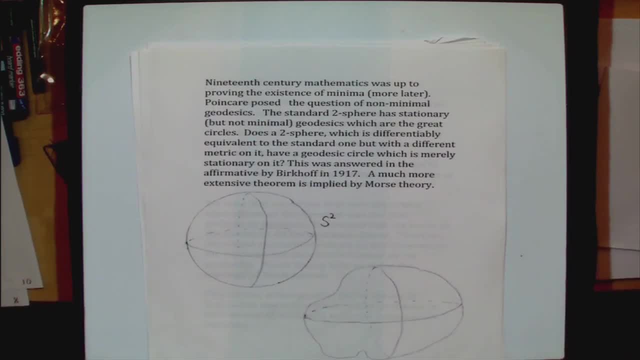 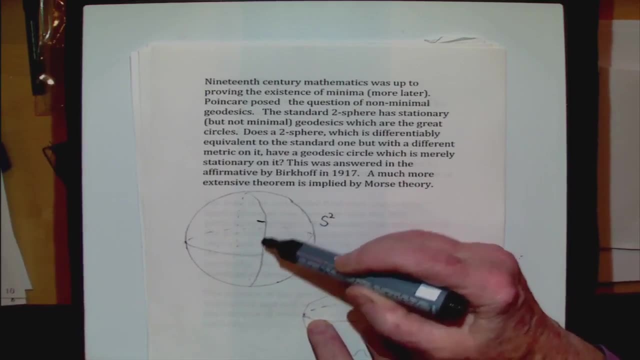 that if you take two points on here I'm not, Oh, here I'm not, I haven't given this talk a lot. So if you take two different points on here, between here and here, it is minimal, It's just. 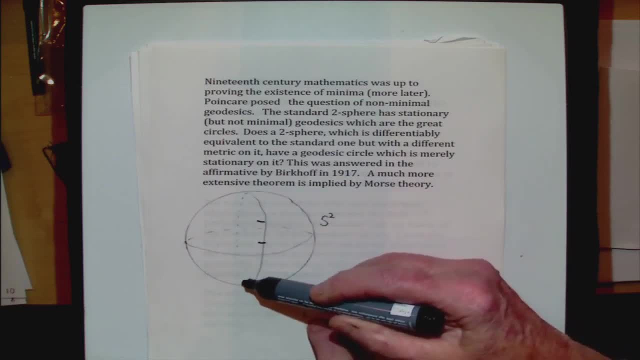 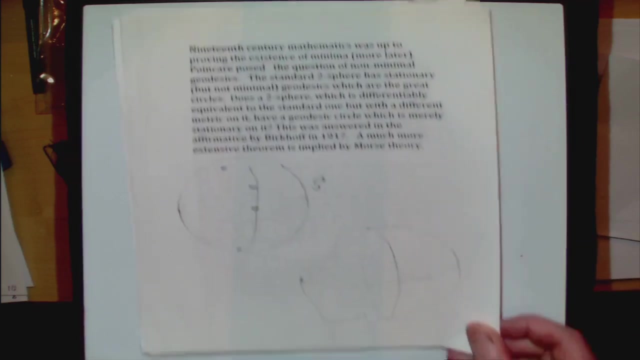 But when you go up and go past the points and you go from here to here, this is minimal, but this is not minimal around there, And so that was a phenomenon that had been well studied in the 19th century. So if you actually change the shape of this sphere, 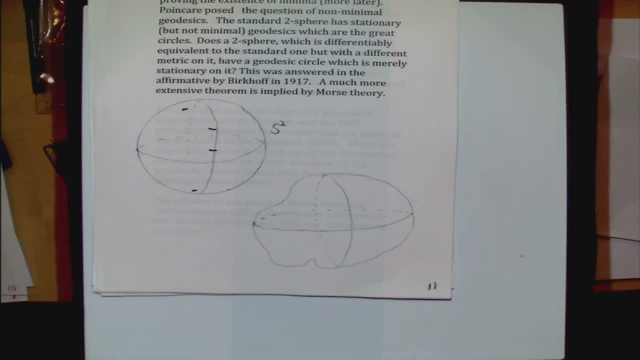 the question Poincaré asked was He actually asked: are there still three? Now that's a little bit of topology to argue that there should be at least three left, But But you see they would be, But you wouldn't have all the great circles anymore. 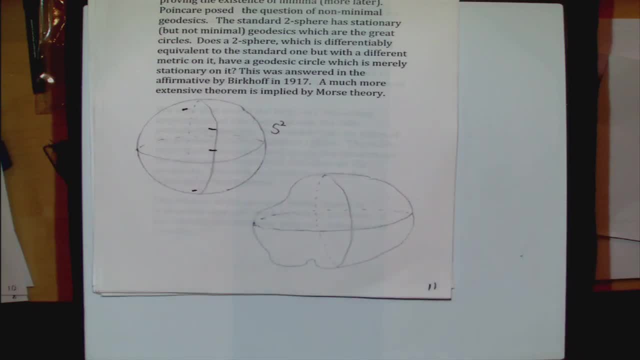 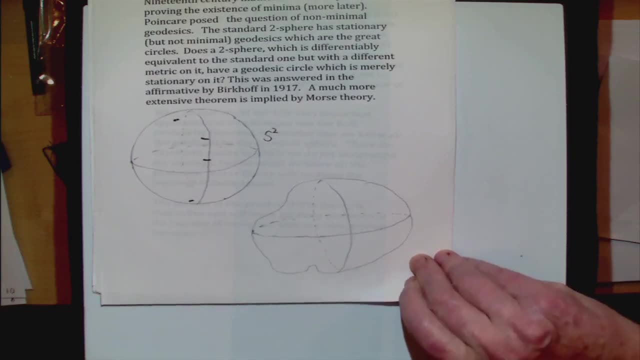 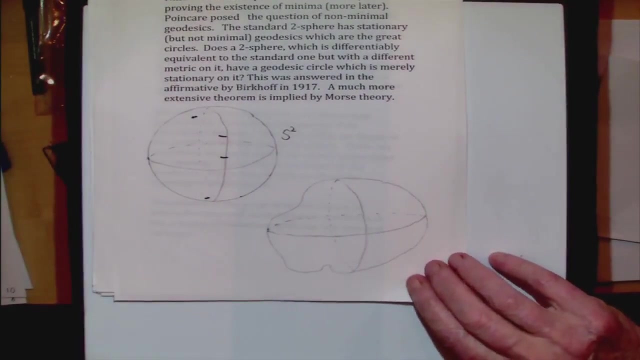 The claim is that three of them would survive, And actually this is a very hard problem which actually only was only solved in the last few decades. It's not, But in fact Birkhoff gave a positive answer that there was actually one that survived. 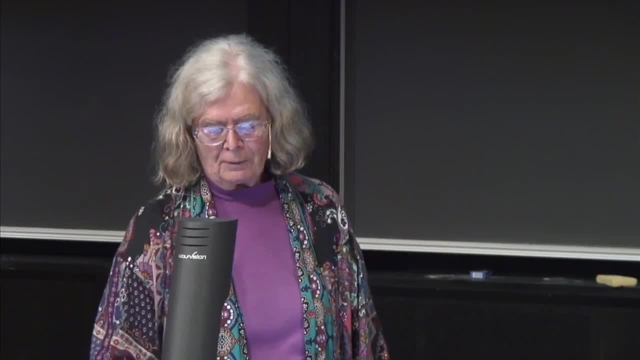 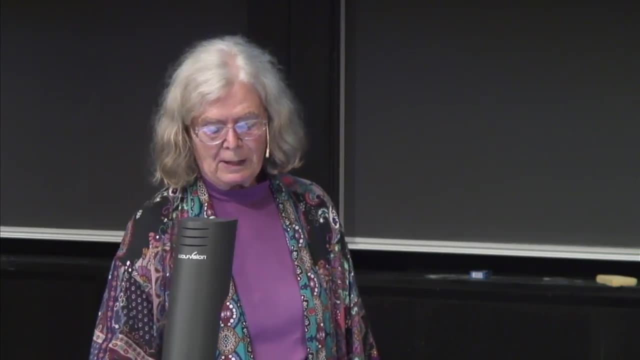 if you deformed the two-sphere, So. So a much more extensive theory is implied by Morse theory. So I'm going to explain to you about Morse theory, because what I'm talking about that's a very important idea, OK. 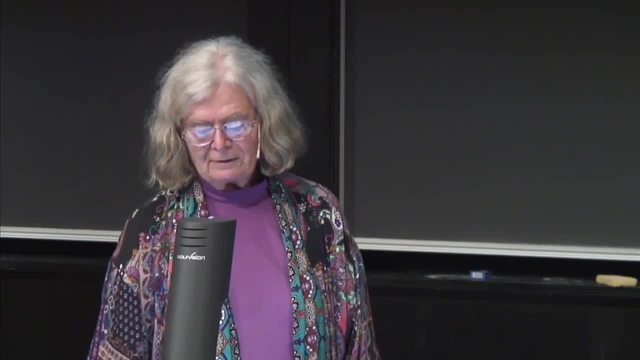 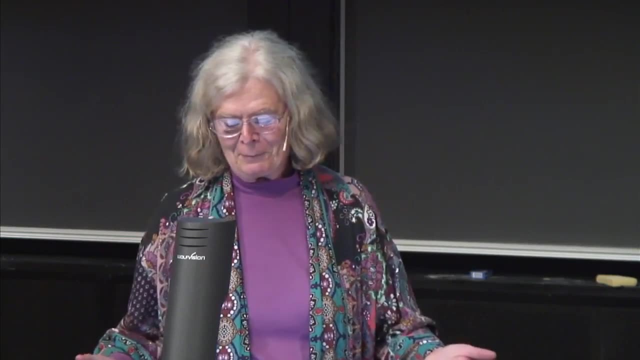 So understanding Morse theory requires quite a bit about the subject of topology, And we don't want to go into that here. That's too Well, we'll do a little bit, but So we'll think of it as a black box. 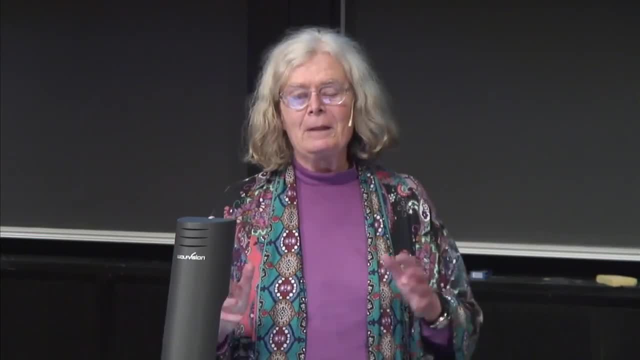 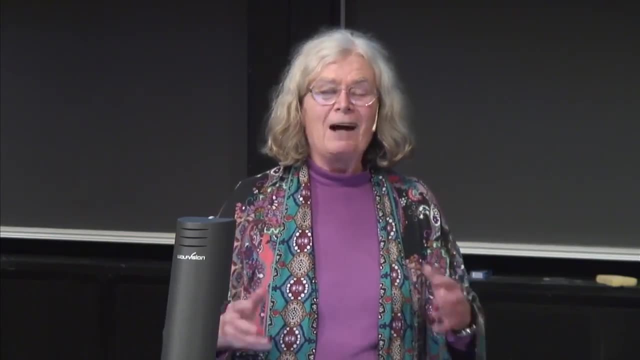 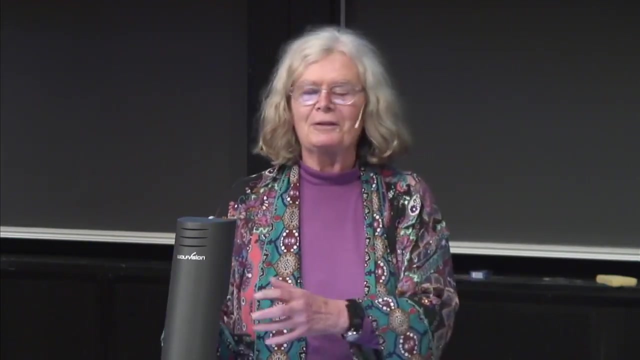 It's, And I should tell you that at the time Morse was actually doing his work. The topology he was trying to do was not really well formulated, So he was actually struggling with proving the theorem about geodesics. He was also struggling with what topology was. 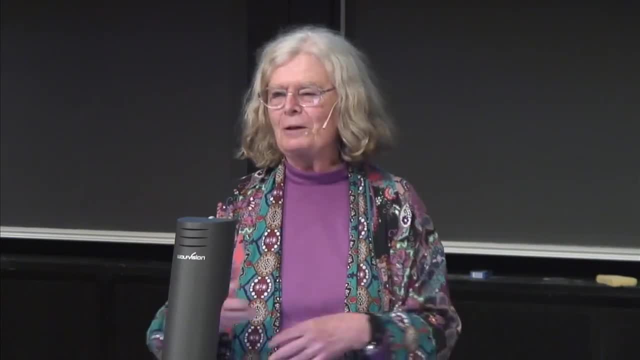 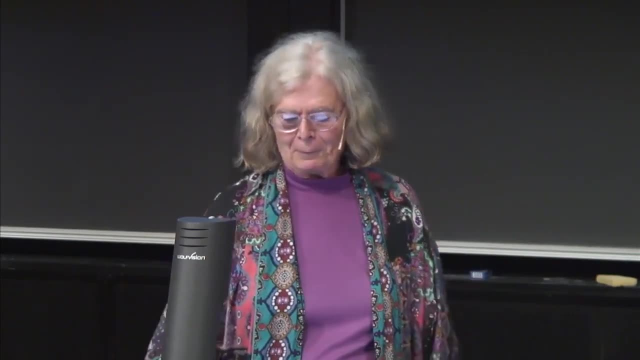 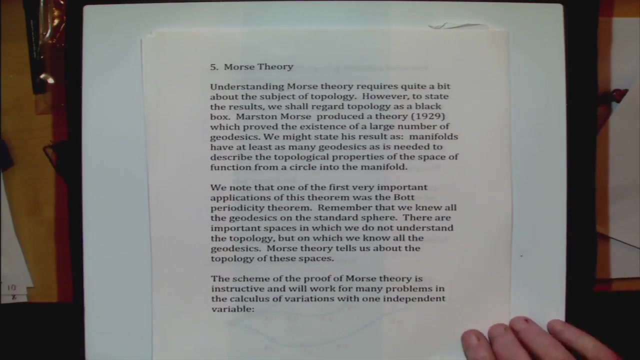 And nowadays, of course, it's something you actually learn. You certainly take a course in topology as an undergraduate in mathematics, But But- And all graduate students know a little bit about it anyway. So But at the time that Morse was working, 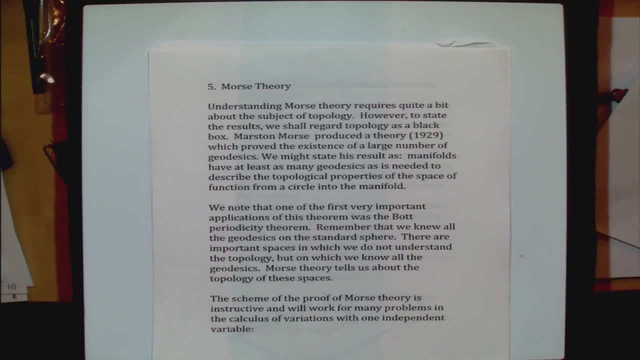 the. It really wasn't well formulated, which is very interesting, because if you try to read his paper, his book- actually it's a book- you'll find yourself struggling from the point of view of the topology more than anything else. 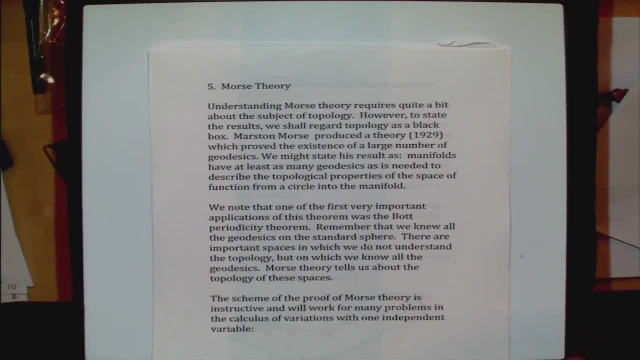 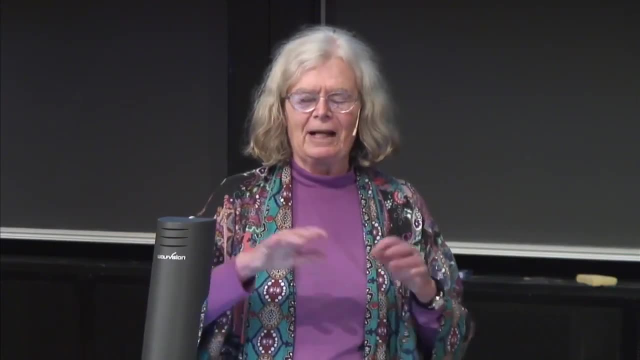 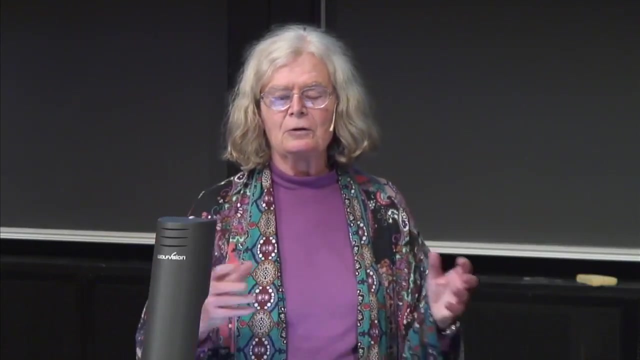 OK, So. So the claim is that if you have this manifold- remember that it's some extension of the idea of a surface in three-dimensional space- that you're trying to describe the topological properties in terms of these shortest distances. And I want to also point out that 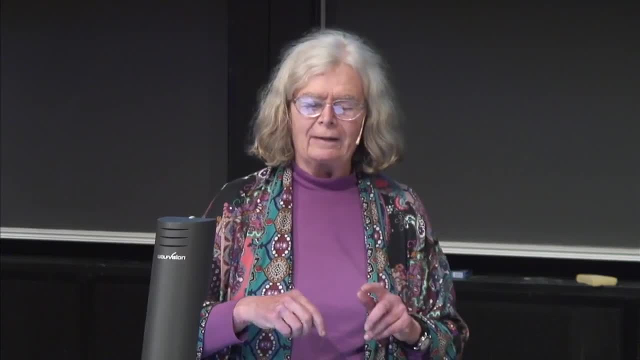 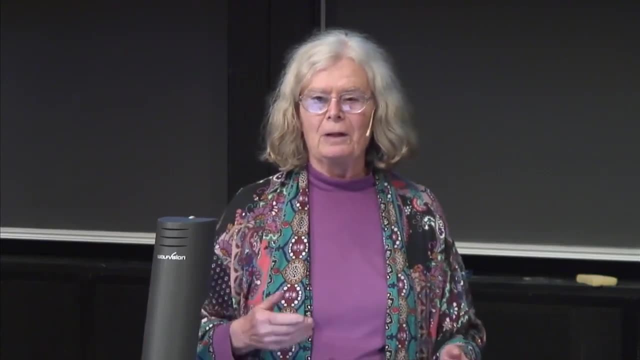 you think You've asked the question one way, that is, is there a geodesic? But in fact one of the most very fundamental applications was the other way around. It's called the Bode periodicity theorem And there's some manifold. 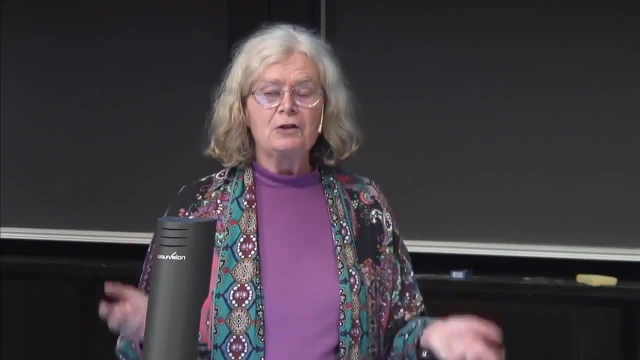 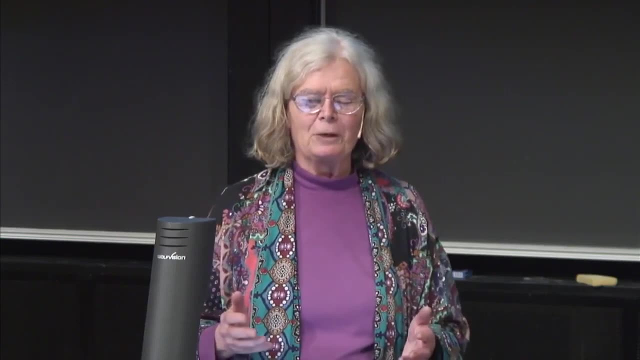 and there's some manifolds called Lie groups and we know all the geodesics on them because they're so symmetric and there's group theory and there's all this material, all this stuff we can do. So we know all the geodesics on them. 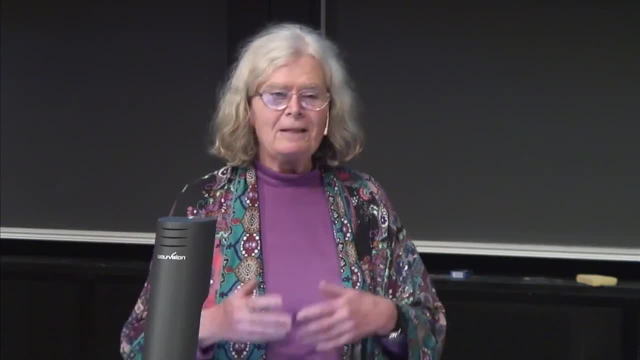 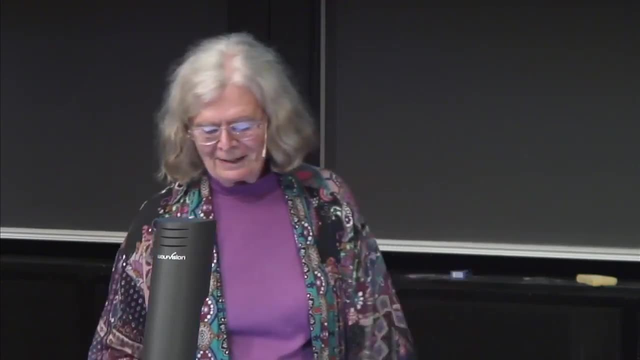 but we don't understand their topology, Because I mean, these are big, Some of these groups are very large-dimensional and even mathematicians can't think that big, And so, But it turns out, since we know all the geodesics. 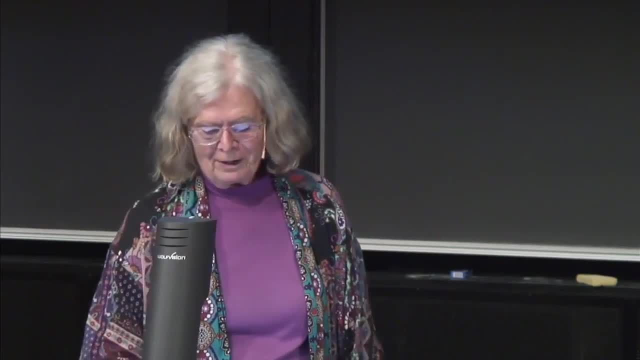 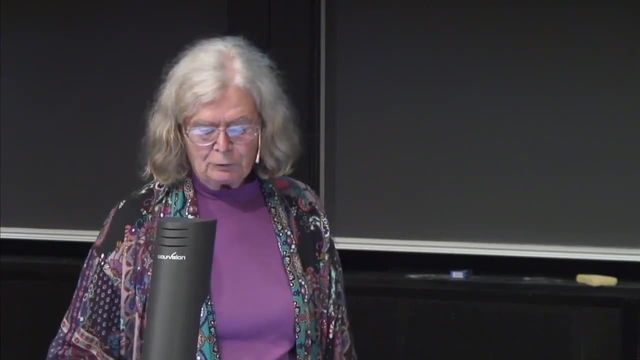 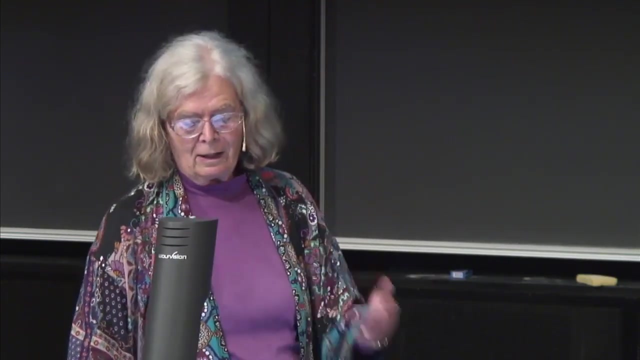 Morse theory tells us something about the topology. So that's to give you some idea of why it's so fundamental. So the scheme of the proof is instructive, and I also. It also explains why, Historically, why what I'm talking about. 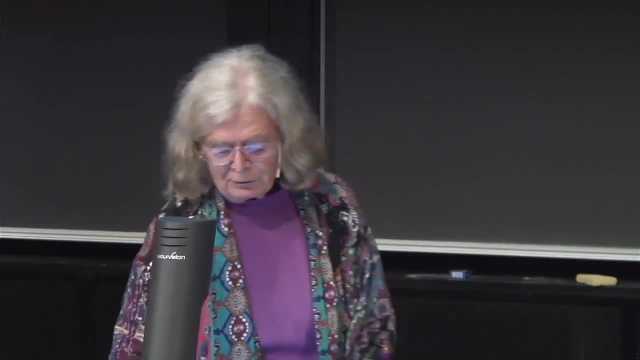 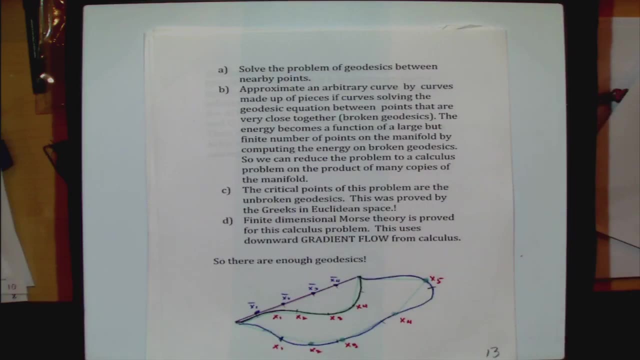 describes some of the history of what I'm trying to talk about. So the way you go about it is to solve the problem of geodesics. you take an arbitrary curve and you actually sort of put a bound on the energy of it. 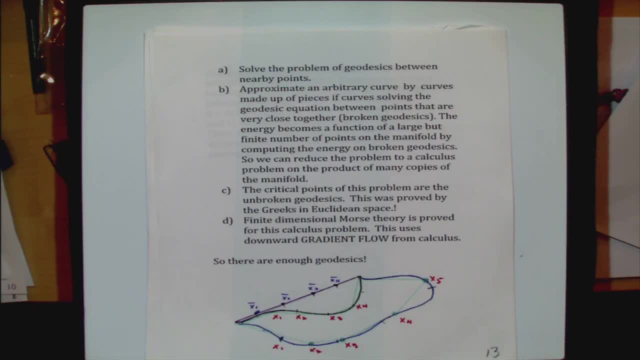 because you're trying to minimize energy, and so you. It turns out that you divide the curve up into a certain number of points and you solve the problem of the geodesics between nearby points. Now, this is something you could do classically. 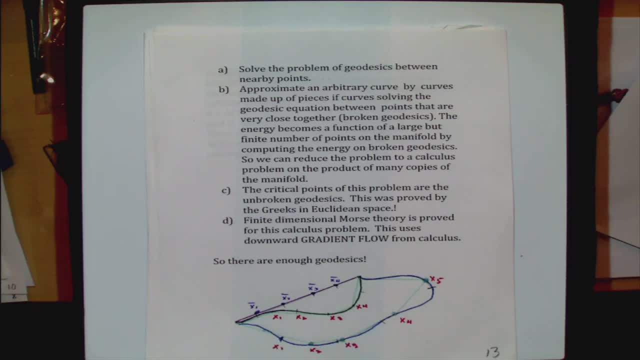 So this could be done in. People knew they could find the distance between two close points classically, And so you solve that. Now you actually look at the energy on this broken geodesic And you actually. Now this is. 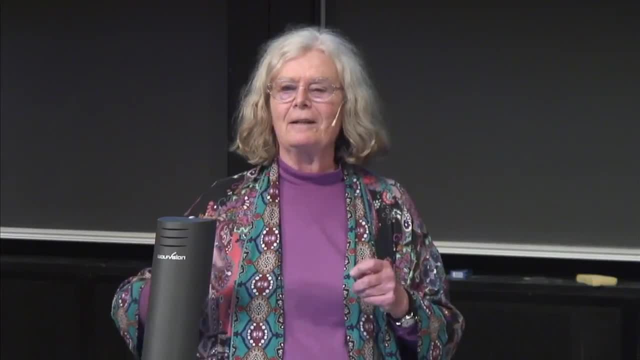 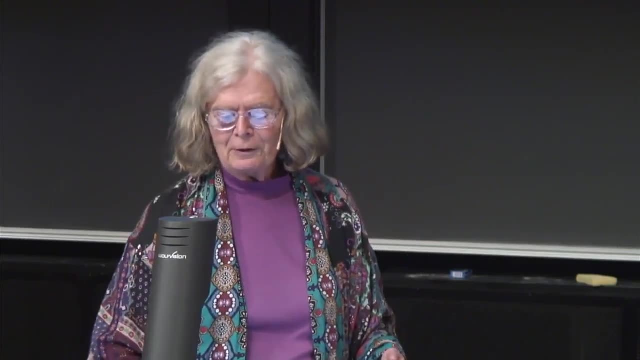 There's a finite number of points. So this is an energy on a finite number of points. It's a calculus problem. So you know the calculus problem, You know. You know that You know theorems of fact, the existence of minima. 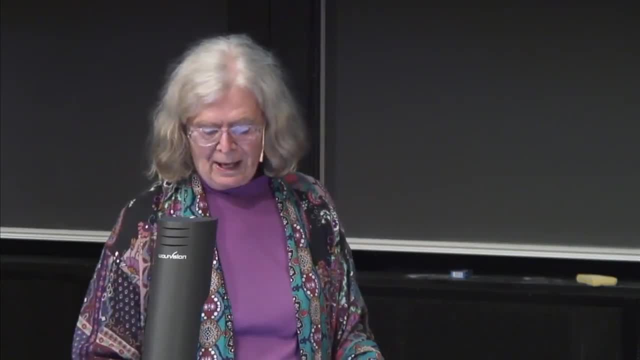 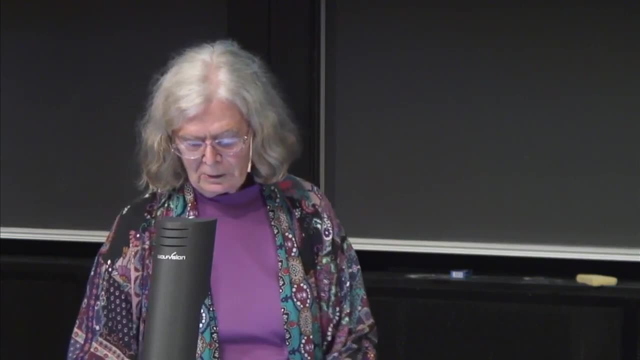 You can take gradient flows, You can do all this, And so what you do is you use the gradient flows on these broken geodesics. OK, The simplest application is the mountain pass lemma, And this will explain a little bit about topology. 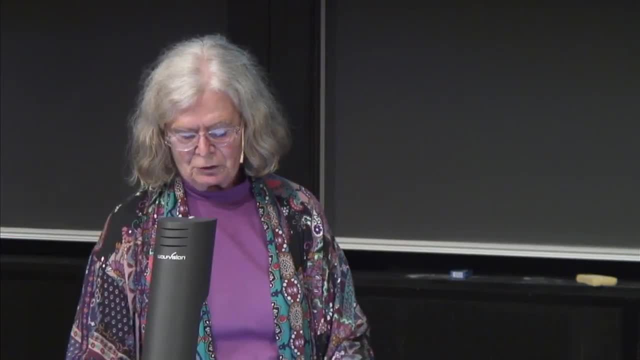 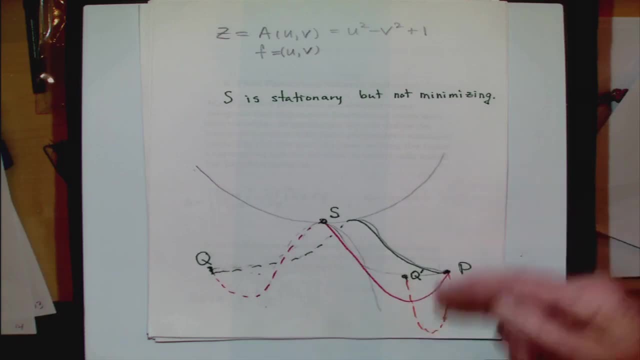 OK, So here I'll just. I'll just draw the picture here. You could actually do an explicit calculation where you have- I've used new variables- u and v, so we don't mix up with what we said before. So we have z as a function. 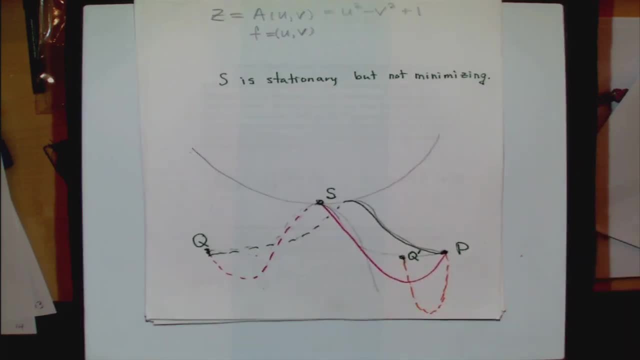 of u and v, And So we have z as a function of u and v And So f here. I'm sorry, This is actually a. This is our action, is z this time. So we're way down. 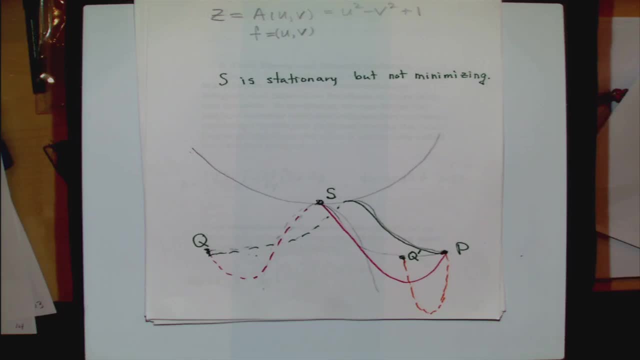 in two dimensions instead of looking at curves, And we're looking at function, at minimizing the height function. Now, if I take two points, p and q prime, and I try to connect them with a, with a path, actually I can make the 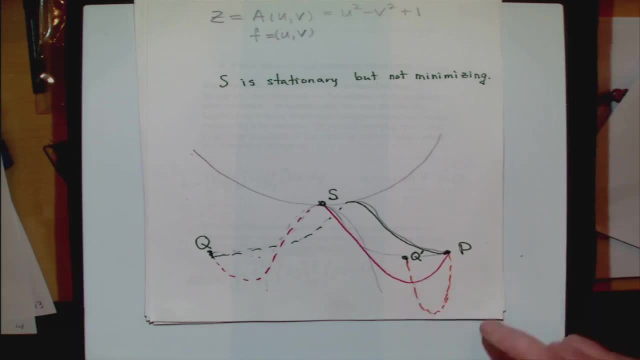 the path go down as far as I want, So I can actually connect p and q by a curve that stays at the same level. It doesn't, But now if I take the q on the other side of the saddle? Oh, by the way, 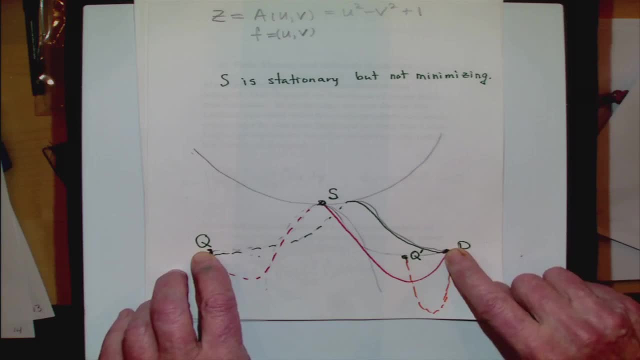 this is a potato chip. We always called it a saddle when I was a kid, but it's now called a potato chip. So you want to go from here to here and you want to go with. You want to go, so you take. 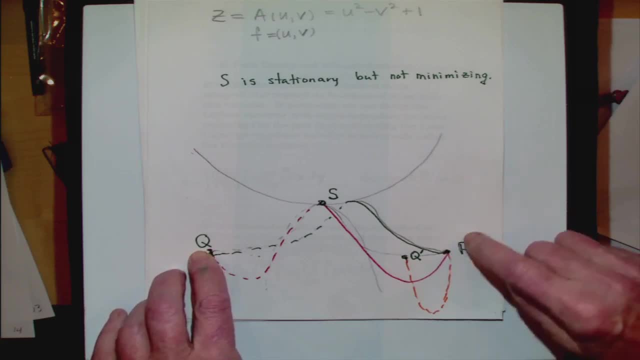 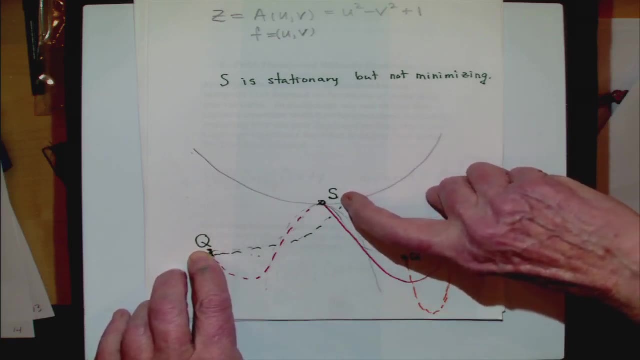 the minimum of the maximum along the path. So you go along here and you say, oh, this is the maximum here. And you say, well, I could have gone down a little bit. And you test it out and then you discover that 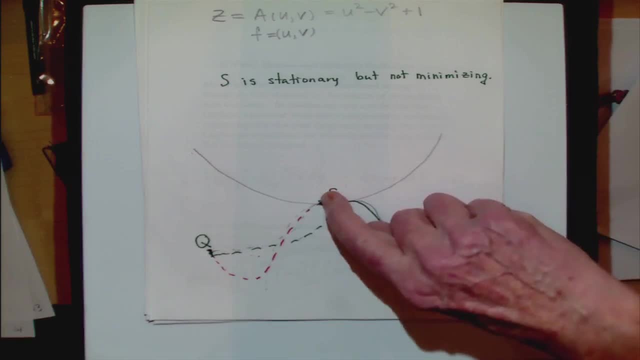 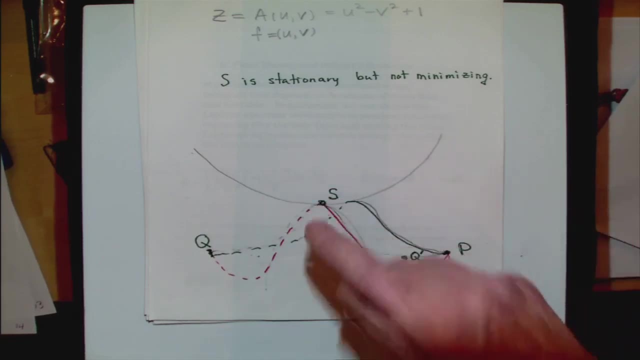 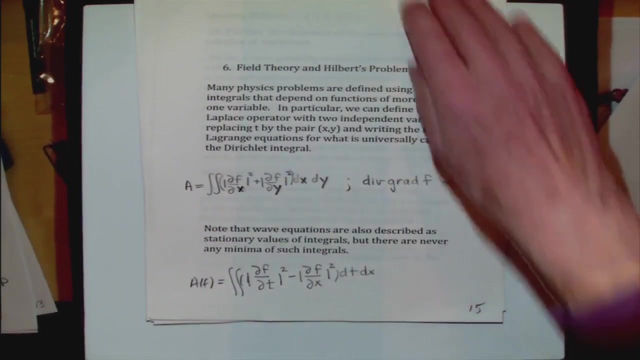 yes, the minimum of the maximum is this point here, which is a critical point, but not a minimum. But notice, it has one direction up and one direction down, So that's Anyway. Okay, So we're getting there. 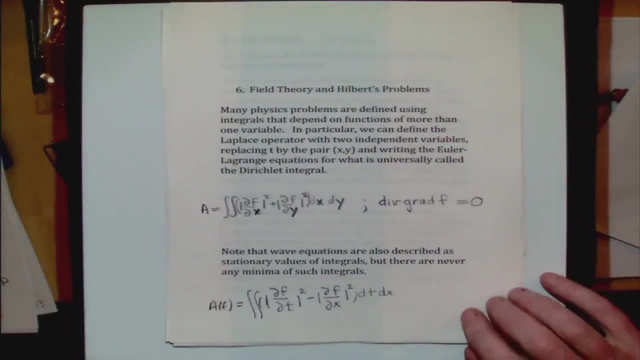 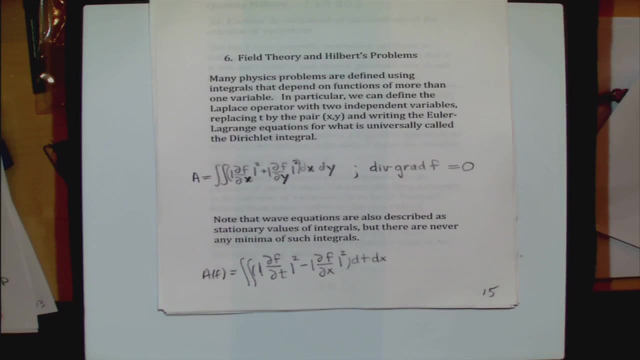 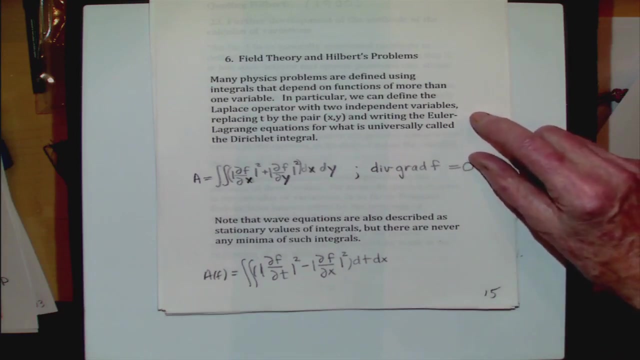 So now we come to. Many physics problems are defined using integrals that depend on functions of more than one variable. We can define the Laplace operator, which I hope some people are familiar with anyway, of two independent variables. So we're putting 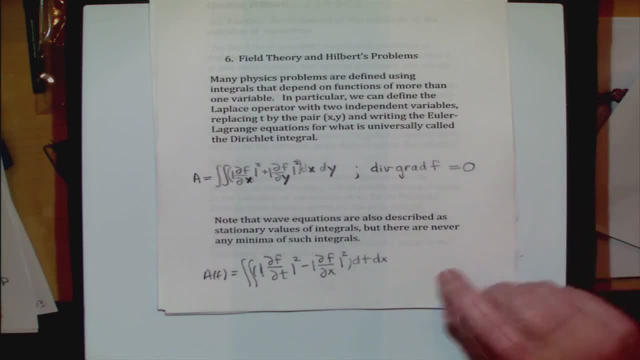 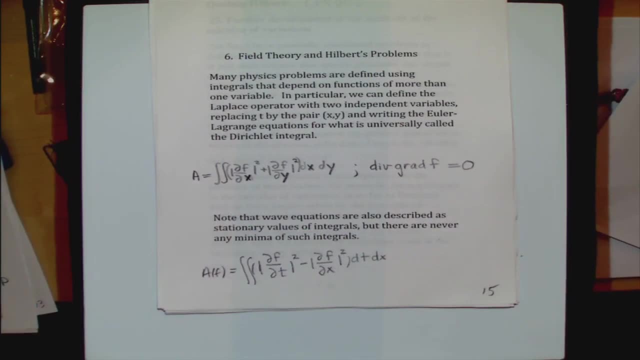 T by X and Y now And we write the. This is the action integral which is naturally, It's really just the norm squared of the gradient integrated over a region. And if we actually do Look at the Euler-Lagrange equations, 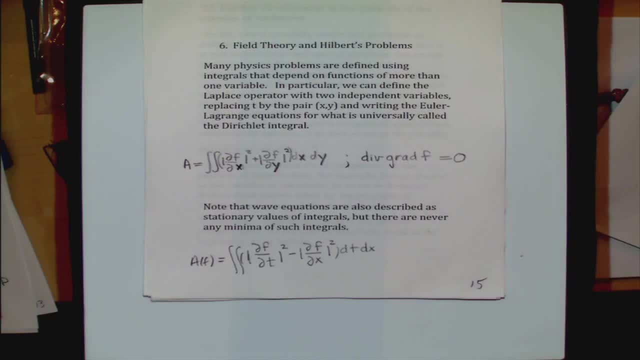 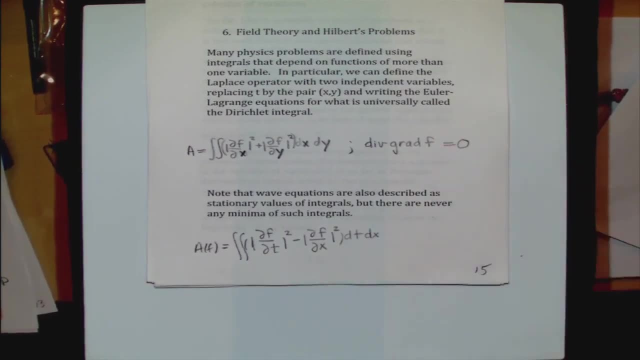 we get the Laplacian divergence of the gradient equals zero. So that's And the equations are also. Remember F is always the unknown in my problem- And notice that wave equations are also described this way And this is actually considered. 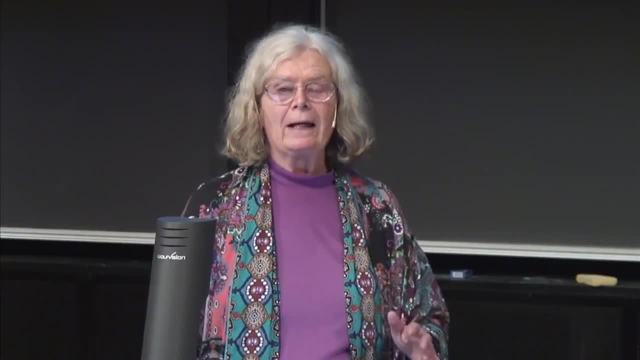 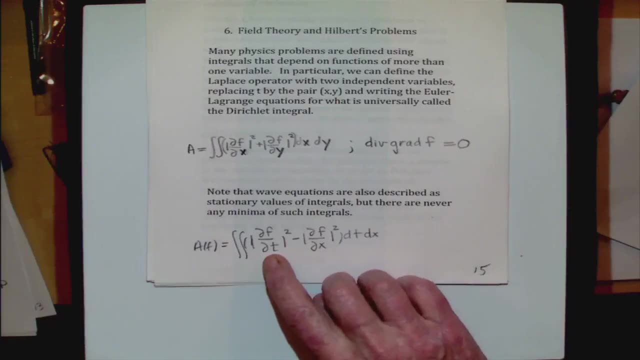 an important fact in physics, but there's no way you ever find a minimum for a wave equation. I mean, you have the, You can't. You can't find a minimum and you can't find a maximum. You can find a stationary equation. 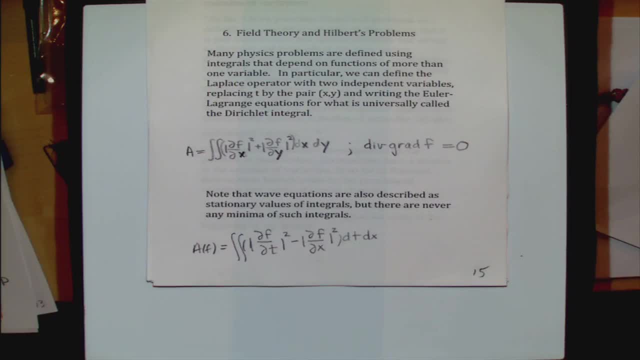 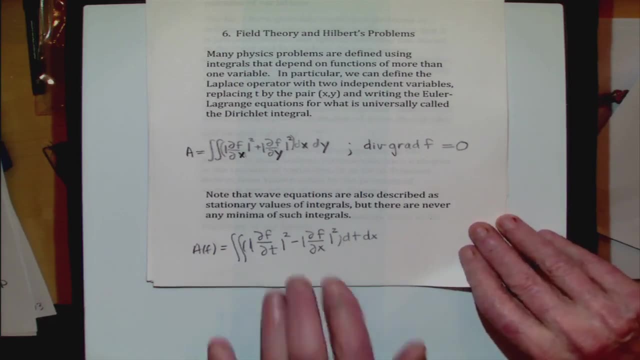 stationary F because the stationary, If it solves the wave equation, the usual wave equation in X and T, it's a stationary point for this, but it's not a minimum. Okay, So it is. This is I am talking about. 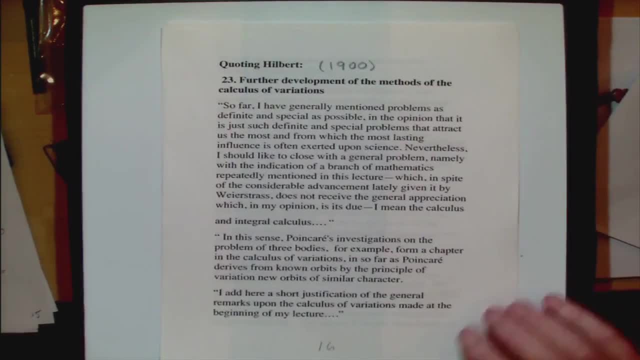 one of Hilbert's problems. Okay, Hilbert was At the 1900. Listed- a famous set of problems. This is his last problem And it's unlike. I've written it out. I don't want to. I don't want to go into it. 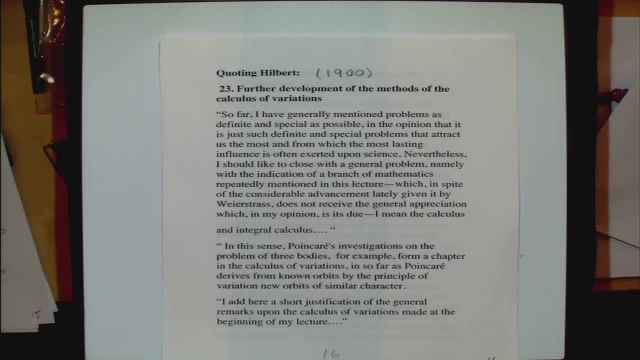 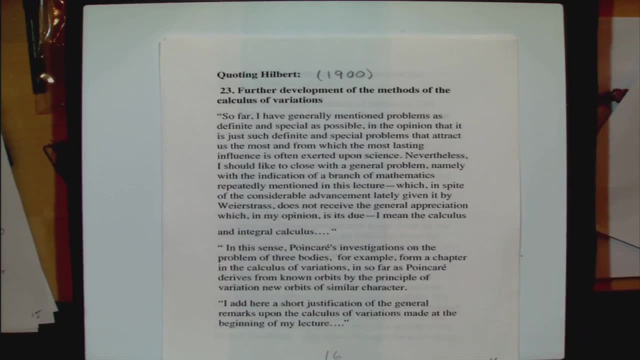 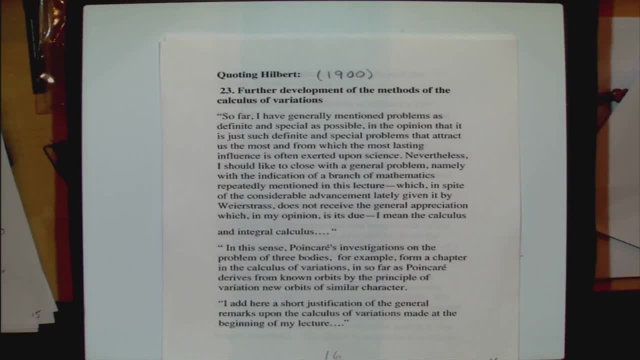 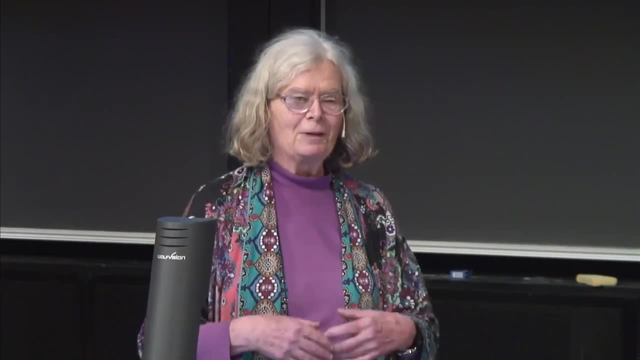 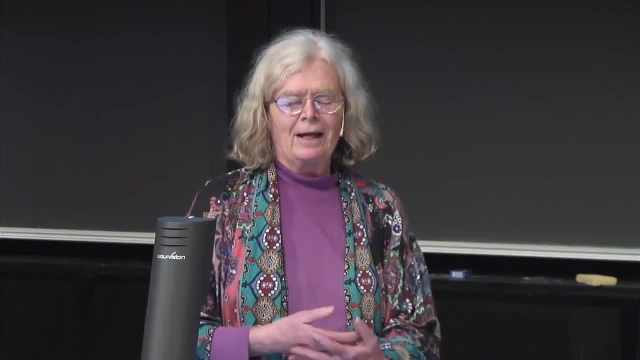 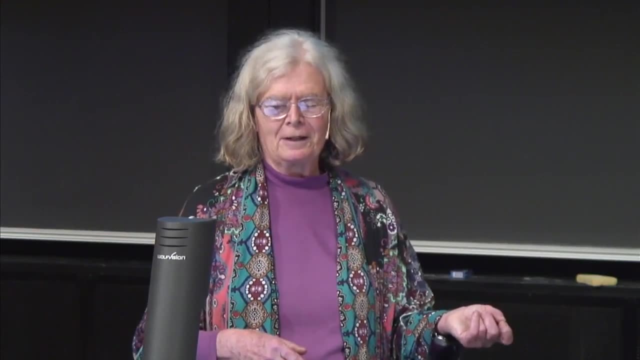 with two independent variables, And I should, I should. I throw in here at the point that there is this guy from Verstrasse, from From the 19th End of the 19th century, who actually showed that a lot of things. 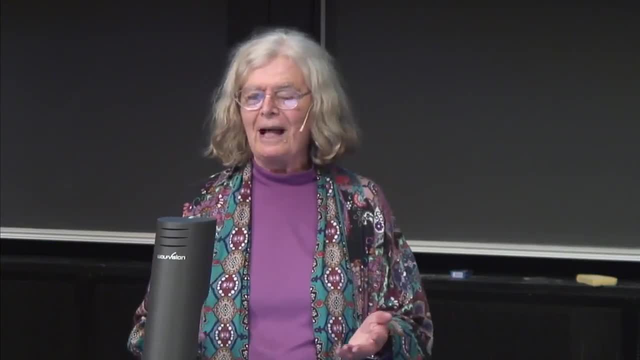 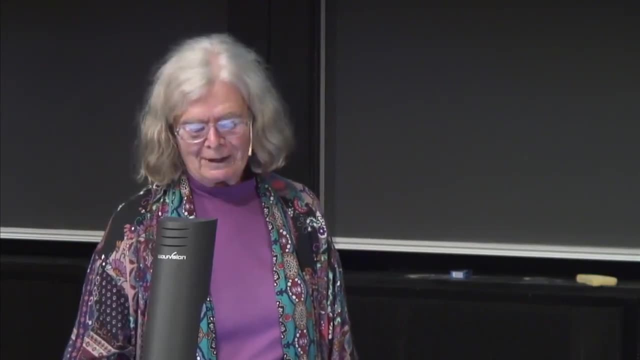 that mathematicians can do inред Cheer can do at that level is a più importante for people putting aside assumed were true, like you could find a minimum- just weren't true, And so they knew at this point that there were a real lot of problems. 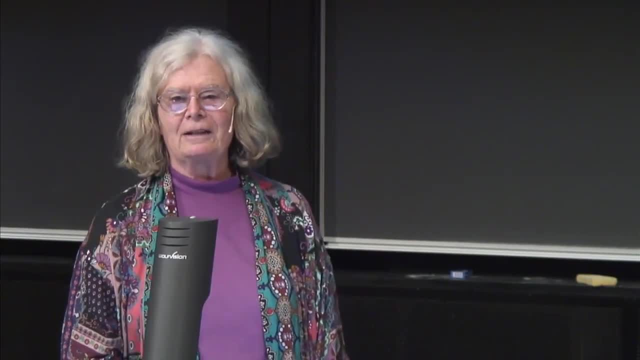 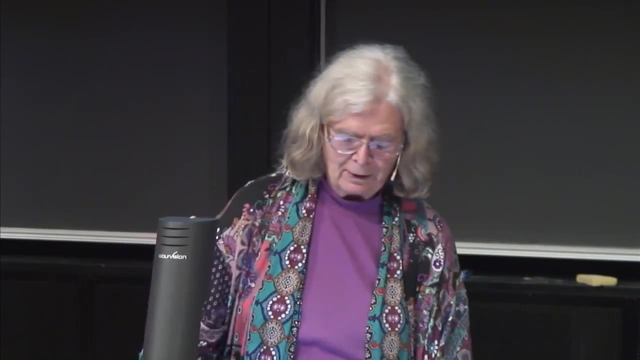 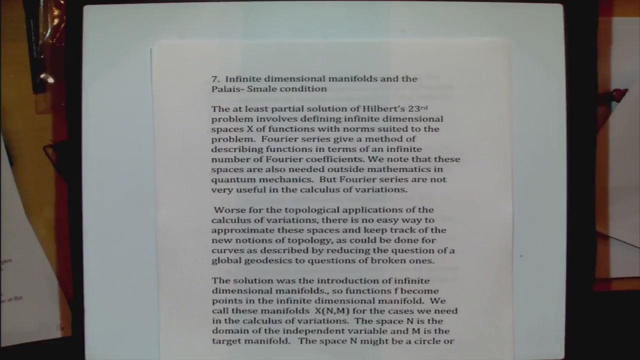 And it took most of the 20th century to actually shed any clarity on this question. So we're coming down to my life in mathematics, okay, And that's what I've called the section I've called Infinite Dimensional Manifolds and the Palli-Smale Condition. 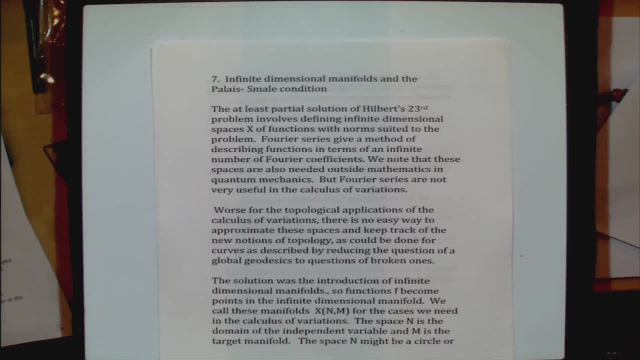 And so at least the partial solution- or in the early part of the 20th century was a partial solution- of Hilbert's problem, And it involves introducing function spaces. Now function spaces are putting norms on spaces and functions. So Fourier series give you a method of that. 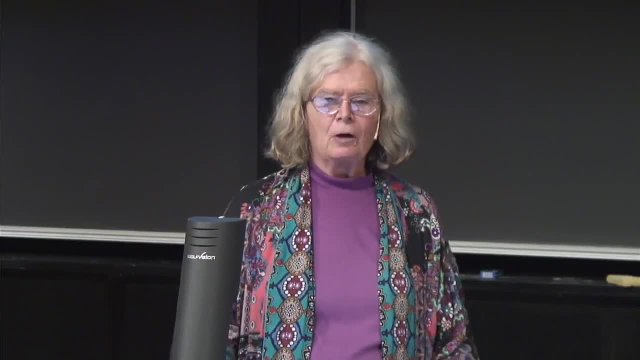 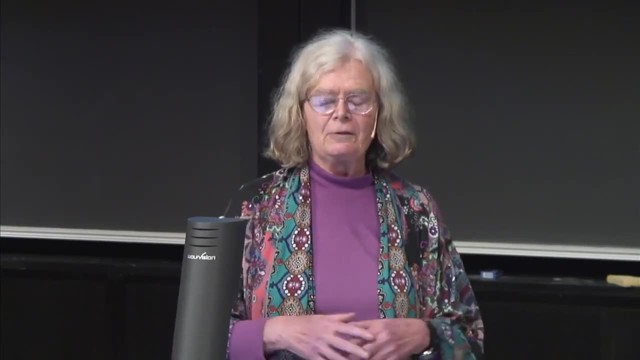 You have a function and you take its Fourier series, then you notice it has an infinite number of coefficients And you can think of those coefficients as coordinates describing the function. So you can either- This is very important in quantum mechanics- that you can think of a function. 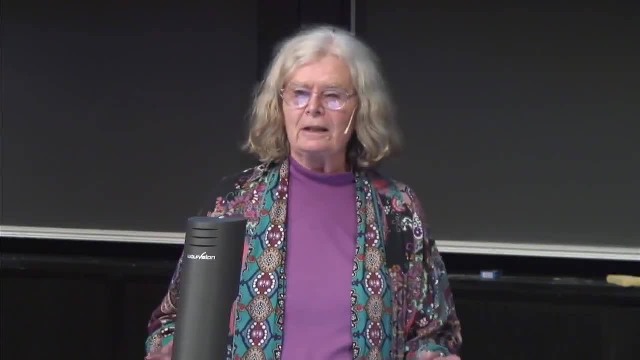 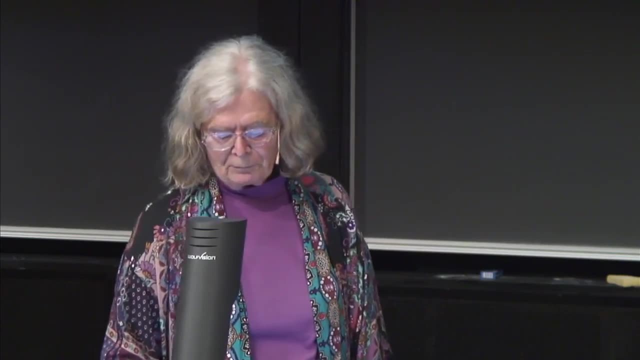 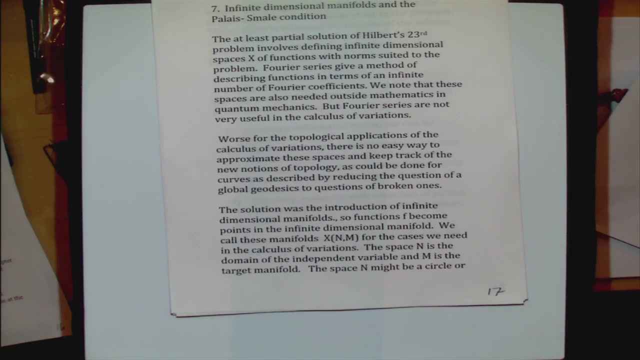 as being an infinite number of variables. Unfortunately, Fourier series are not a good way to go about solving calculus of variations problem. So, and for the topological applications, the real problem was to do the functions of one variable. We approximated it by a finite dimensional set. 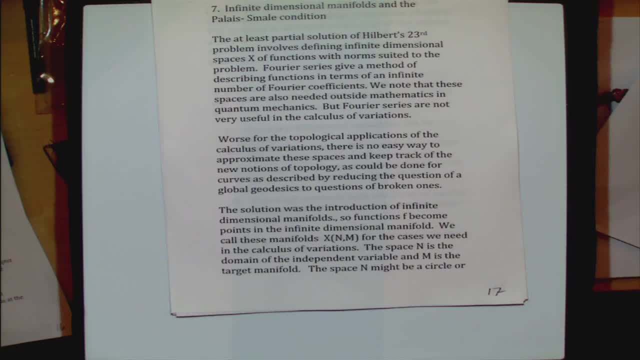 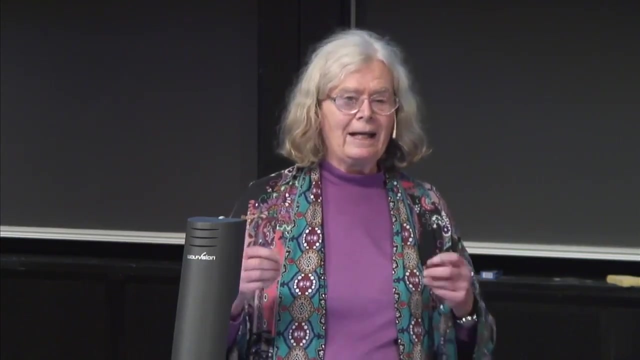 a finite number of points that sat in a manifold, And that was so. we were actually approximating the problem by a finite dimensional problem, And from calculus that was developed during the 19th century, one knew how to handle the problem, And so we were able to do that. 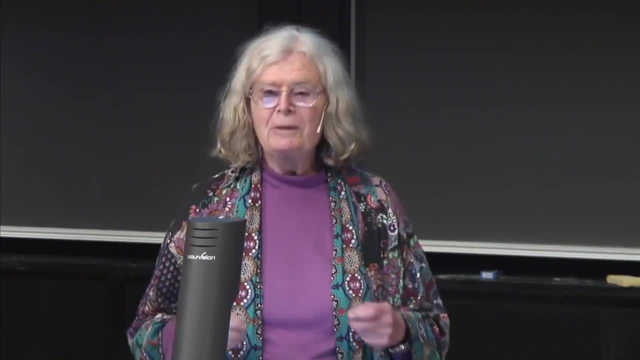 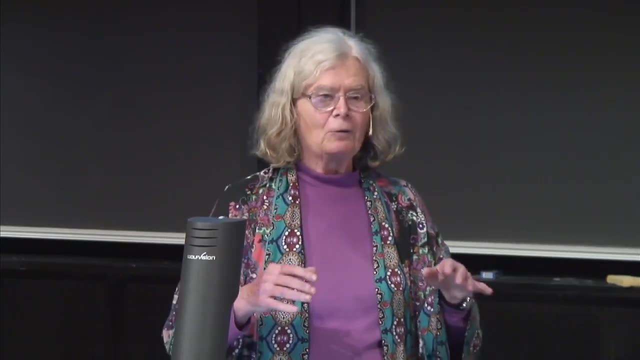 And so we were able to handle these problems of a finite number of variables. But they really tried, They really tried, They took. You have a function on a plane and you're trying to figure out a way to approximate it, And so how are you going to do this? 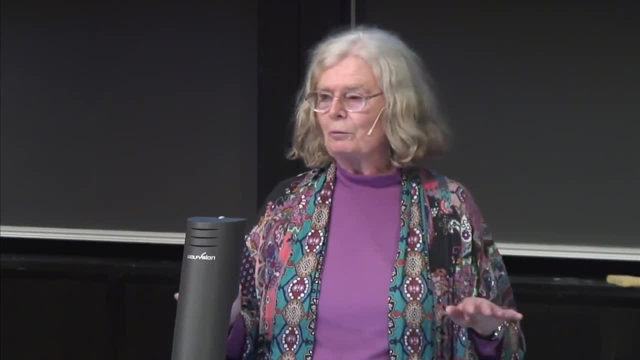 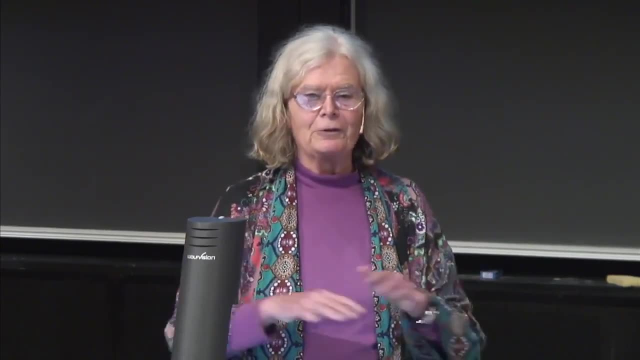 Well, in fact, of course, with computers we do it real easy. We just put a whole bunch of points on it and we take a lot of difference quotients and we actually approximate all the derivatives by difference quotients and so forth. 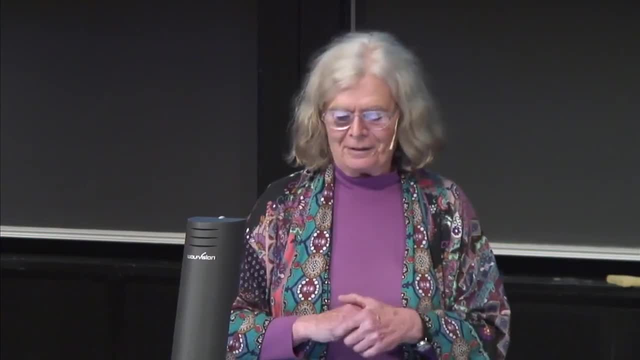 But they didn't have. They didn't have a lot of difference quotients, So they had a lot of difference quotients, So they had a lot of difference quantitions And they were able to do this with computers And the And also sort of for rigorous mathematics. 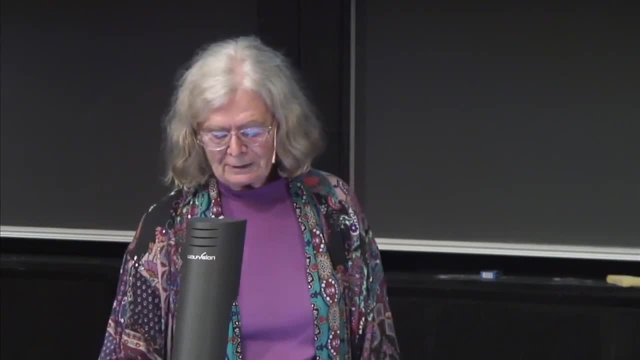 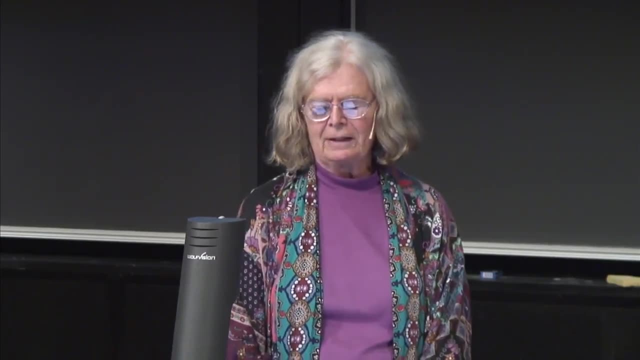 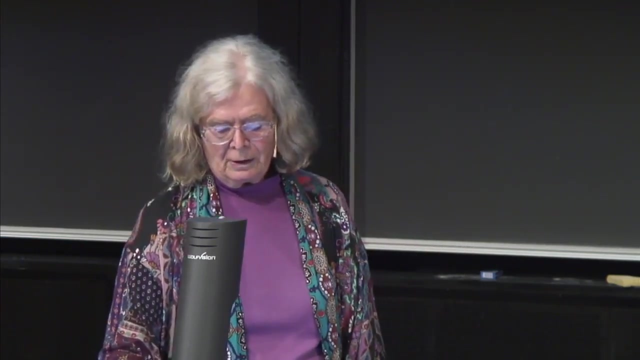 it's not. it's a little bit hard to take that approach, But so the the solution that was discovered in the early part of the 20th century was is that we use these function spaces. So now we come to the question of how do we solve that problem. 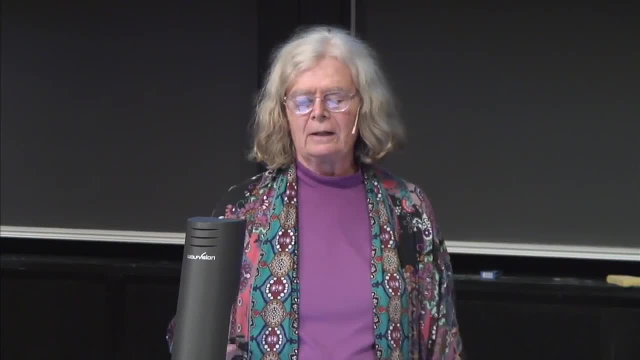 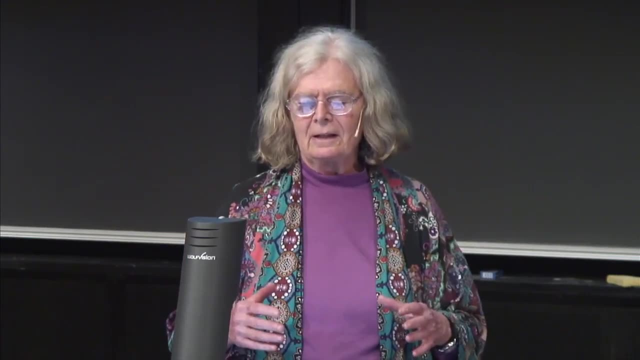 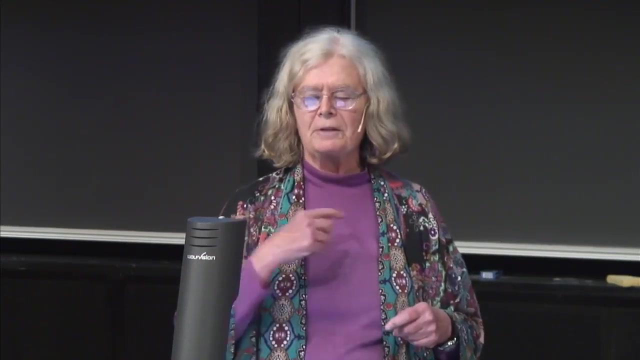 question of how we treat problems like the geodesic problem. I mean a typical example, if you really want to, is that, of course, the typical example that's easiest to explain is the plateau problem, which is you have a curve in free space and you want to put a minimal surface. 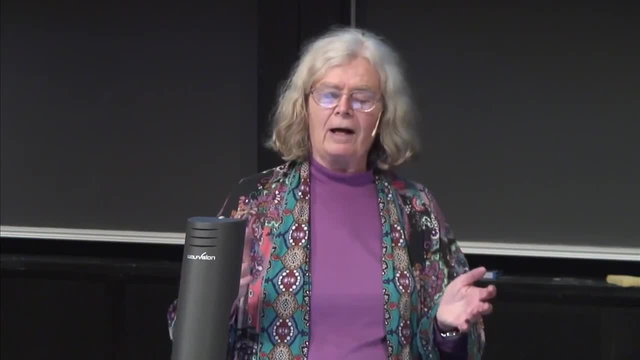 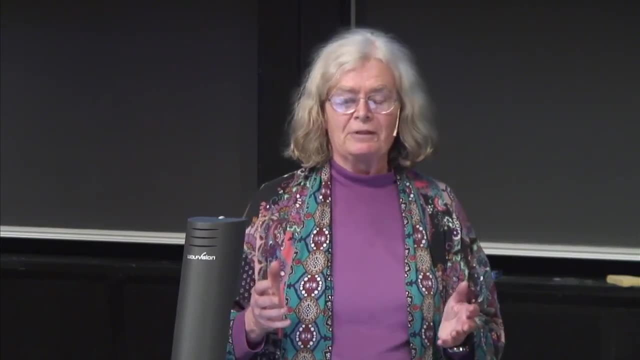 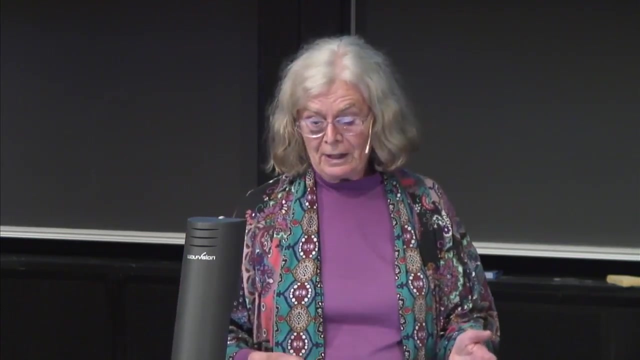 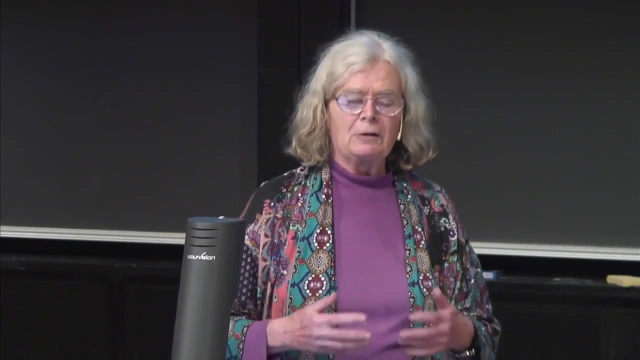 area surface in it. But if you have a curved space, if it's curved, then the problem with even setting up the problem becomes difficult because you don't really have the right tools And it turned out. so what the solution? that actually of solving these geometric calculus? 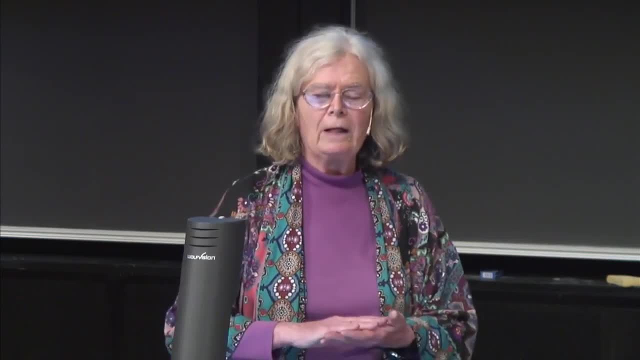 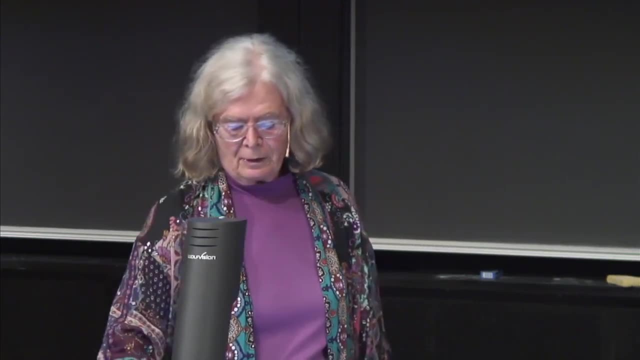 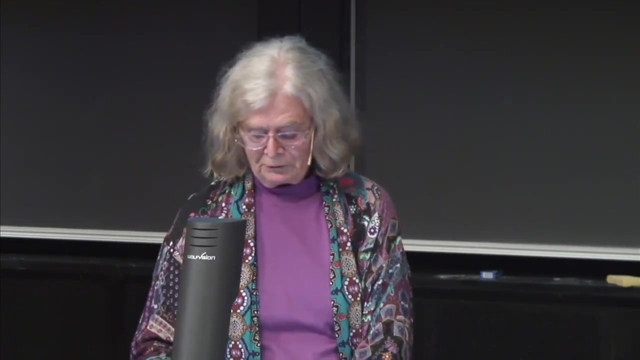 problem- calculus of variations, problem with more than one independent variable- was to introduce infinite dimensional manifolds. And this was done in mostly in the 60s- I think- I'm not when I was a student, you see. So we introduced infinite dimensional 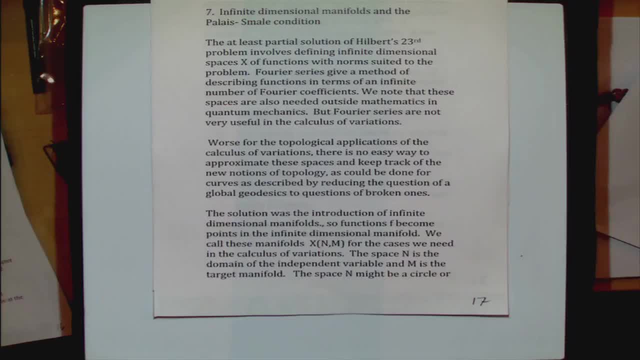 manifolds and I'm calling these manifolds, I'm calling the space. x is your function space. Now, the function x is a Hilbert space, or a Hilbert space with, or a functions with, one derivative in a Hilbert space, or it's the space of c. 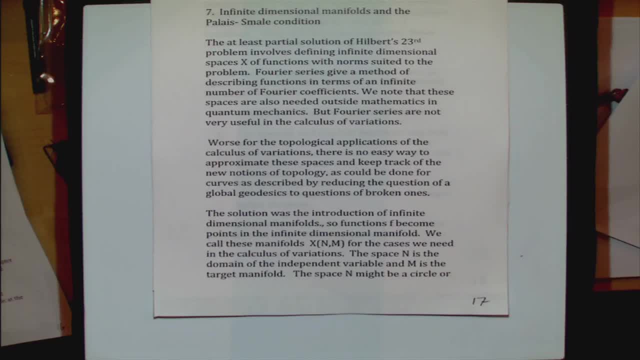 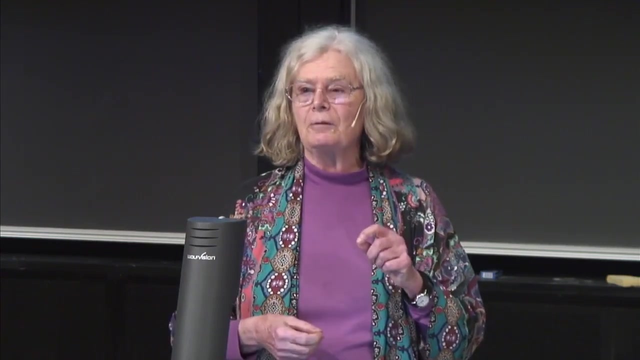 In other words, say the space is in the right space, then the space of the left space is in the right space, and that's followed by a function space, that's followed by a function space. And you can, you can. you can do infinite differences. You can do infinite things like: 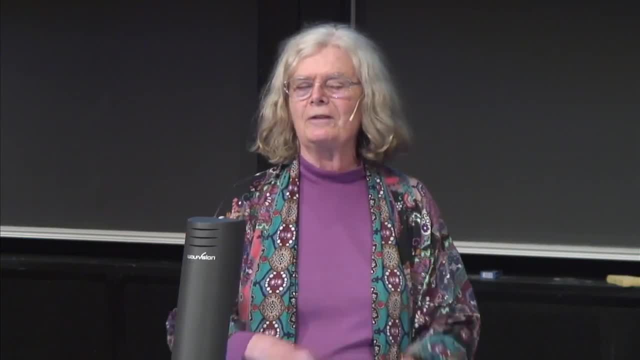 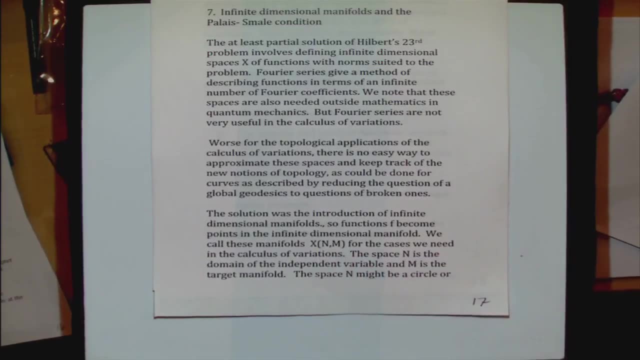 Aussie infinity functions, or there are many different kinds of spaces. you can actually. I mean, there are so many different kinds of spaces, they have different norms on them, They're all. And so there are two manifolds involved. One is the manifold that you start with. 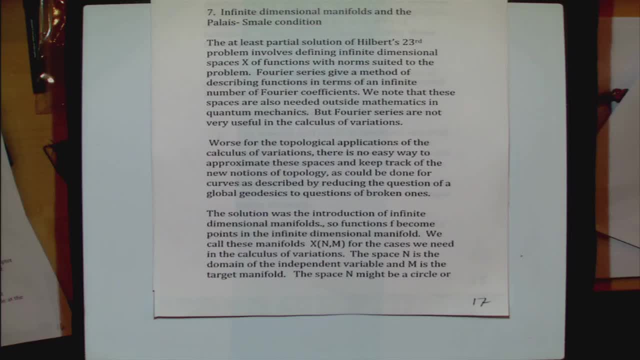 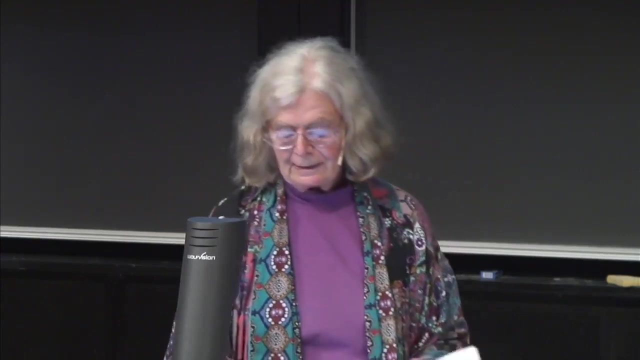 We can actually really think of starting with a two-dimensional plane for the easiest case, And we want to map it and we want to look at the space of functions that go from a plane into a curved space, And it is the dimension of n that's important, okay. 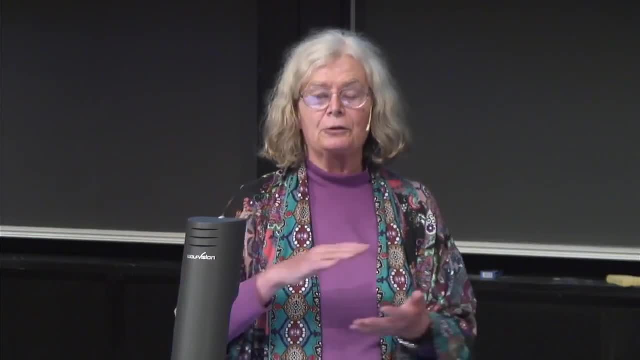 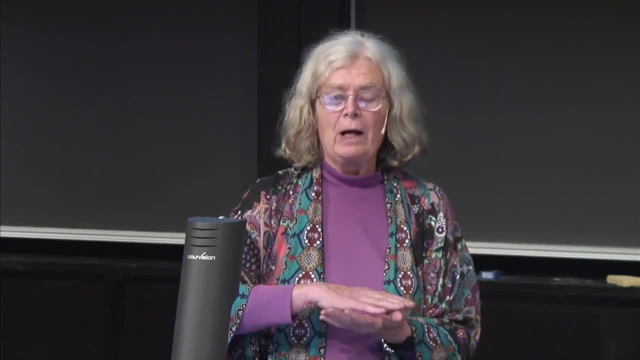 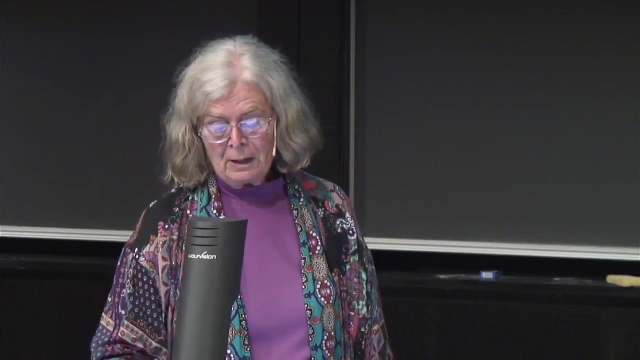 Remember, we couldn't go from one independent variable to two independent variables with the classical notions, So we couldn't go from one to two without actually changing the way we did things, And in two dimensions. it's the dimension of n which is important. 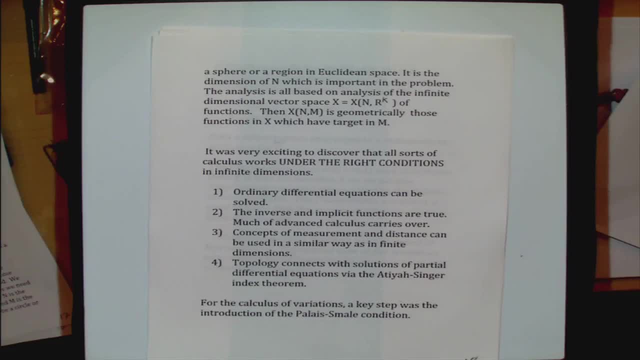 And all the analysis is based on the linear analysis in the function space of maps from your, say, two-dimensional object into into a Euclidean space, which is a linear space which you understand, And you also have people that you can go and ask questions to about them. 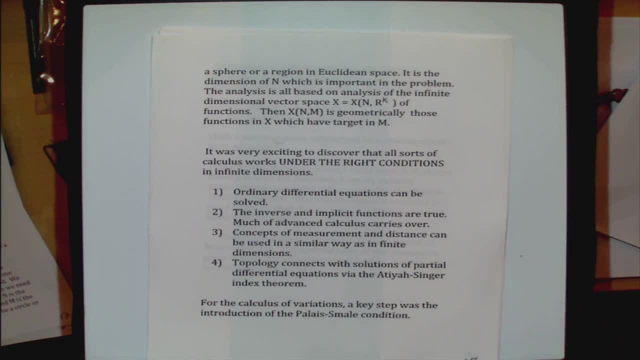 And so what the manifold is is, geometrically, the space, is the space of, It's the space of functions in the linear vector space, of maps into Euclidean space that actually sit in time, And that's why the manifold. We're using the Nash Embedding Theorem again. 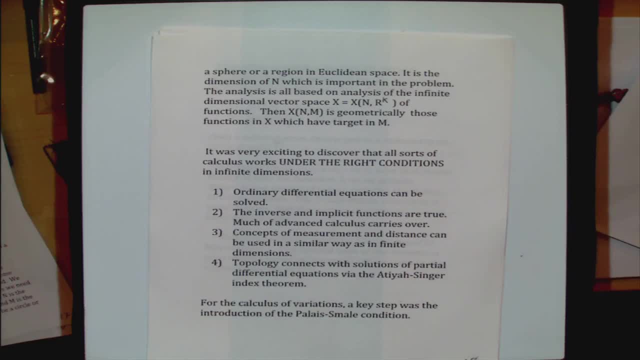 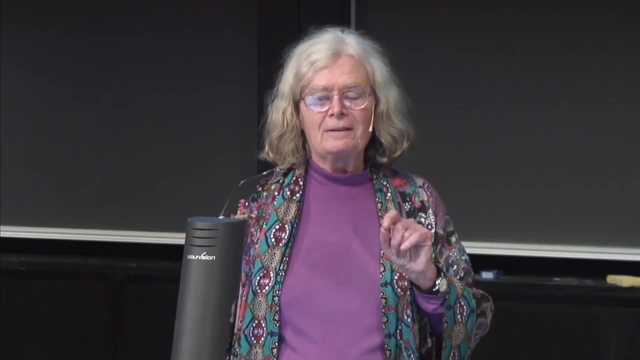 I mean that's. You know, the Nash Embedding Theorem is not absolutely essential. You can do it without the Nash Embedding Theorem, but it simplifies. It simplifies like pages of work to use it, So it's. 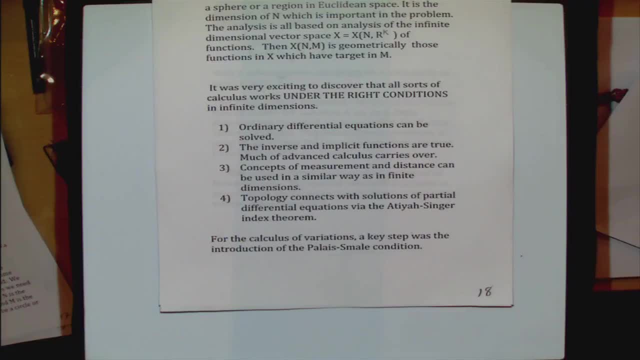 So it was very exciting to discover that calculus works under all the right conditions. okay, You could actually do calculus in infinite dimensions. Now you think- And you know people are really Kind of: How do you think about infinite dimensions? 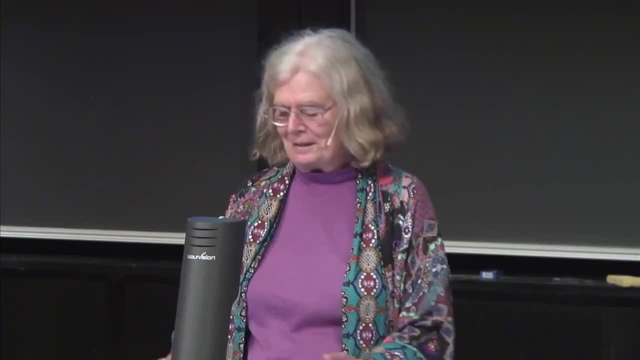 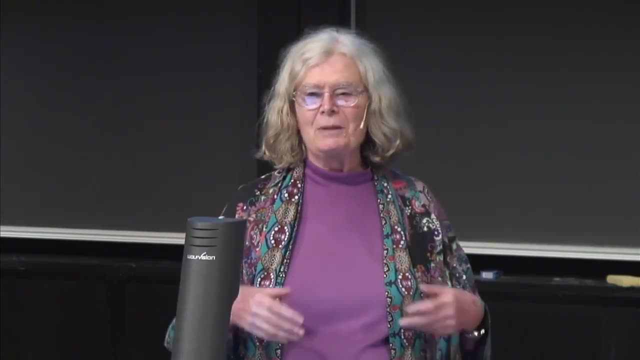 Well, functions are infinite dimensions. So you have to think about functions and then you know. So what you discover about infinite dimensions is that ordinary differential equations can be solved. You use the same proof, I mean, as you do in your ordinary differential equations. 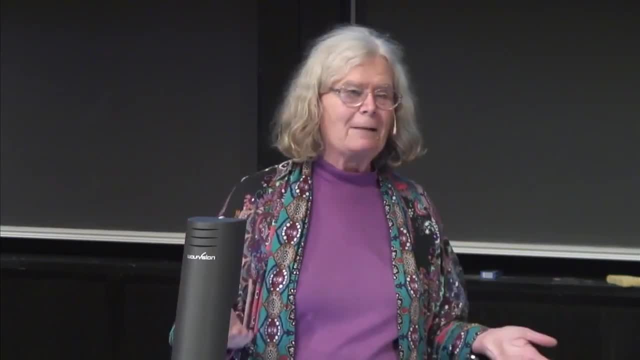 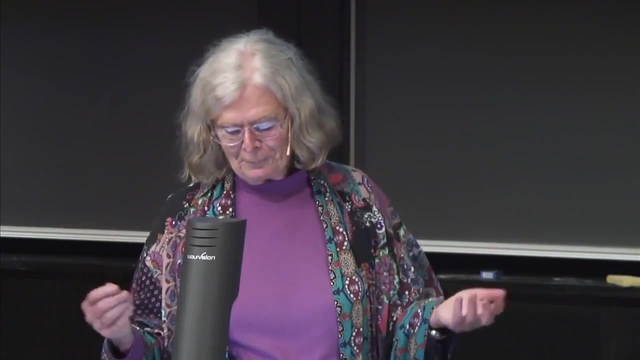 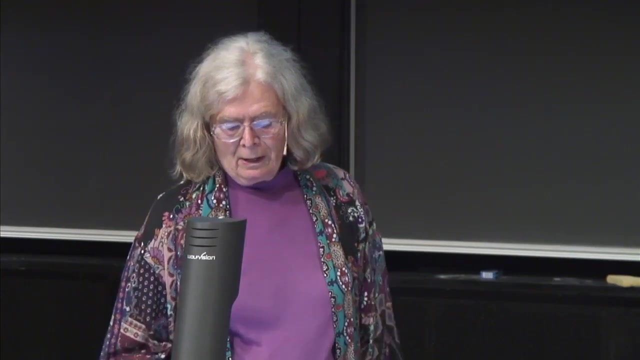 The inverse function theorems are true. Not only that, the same proof works. You have norms and distances and so forth, and you do it in two dimensions and you can do it in infinite dimensions, And you can also set up concepts of measuring distance. 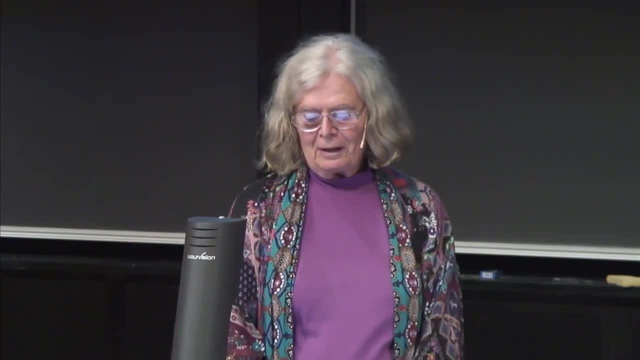 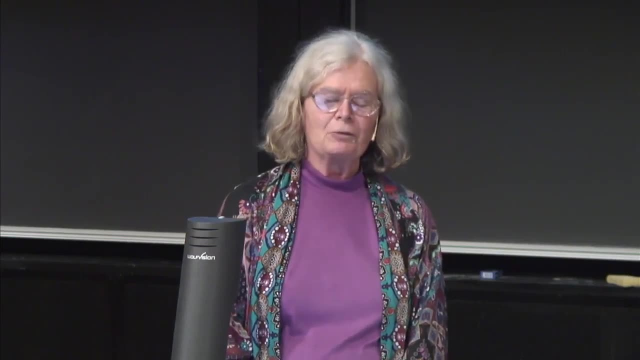 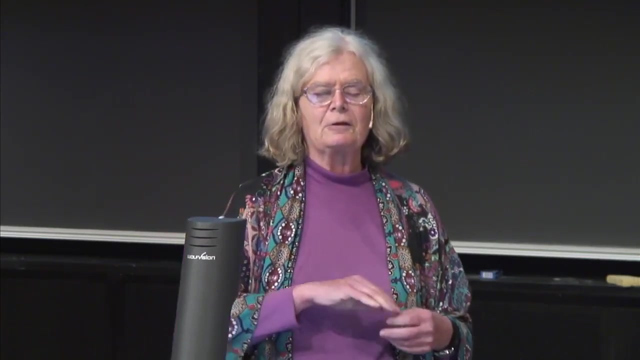 And I also mentioned. I noticed that Also there was sort of an indication that this was a really interesting area of endeavour because the Attia-Singer Index Theorem could connect the dimensions of spaces of solutions with the topology of the manifolds you were working on. 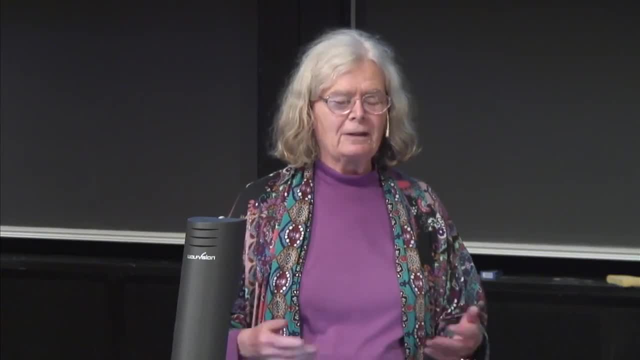 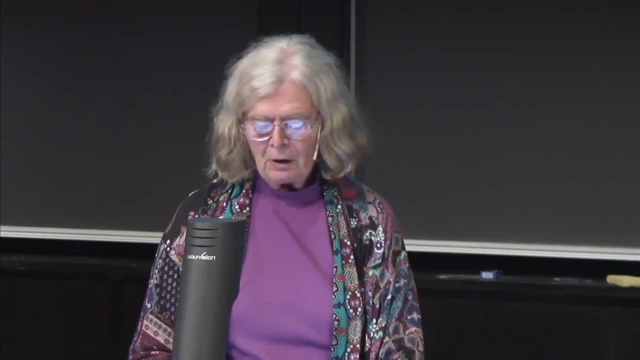 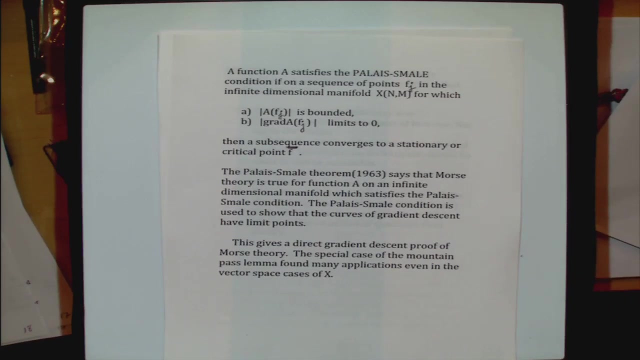 So it was a clue that there was something really interesting going on. I mentioned Attia and Singer. both have Abl prices, So So for the calculus of variations, the important thing is the Palais-Mille condition. OK, And the Palais-Mille condition. 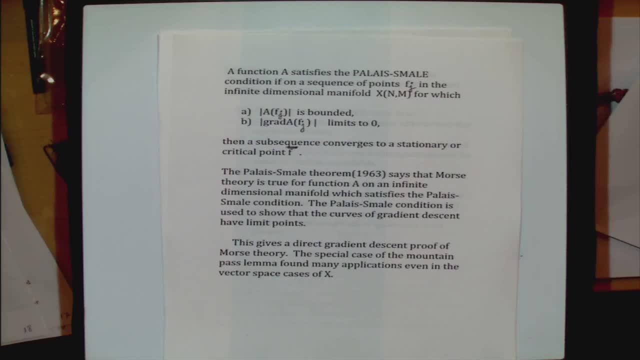 basically is a condition that says if we have a bound on the function, Remember our action. integral is what we're trying to find out something about, We're trying to minimise it, or we're trying to actually find a saddle point or something, And so we have. 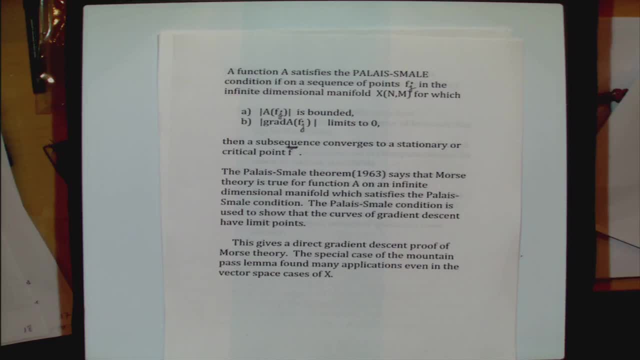 The size of A is bounded, but the gradient when we compute it, And we have a sequence of points on which A is bounded and we have a sequence of points along which the derivative goes to zero. So we're actually following a gradient curve. 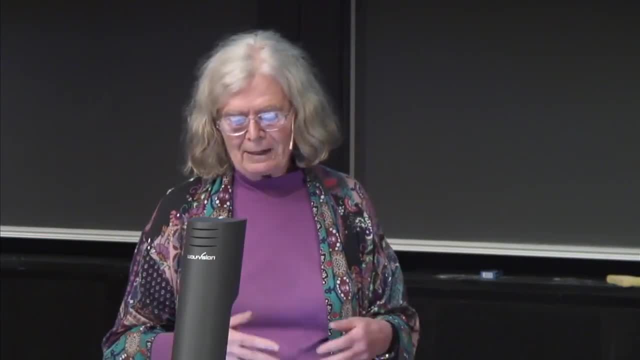 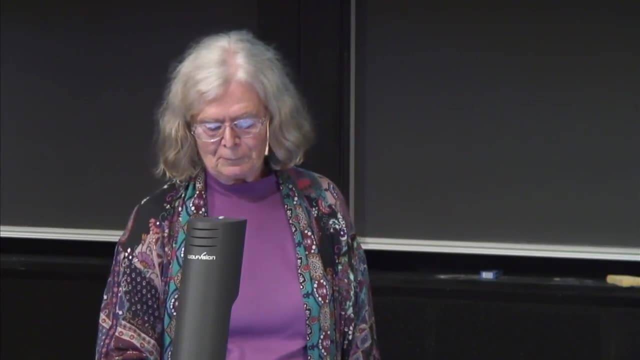 and we're trying to figure out where the gradient curve goes And the Palais-Mille condition is a condition that says It's a condition. You have to say the functional satisfies, the Palais-Mille condition, And it's used to show that curves of gradient descent. 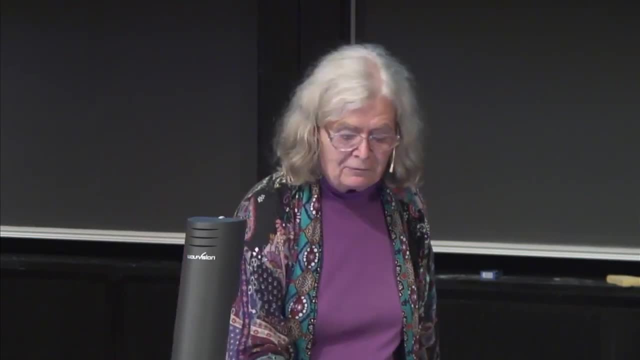 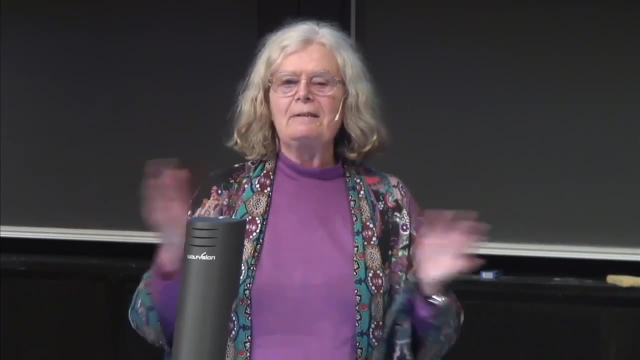 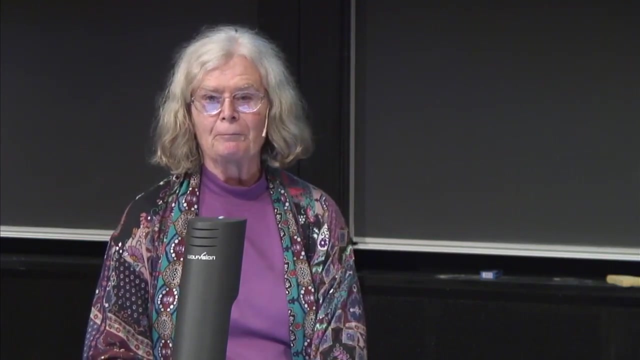 have limit points, OK. So in fact this found a lot of applications to the mountain pass lemma. It gives an easy proof of Morse theory for the geodesics and it gives very many applications of the mountain pass theorem. So 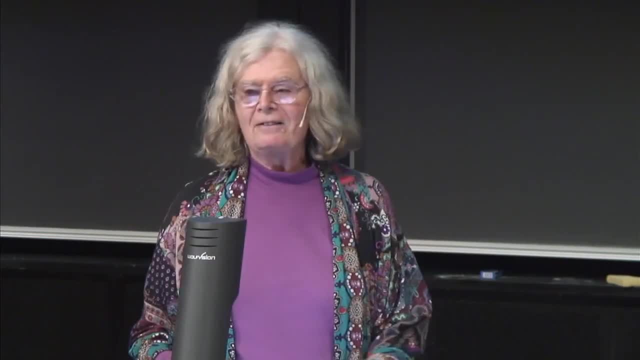 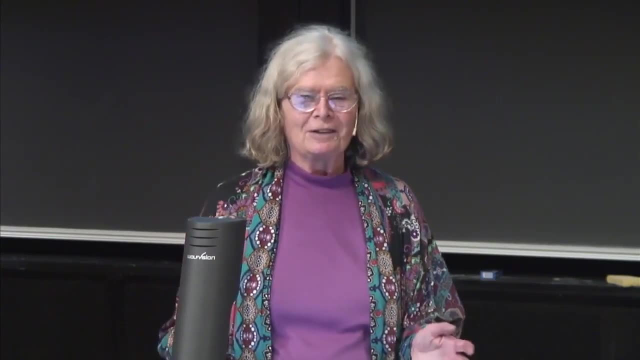 So, in fact, however, it's interesting that it was not accepted as being a very exciting thing. It was way overblown. We didn't really. It didn't really do everything it promised to. This was a new subject, a whole new idea. 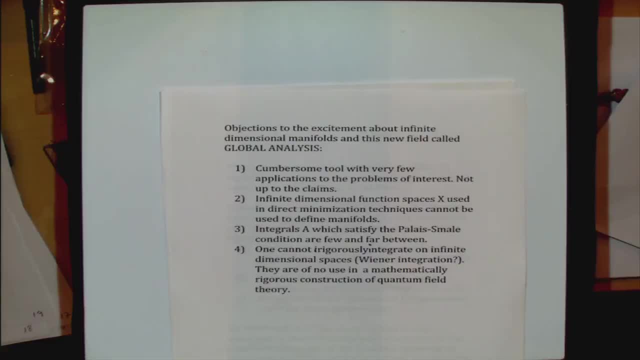 a whole new way of approaching things, but it wasn't all that great And I think it's really interesting you make that point. It isn't when something happens that's useful, that everybody jumps on the bus. I mean, there's always these people saying: 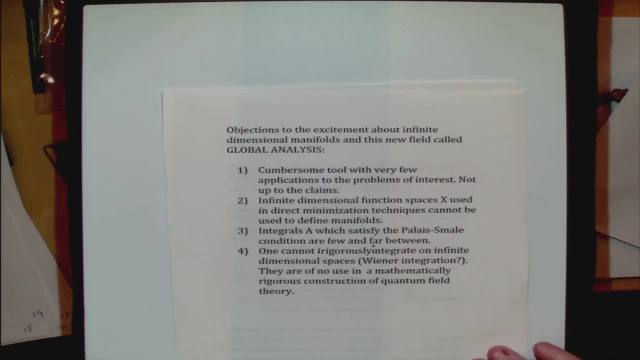 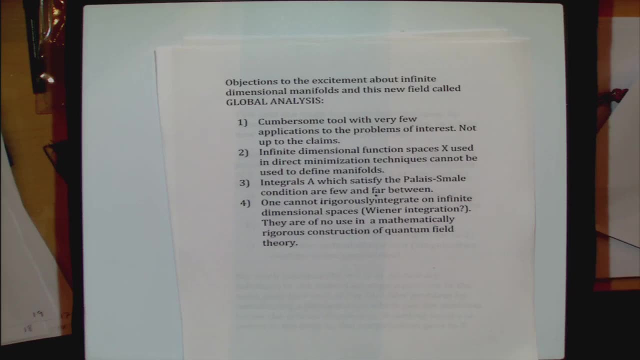 Oh no, You do it the old way. We don't want to do it this way. So I also want to point out that the one that bothers me the most is that you can't integrate in infinite dimensions, And so you can't do quantum field theory. 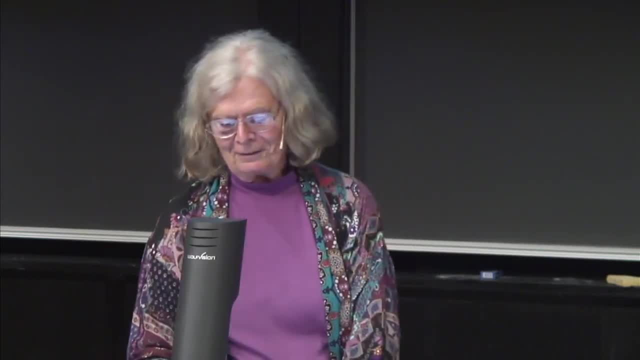 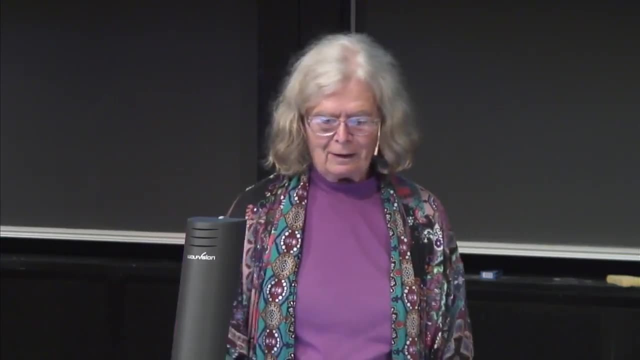 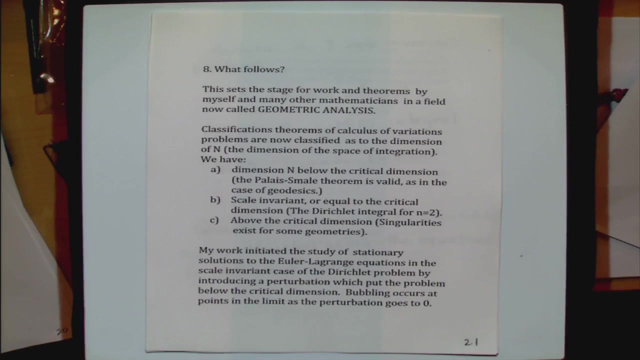 as rigorously in mathematics at all, And that bugs me the most. but OK, So this gives a quick. I'm running out of time, But this is really what sets the stage for the work of theorem for myself and current theorems. 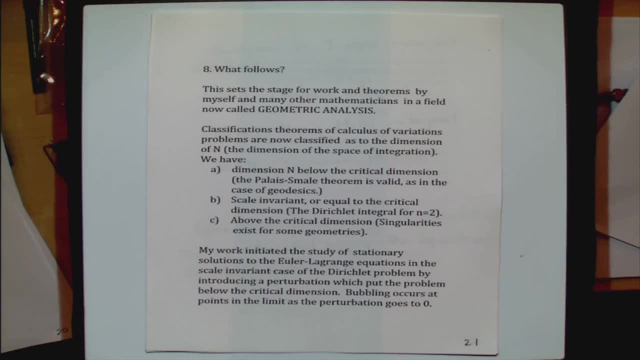 and the calculus of variations in the lab, And I think it's really important that we think about this in the context of the last 40 years, which has been the time period with that And what We now have: a classification problem that we usually have a set of problems. 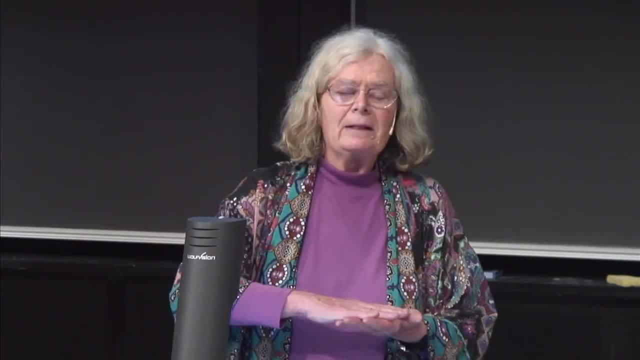 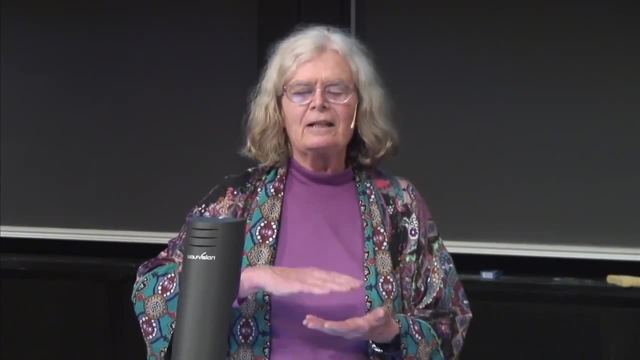 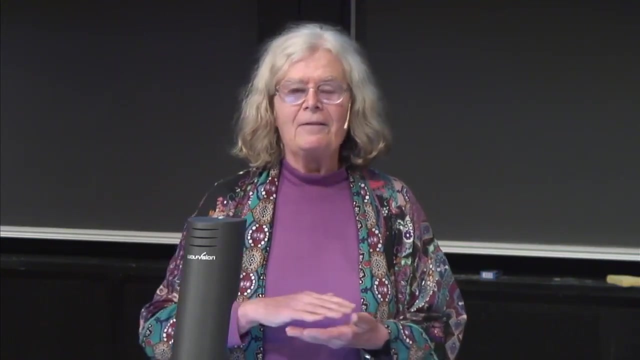 that we can define in any dimension, And the dimension always being the number of independent variables, And if the Pauli-Smil condition is true, is valid, or with other conditions it's a scale invariant problem, It's called borderline, And those are a lot of interesting problems. 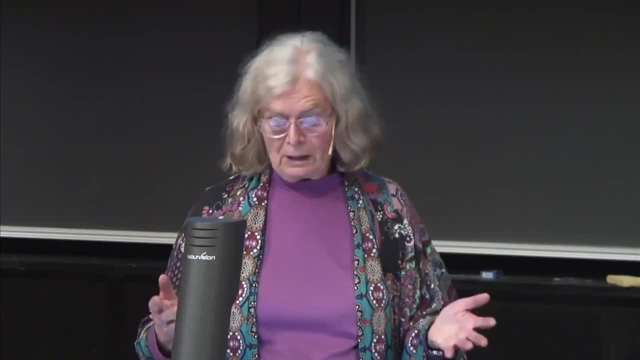 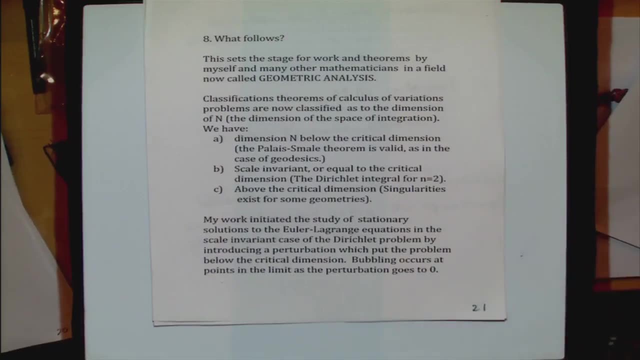 Minimal surfaces, Yang-Mills equations and so forth fall into that. And above the critical dimensions is singularity. Singularities always exist, So that answers Hilbert's problem. Forget that one. There's singularities and holes in the thing and it's a mess. 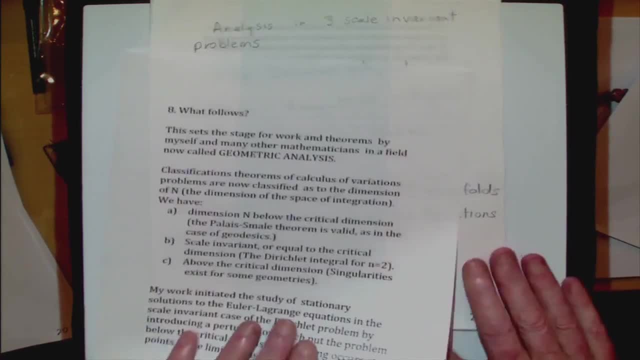 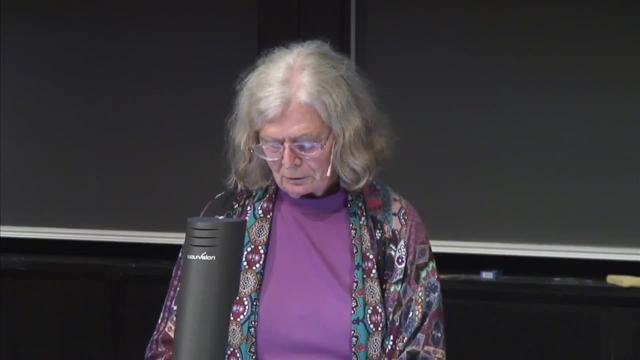 So we still study that. That's what we're looking at. We're looking at the singularities. OK Well, I want to stop this. Sorry, Oh, Oh, OK, Yeah, OK. So what follows? Oh? 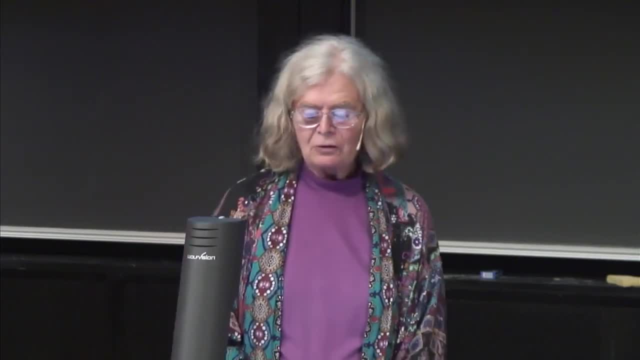 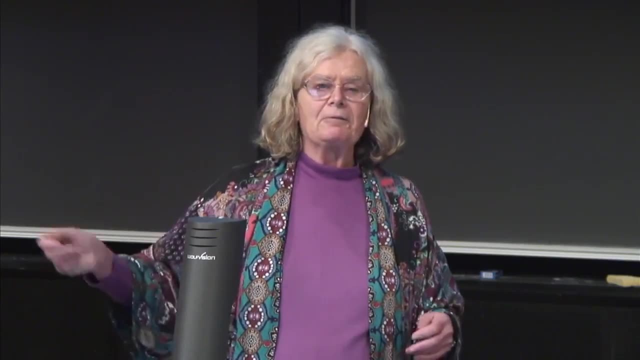 Yeah, And I should say something about. So actually I've actually studied. Most of the work I'm best known for is for the scale invariant case, And what you do is you add a little bit to the functional and it's Pauli-Smil. 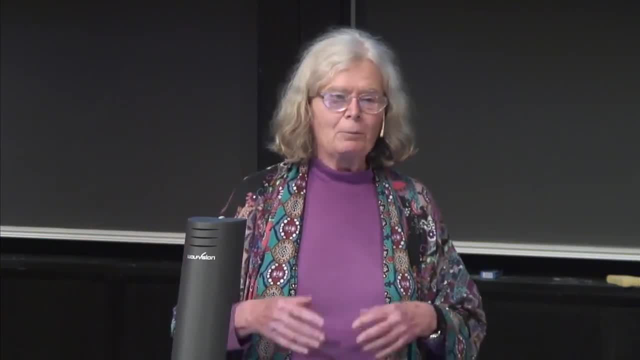 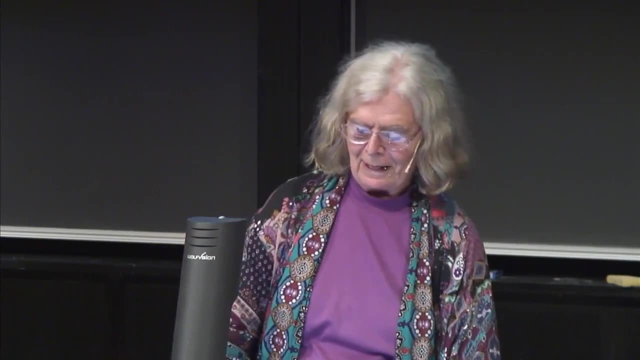 And then you take the little bit away and you see what happens And I think probably Robert Bryant's going to tell you a little bit about actually what happens in that case. So So I really want to get to the end. So what looks interesting. 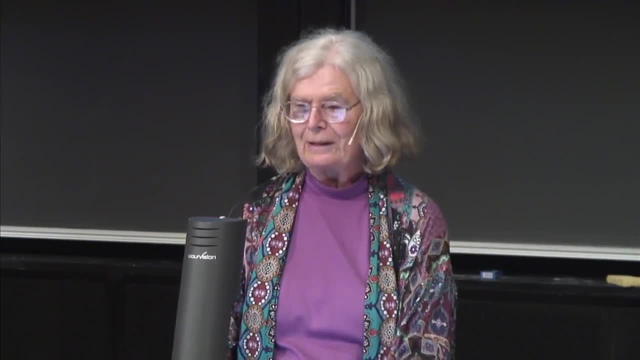 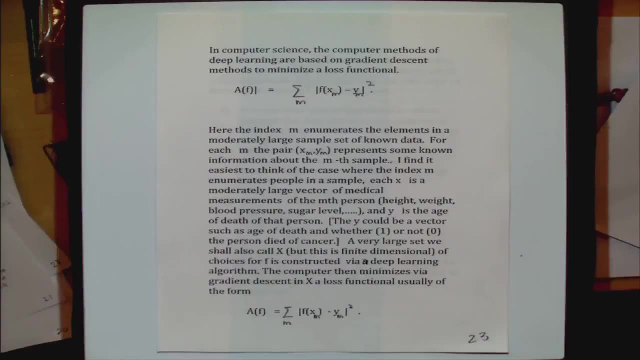 Well, you know, people keep on asking me what sort of math you could do, And the answer is: if I knew I'd be there. But anyway, I have to talk. I've heard so many talks on this. I have to mention it. 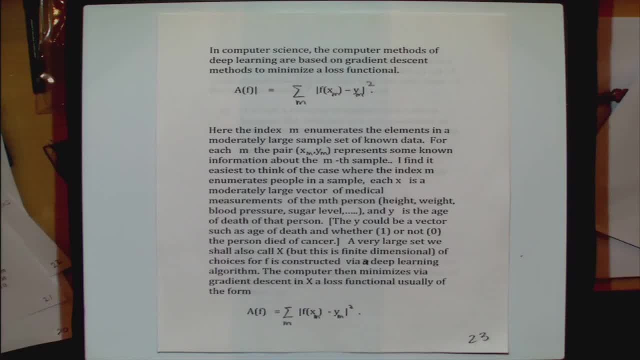 And this is the question of deep learning in computer science And computer. So computer, This is really hot, I mean, And It's not hot in mathematics, but it's hot in computer science, and you can easily hear a talk. 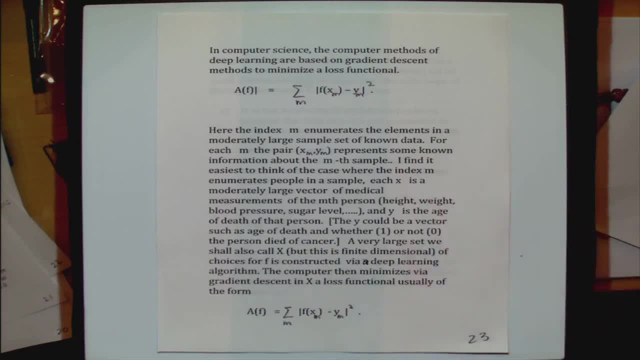 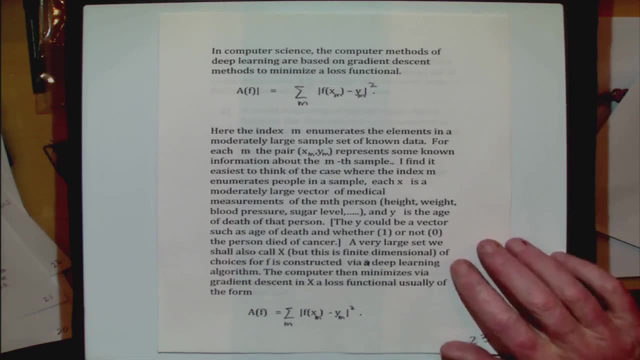 Here we have Our F now is a. Our unknown is the Well there's. First of all, we have a finite number of a sample, And you should think of the sample as being a whole bunch of people I don't like to use. 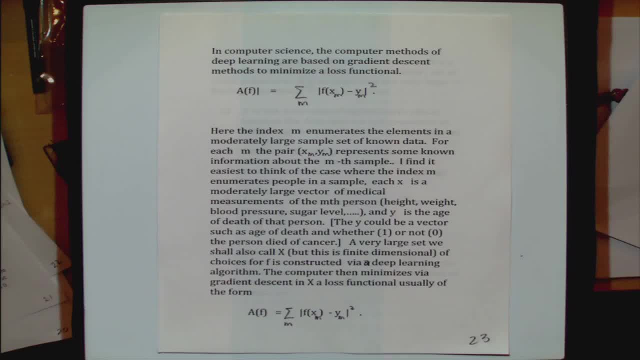 They use pictures, but that's I mean photographs. but that's not good because you're thinking space there, Don't think space. A whole bunch of samples, like a list of people and their medical records of you know what they measured and so forth. 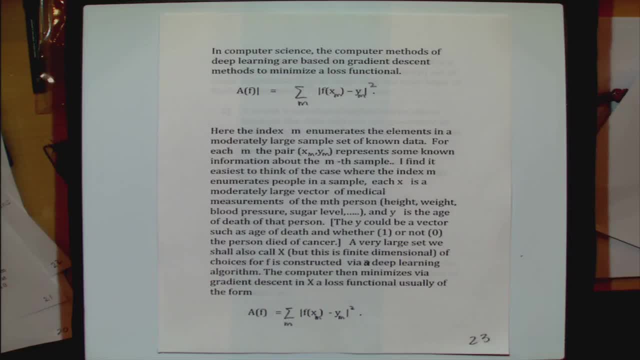 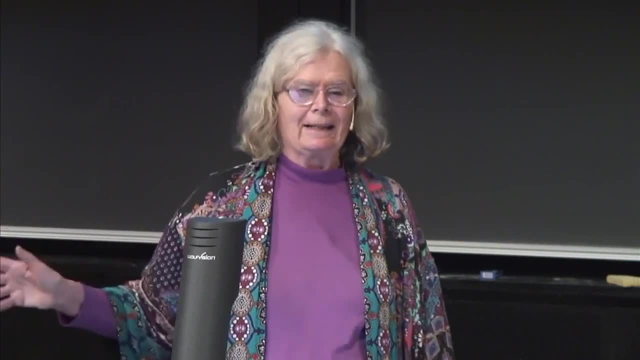 And then you say You look at some outcome and that's: when did they die? It could be two things: When did they die, and did they die of cancer or not or something like that. It could be ten things, but it's usually only a small number. 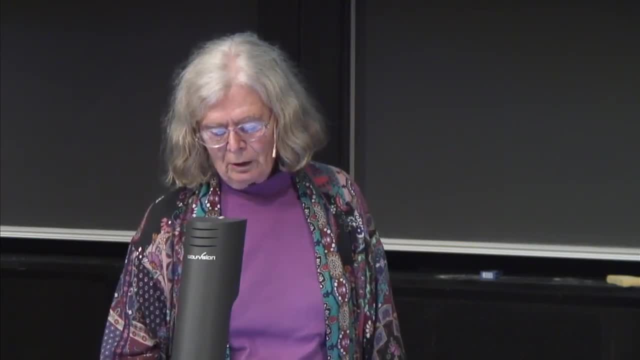 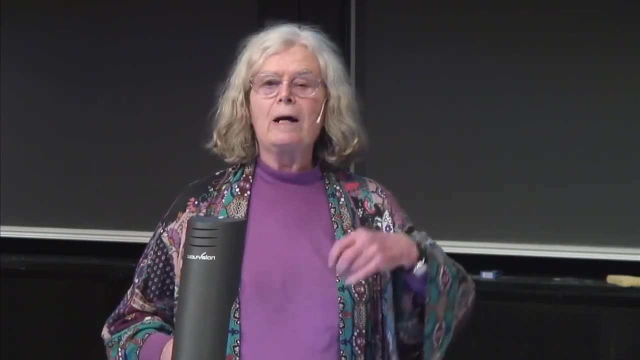 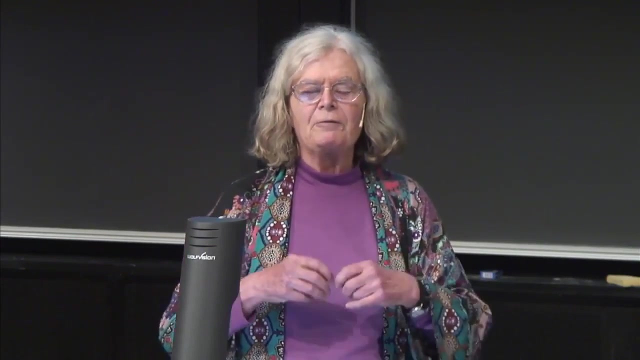 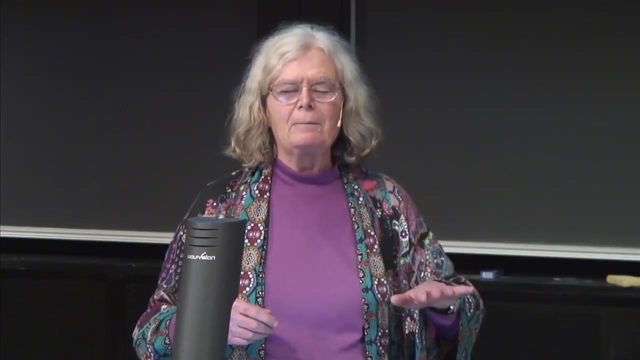 And so the way it goes about is that you have this sample and now you want to predict somebody not in the sample. So what's done is the deep learning involves a very complicated method of constructing possible maps from elements in the sample to the outcomes. 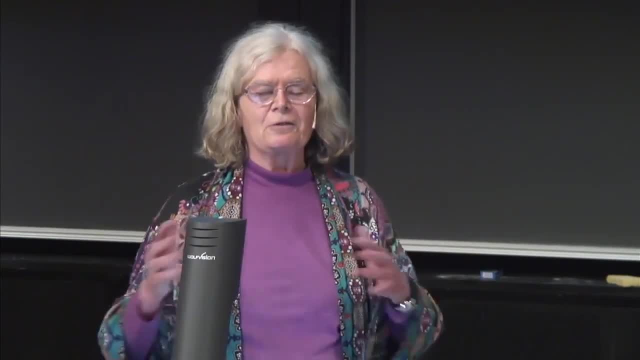 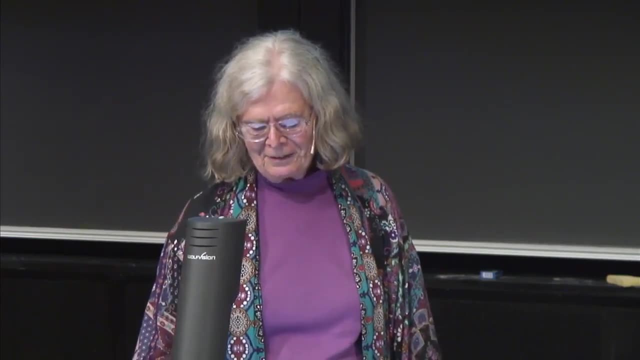 And that's the deep part of it. It's very complicated, and the computer scientists will tell you all about it to an extent, But what we want to do is understanding what they're doing, And so this It's a very large set. 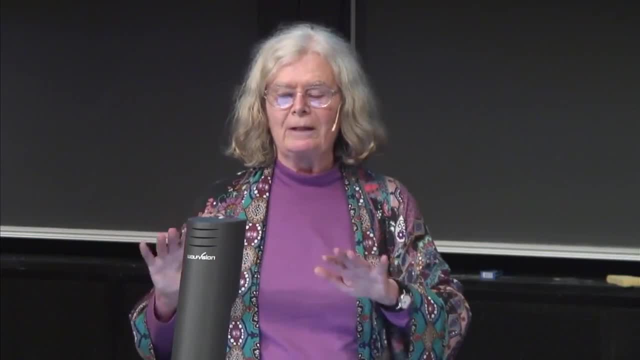 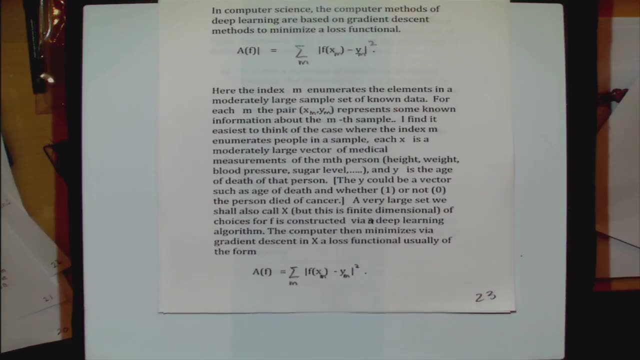 but it's a finite dimensional one and it's very important, And how it's constructed is very important and it's finite dimension And the problem is to minimize a loss. functional, which is our A again, But now this is still a calculus problem. 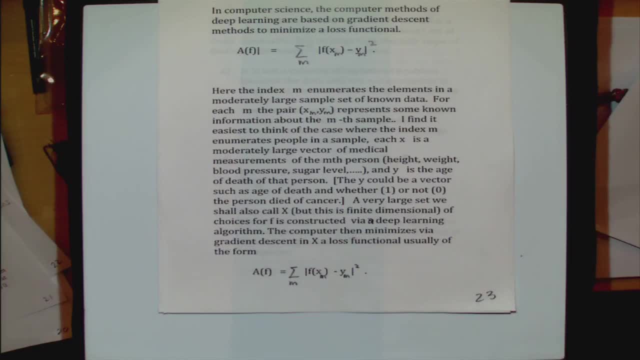 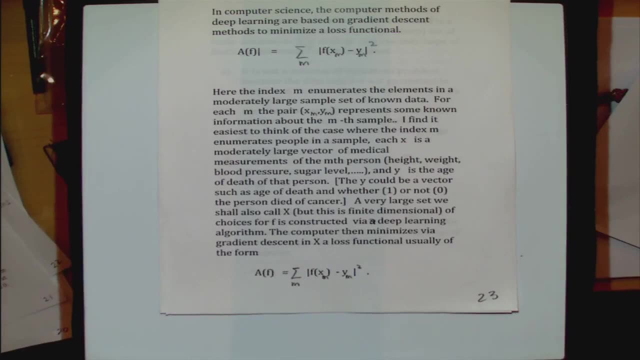 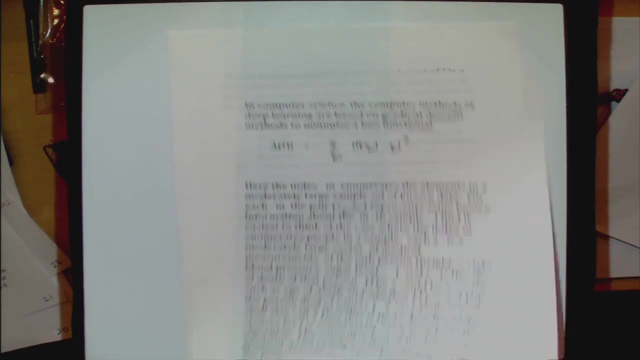 because we're in finite. We only have a finite, It's F that's finite. We only have a finite number of choices, of ways to go from the people's data to the outcome of whether they die. And it's a calculus problem because it's. 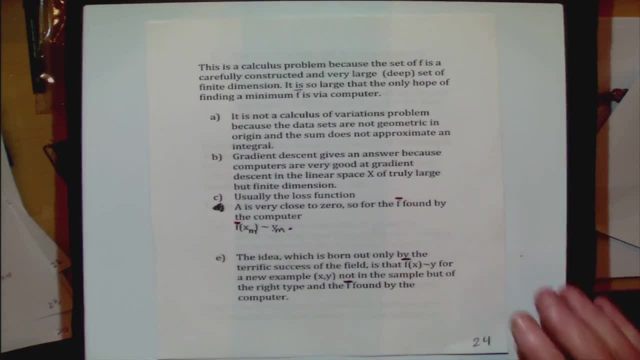 And so gradient descent, Gradient descent methods work. They work fantastically, They work beautifully. You put all this stuff on the computer and you tell it to find the best function, and it does. It gives you an F bar, and not only. There's a lot of interesting thing about this. 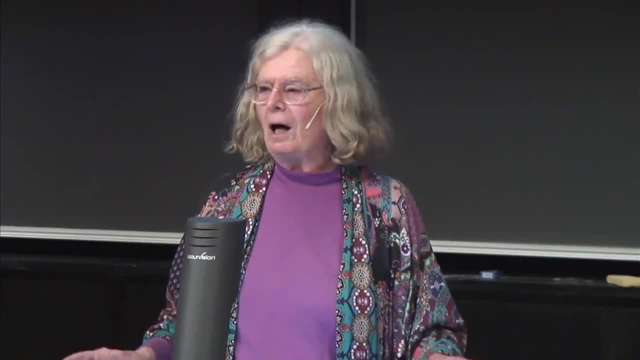 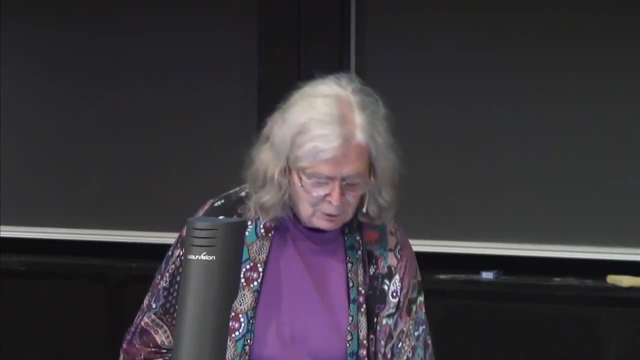 The trouble is is they don't really know what's going on. They're doing it and it's a magic kind of thing. It's not a calculus of variations problem, because there's a sum here which you like to make an integral, but there's no way to do it. 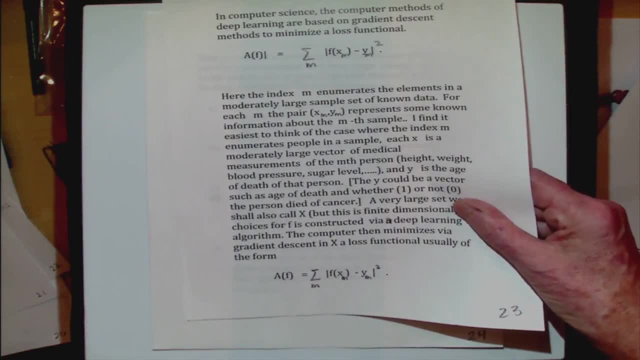 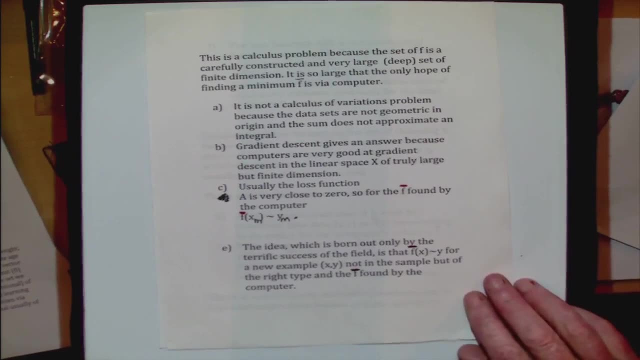 But there's no way. How are you going to get a DX in this? Where is that? It doesn't. It's not a calculus of variation and there's no integral involved, And gradient descent gives an answer, just because computers are great at that. 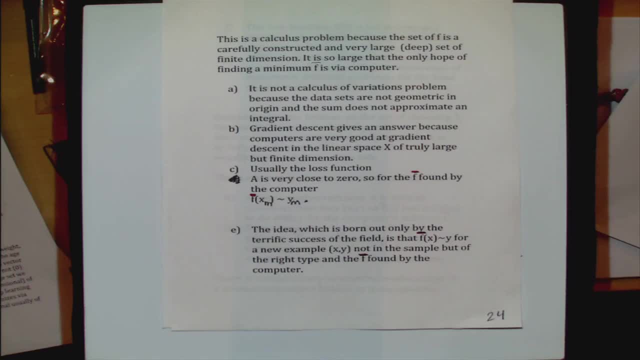 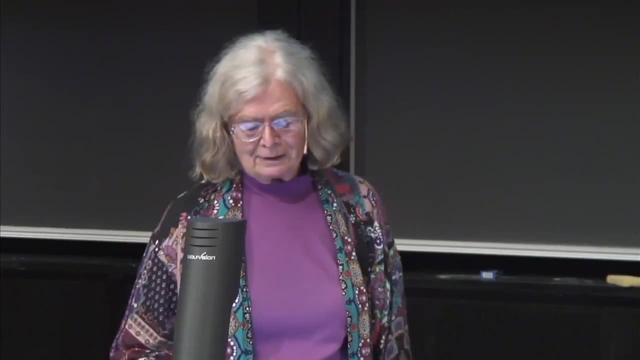 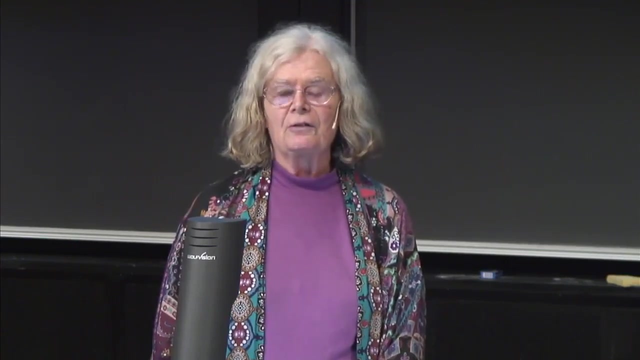 They've been doing that ever since computers were invented and they really know how to dig gradient. They don't know how to construct the functions. That space of functions is an art But And the actual facts? the loss function is usually very close to zero. 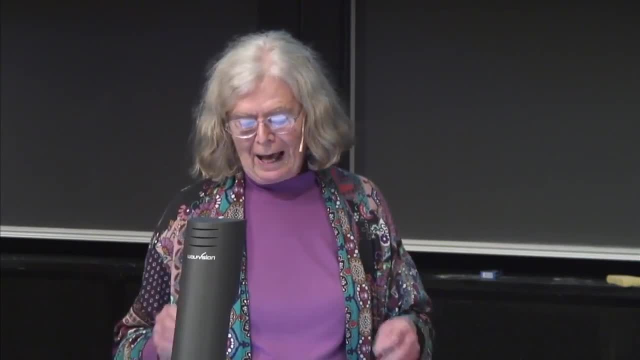 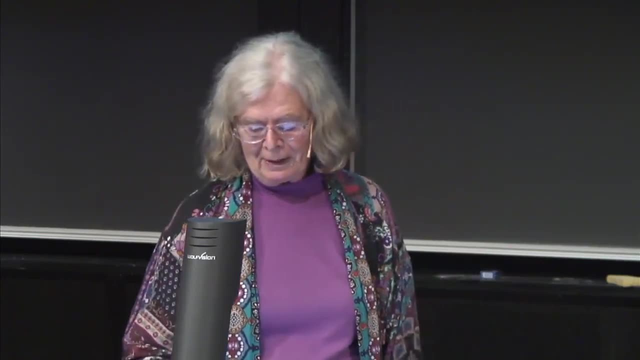 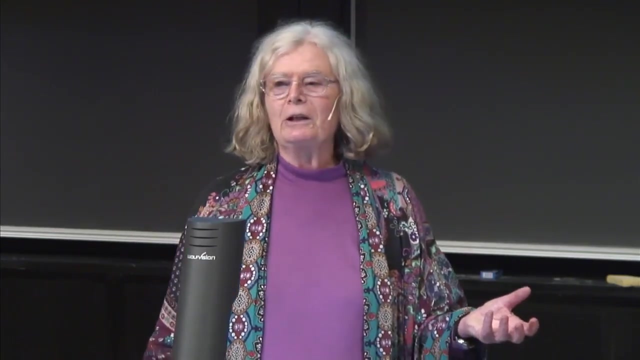 So, in fact, the F bar found by the computer actually gives the right answer for all the sample that you've got- pretty much So. So what happens? Well, then you go out and test your F bar and it's really good. 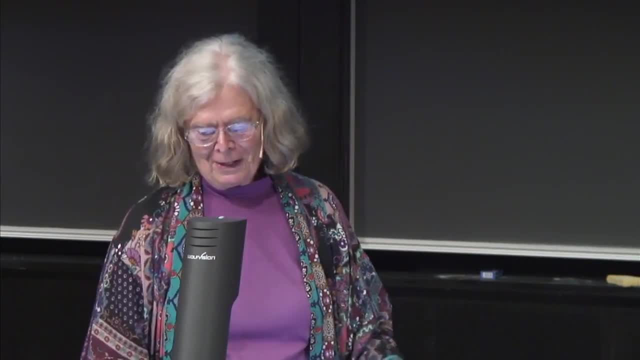 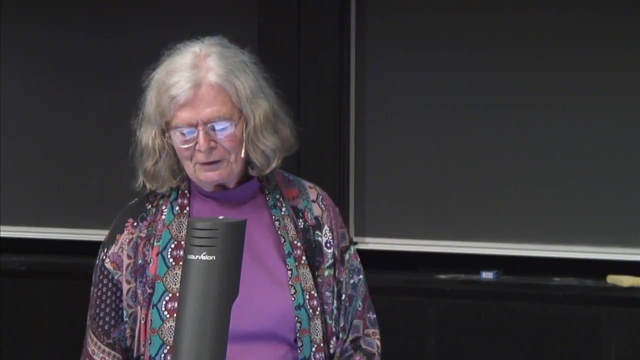 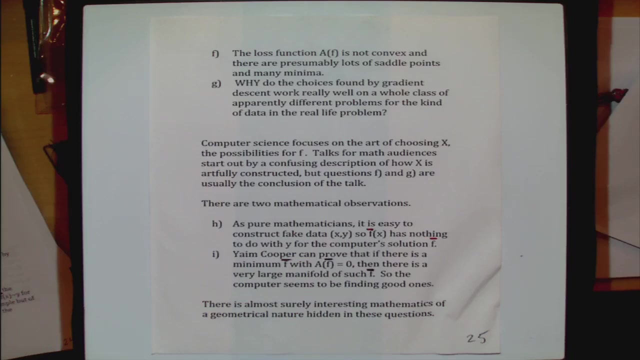 And the question So. So let's We come to the Oh, I really OK. Now there are two things: The loss function is not convex and there are presumably lots of saddle points, And in fact they know this.